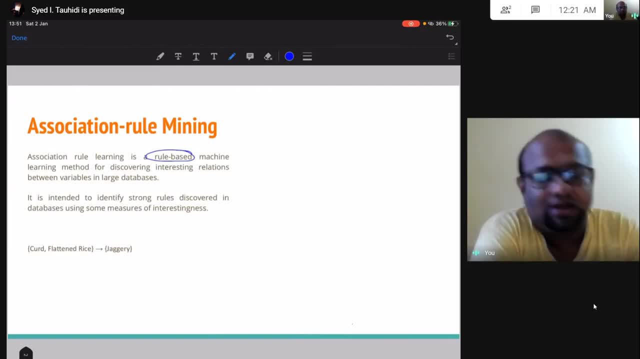 be significant. Now, what do we mean by significant? It will be significant using some measure of interestingness, So we are going to find rules which are interesting in some way. Alright, Now, what is a rule? That would be the most obvious question. A rule is an implication. 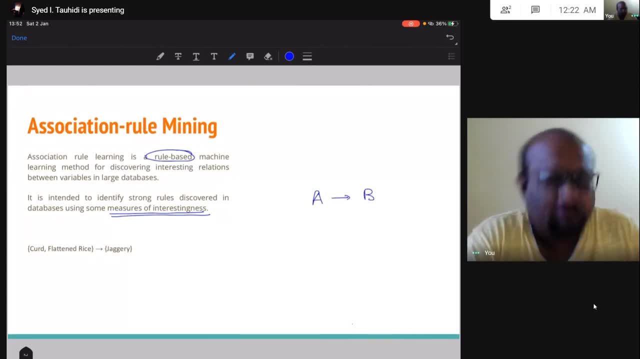 of the form A, It implies B- Alright, These kind of implications are called rules. Now, both A and B over here are sets, Alright, Sets of different things. For example, A can be a set of movies. So if A is a set containing one single movie- Harry Potter and Philosopher's Stone- Okay. 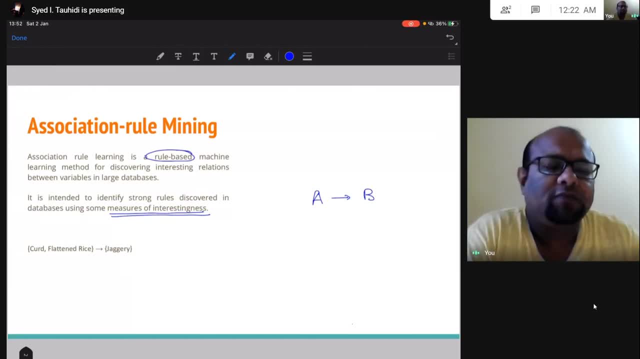 And B can be a set containing other movies, Like, say, three the other six Harry Potter movies or seven Harry Potter movies. There are eight Harry Potter movies. So what would that mean? What would this mean? Harry Potter and Prisoner and Philosopher's Stone implies say Harry Potter and say Chamber of Secrets. 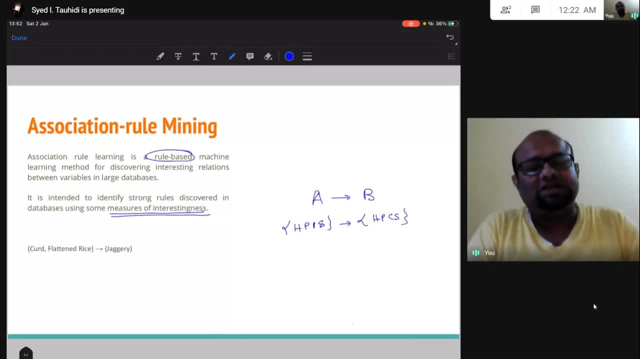 Alright, Let's keep it simple right now. This kind of rule would mean this: that if a person watches Harry Potter and the Prisoner and Philosopher's Stone, then they can see that the person is going to watch Harry Potter and the Chamber of Secrets. Alright, We will. 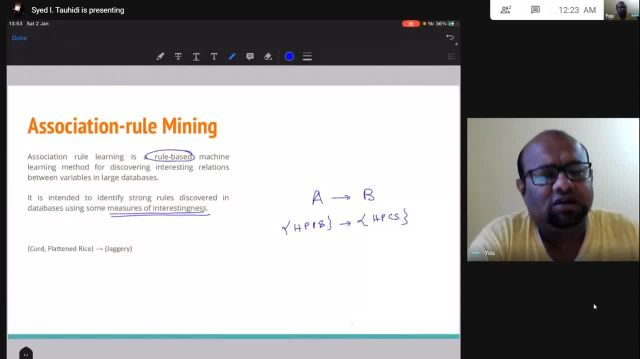 have to generate rules like this from dataset. If our dataset contains information of what kind of movies people watch, then maybe we will go ahead and generate this kind of a rule. Alright Now, another rule might be Harry Potter and the Prisoner and the Chamber. 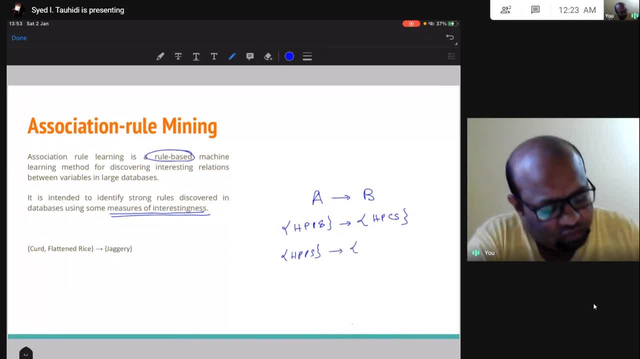 of Secrets. So if a person watches Harry Potter and the Philosopher's Stone, alright. and then I am going to recommend Harry Potter and the Chamber of Secrets, Harry Potter and Prisoner of Azkaban and so on, Alright. So if a person watches Harry Potter and the Philosopher's 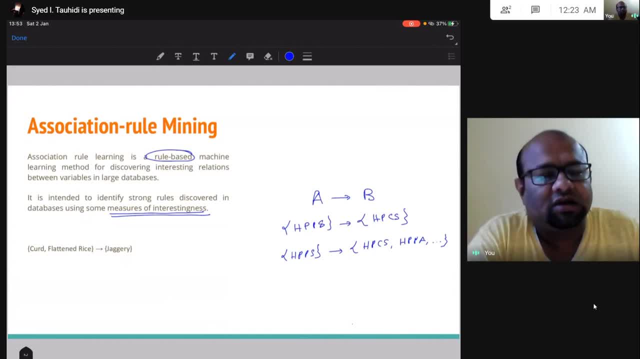 Stone, I am going to recommend, okay, Chamber of Secrets, Prisoner of Azkaban and all these other movies. So this would be what this second rule might mean. Alright, And then we may have this kind of rule. Well, I have this kind of rule. I have this kind of rule. 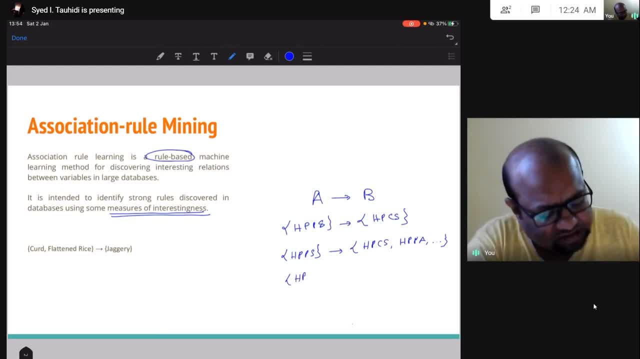 I have this two movies on the left. So the person has watched Harry Potter and the Philosopher's Stone. The person has watched Harry Potter and the Chamber of Secrets, So I am going to recommend the next movie to that person, And that is Harry Potter and the Prisoner. 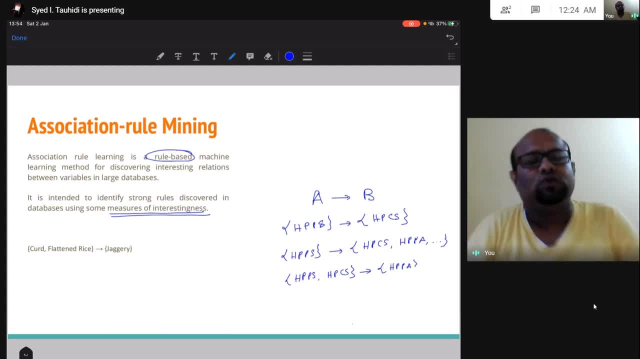 of Azkaban. Alright, In this way we have rules, Alright. So what is the takeaway from here? The takeaway is this: A rule is an implication of the form. A implies B When B are both set. Now, what is this set composed of? What is there in this set A and B? We will 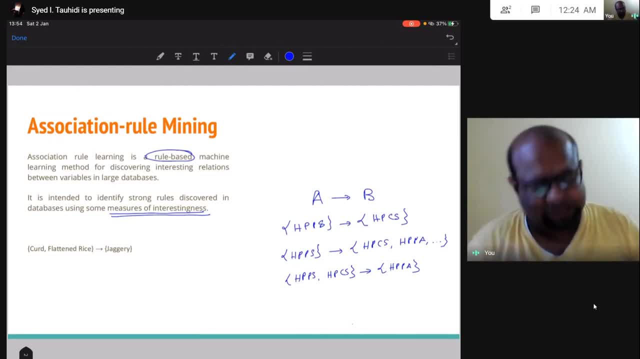 talk about that soon. Another example of rule that is there on your screen is this: Okay, Maybe we have a shop, There is a shop And in this shop, if a person buys curd and flattened rice, then we are going to recommend jaggery to that person, Right? 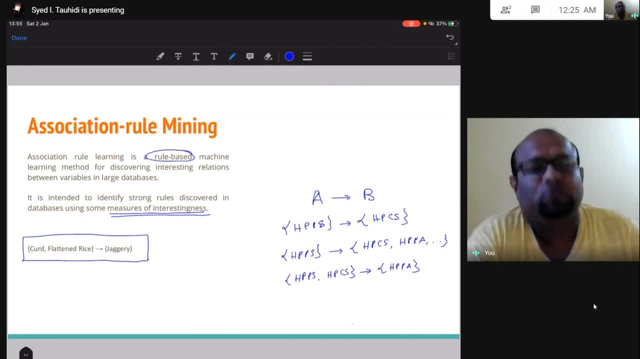 If a person buys doi and sira, we are going to recommend goo to that person. Probably the person after buying doi and sira that person wants to have zompan. Alright, So we will recommend jaggery. So this kind of rule, this kind of implications, are called. 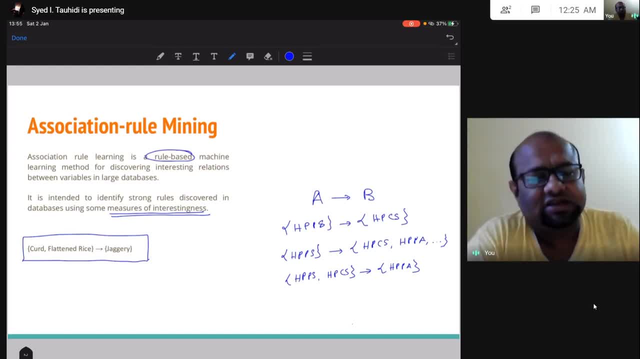 rules. Now we will have data set And from our data set we have to create rules like this: Alright, Rules that make sense together. Now, if I have a rule like this, then I have this Say: in my shop a person comes to buy a mobile- Okay, And I end up recommending: 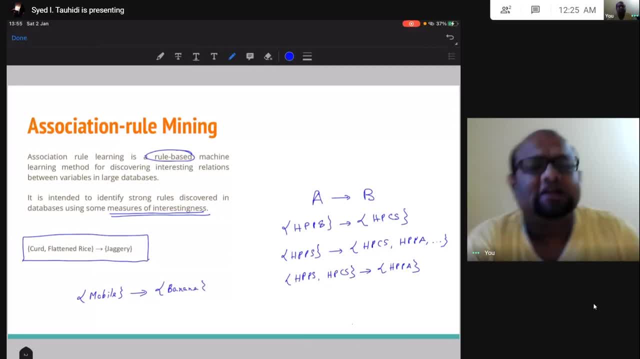 banana to that person. This is- I don't think this is a rule that makes sense. Okay, So if a person comes to buy a mobile, if I recommend a mobile cover to that person or I recommend a mobile headphone to that person, that would make sense Okay. But if the person comes, 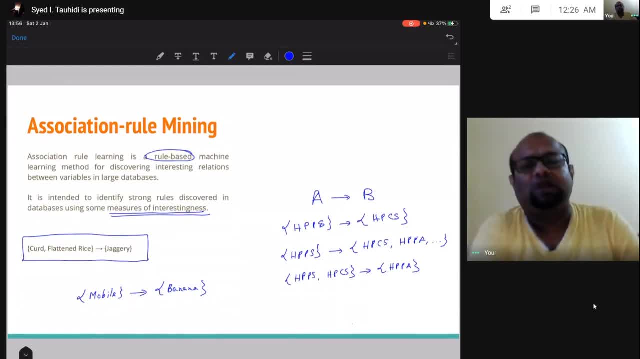 to buy a mobile and I recommend a banana to that person, then I recommend a mobile headphone to that person. That would be bananas. That would not make sense. So how do we get this? sense Means for me. I am a human, So based on my experience I can say that mobile implies 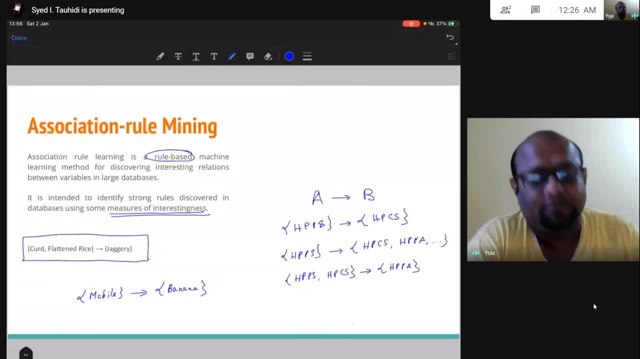 banana does not make sense. But for a computer, how will a computer make sense out of all these things that people are buying? Alright, For that we need some measure of interestingness, Alright, And this is what we are going to talk about soon. Let me give you two more. 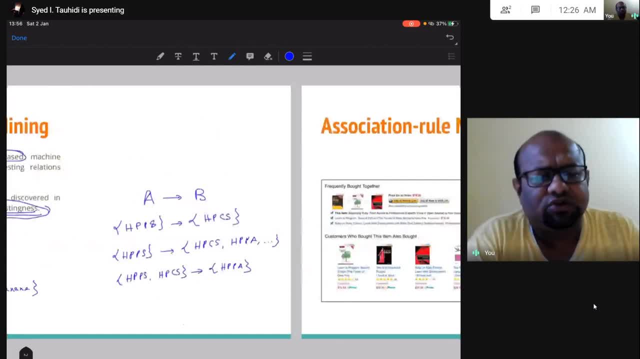 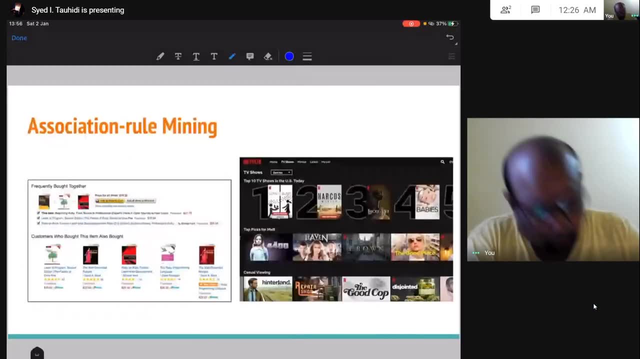 examples of association rule mining that are very popular, very frequently used in our day-to-day life. One of them is- you see this very often when you go to Amazon. These things are frequently bought together. So if you buy, go to a page, then you would be recommended. 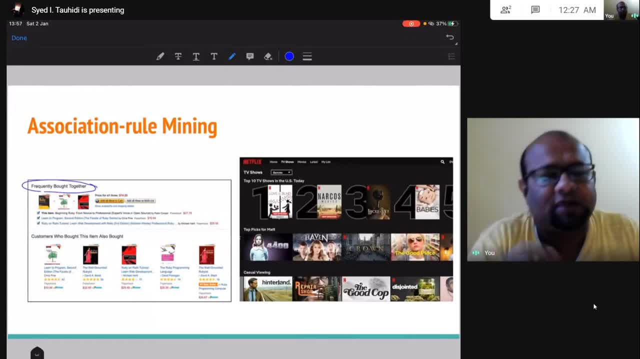 to buy a mobile. So if you buy a mobile, you would be recommended to buy a mobile. So if you buy a mobile, you would be recommended that if you buy a, go to a page of a particular mobile phone, you would be shown cover of that mobile phone. Alright, Or customer who? 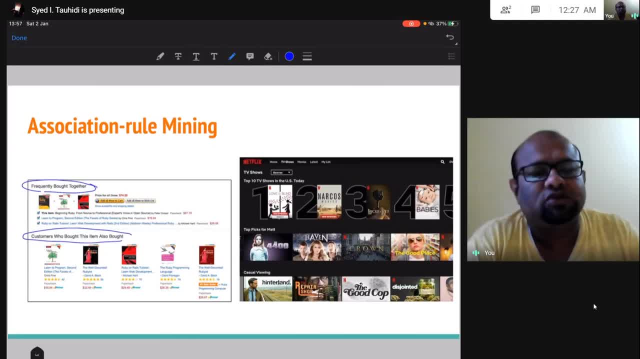 bought this also bought this. Alright, So if you go to a page to buy Arduino, maybe they will show you motors and LEDs, relays and all those kind of stuff. Alright, So yeah, Recommendation engine Mm-hmm. 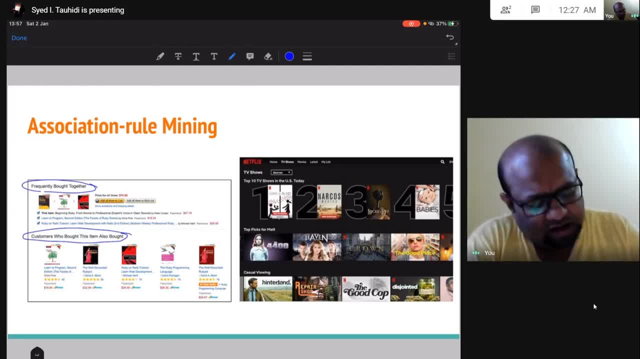 We called it the browse engine, So note that this is first version here. Okay, The one thing that I will repeat and then some comments to make sure that the other side is clear. Okay, So, based on what you like to watch, they are going to recommend only those kind of videos. 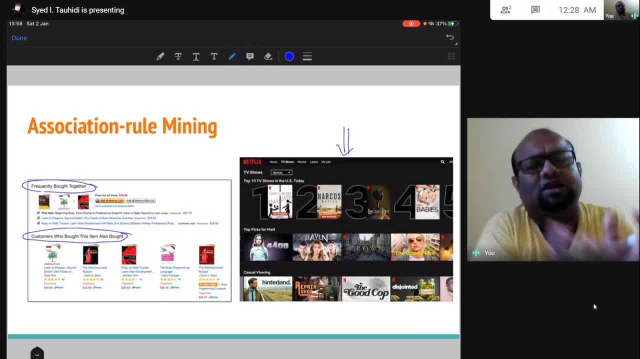 Alright, This is what association rule mining or a recommendation system, is going to do. Now, I am not going to make it a political statement, but this is something to think about, right? So YouTube will do what YouTube, Facebook, all the social media they like- to show you things that you like to watch. 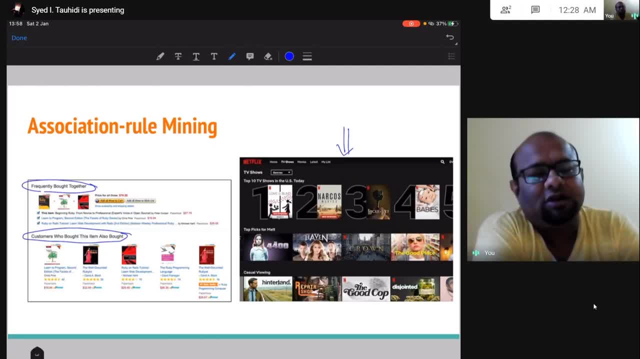 And in doing this, they push you into a bubble where you only watch videos that agrees with your viewpoint. So you live in a bubble. You don't really get an idea of what is happening in the real world, Alright, So that is one negative point about these things. 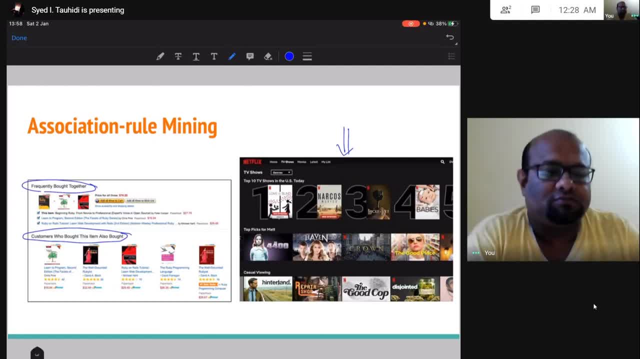 But that is not a thing that we are going to talk about And this course, alright. that is beyond the scope, So let us not spend any more time talking about this. I just wanted to show you two examples where two popular places, Netflix and Amazon- where recommendation system using this rule-based association, rule-based data analysis- alright is used. 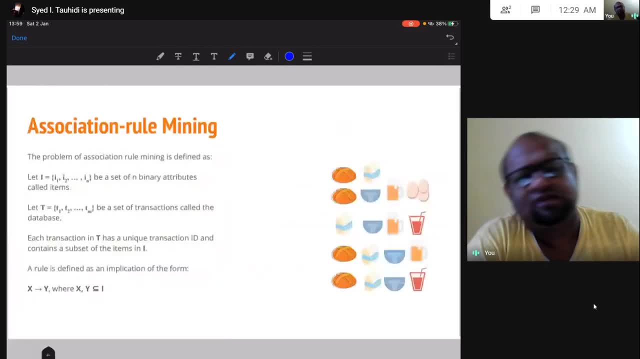 Alright, Now let us look at that. So let us look at the formal definition of association: rule-based Alright. And in doing that, we will be looking at the data set that you see on the right. So this is a data set. 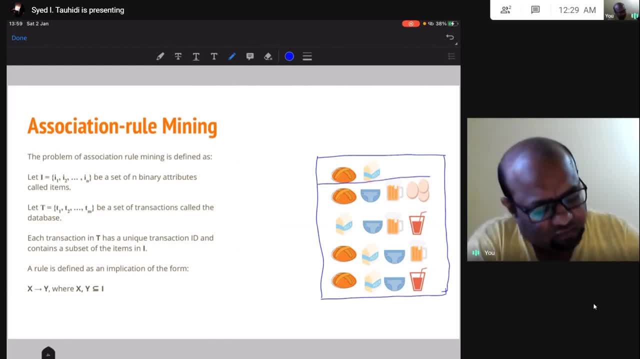 Alright, This data set contains five rows, Alright. So this five rows corresponds to five transactions that happened in a shock. Okay, So a person came into the shock person number one. That person bought something. Alright, What did the person buy? 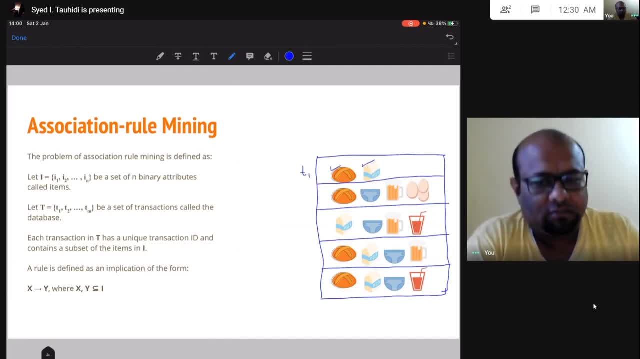 The person bought a bread and a milk. Okay, So that was your transaction one. Then another person comes in. That person buys bread, diaper, beer and egg, So that was transaction two. Then another person comes in, buys milk, diaper, beer and juice. 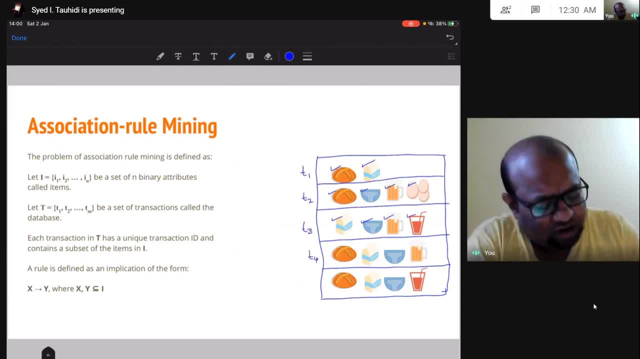 So that was transaction three. Similarly, we have transaction four and transaction five. So there were five transactions that took place in the shock, Alright. And then there were, each transaction, the people bought certain number of things, Alright. So we are going to look at three things over here, three sets over here. 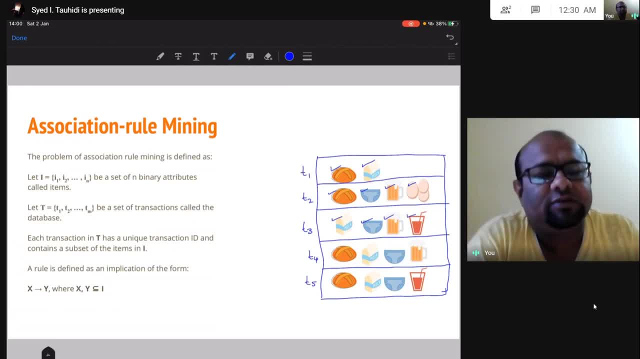 Alright. The first set is the set of all items that are available in the shop. So in our case, we have bread, Alright. We have milk, We have diaper Eggs And we have juice- Alright. So there are five things that somebody is going to buy from the shop. 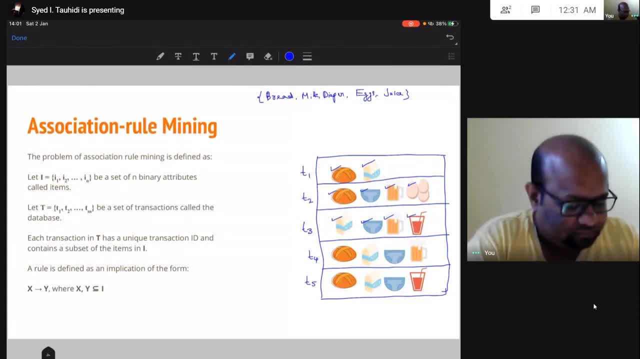 Alright, Now this set is called the set of items. Alright, So I we are going to denote this set using this capital letter. I Let I containing these attributes I1 to IN, be a set of N binary attributes called items. 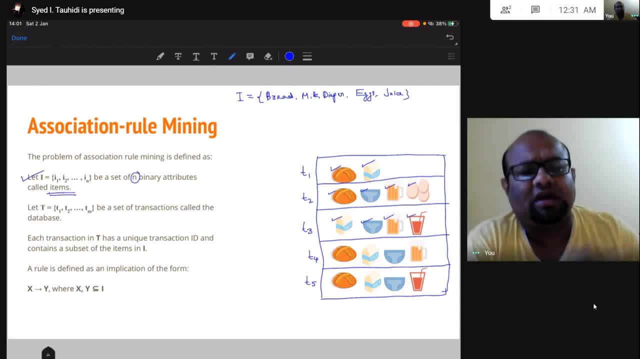 Alright. So there are these items that are available on your shop And the set of all the items that are available in your shop is the set I. Alright, Then the set T be the let T be the set of transactions that are there in your database. 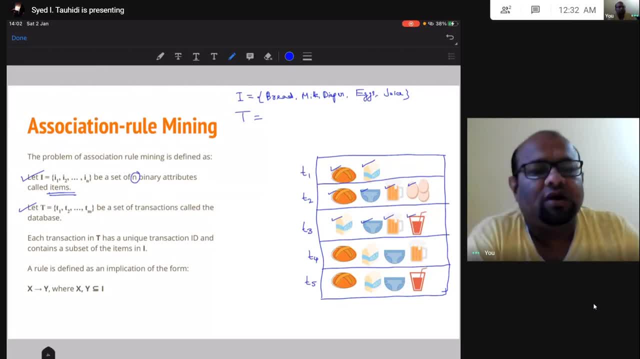 Alright, So in our case we have five transactions, T1 up to T5.. Alright, So transaction one was this transaction that contained bread and milk. Okay, In transaction one, the person bought bread and milk. In transaction five, the person bought bread, milk, diaper and juice. 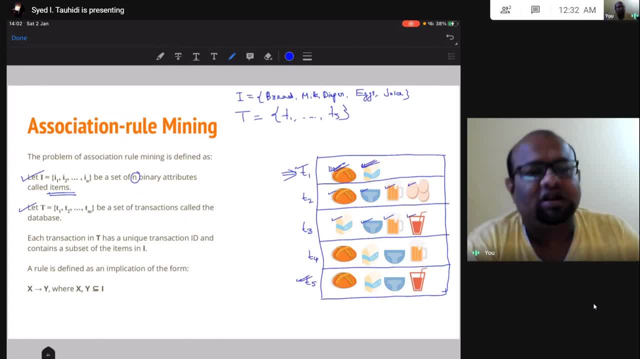 Alright. In this way, we have five different transactions Alright And this set of all transactions that took place in our case. this five, This set is denoted by this capital letter T And this is our entire database, Alright. 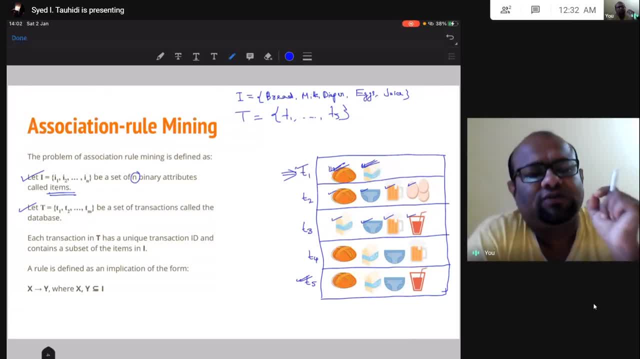 Now let us talk about what is each of these elements inside this set T? All right, This T contains all the transaction. What is the transaction Now? each transaction in T has a unique ID, All right, And we have done that. We have called this transaction T1.. We call this T2, T3 up to T5. So every transaction has a unique ID. That's fine. 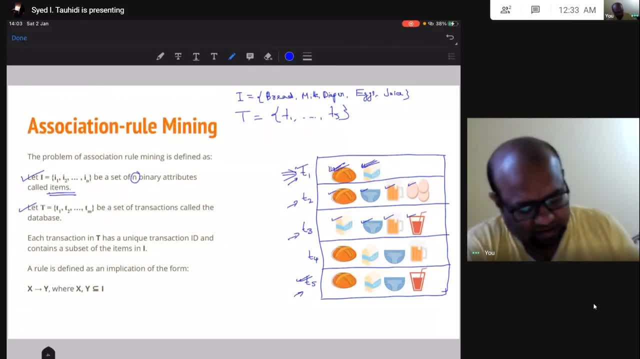 And what is the transaction? It contains a subset of the item in I. All right, A transaction will contain a subset of the item in I. So what is I? I is the set of all the items that are available in my shop. 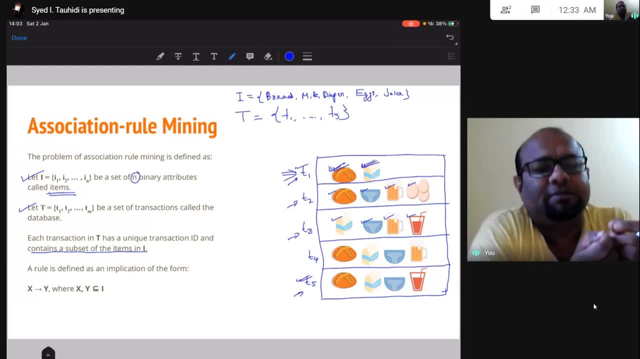 What is the transaction? The things that people are buying. All right, So a person can buy only things that are available in my shop. So a person will buy things. All right, A couple of things. For example, in transaction T1, the person is buying bread and milk, This set set containing bread and milk. This T1 is a set containing element item bread and milk. So T1 is a subset of the set of all items. Right? So yeah, that is what we have. So each T I is a subset of T. All right, Now what is a rule? 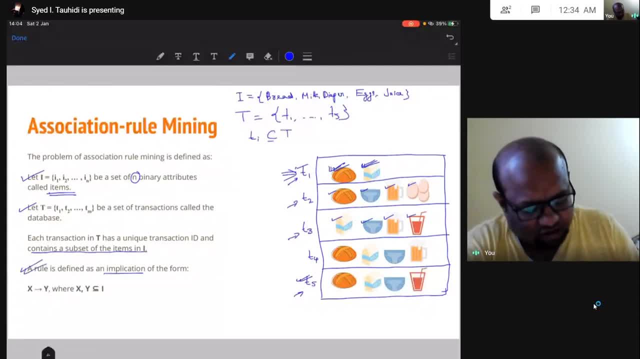 A rule. A rule is defined as an implication of the form. X implies Y, All right, Already talked about that. X implies Y. This should be a rule. Okay, It's an implication of this form. What are X and Y? X and Y are subsets of I, All right. For example, a rule may be: if a person buys diaper, go ahead and recommend beer to that person. 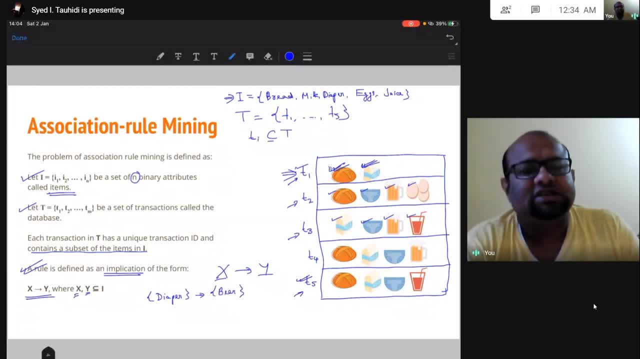 All right, So this is a rule Here. the set X is this set, the set containing the element the item diaper, And the set Y, the set on the right, is the set that contains the item beer. All right, So both X and Y, both the set containing diaper and the set containing beer, are subsets of the set of all items. 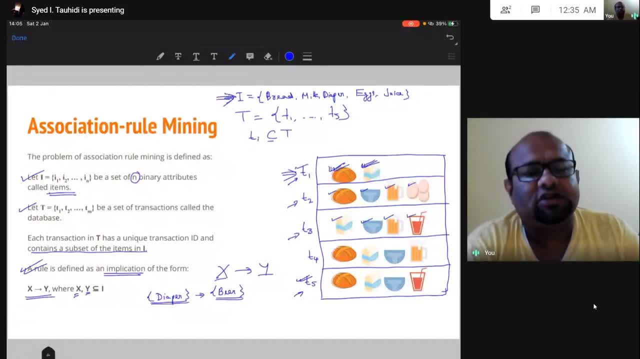 There are lots of items And X and Y are subset of that set of all items. All right, So this is a rule. This kind of statement are rule. Now I may have another thing I may have. if a person buys bread and milk, then I'm going to suggest what Egg to that person. All right, This may be another rule. 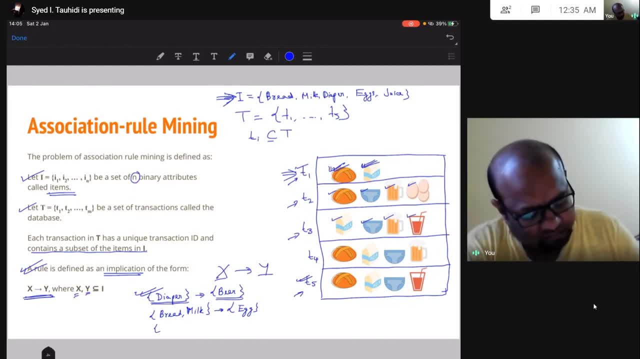 I may have yet another rule where, if a person buys juice, go ahead and suggest milk and bread to that person. This might be yet another set. All right, Yet another rule. Anyway, a rule will contain a set on the left and a set on the right. 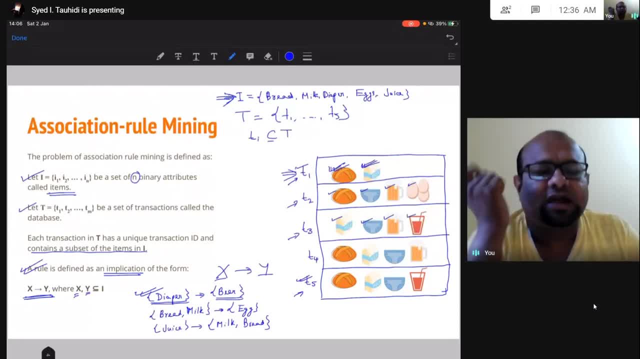 All right, Both these set that are there on the left are subsets of the set. All right. So this is a rule, Both these set that are there on the left and right. we are indicating that by X and Y respectively, both of them will be subsets of I. All right. So, yeah, This kind of rule, this kind of implications, are called rule All right. And what is our task in association rule mining? Our task is to generate this kind of rule, All right. 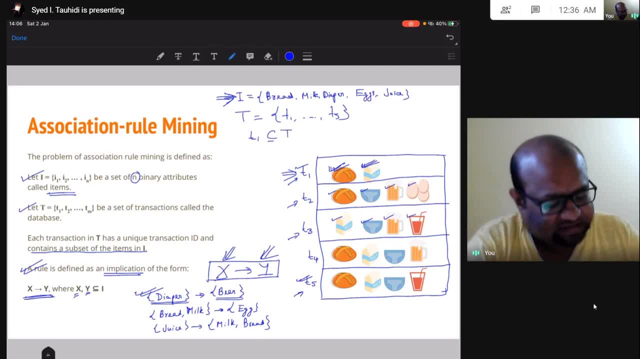 All right, This data set, This is our entire data set And by doing running some algorithm on this data set, we have to generate this kind of rules, Right. What does this data set contain? The data set contains transaction. The data set. 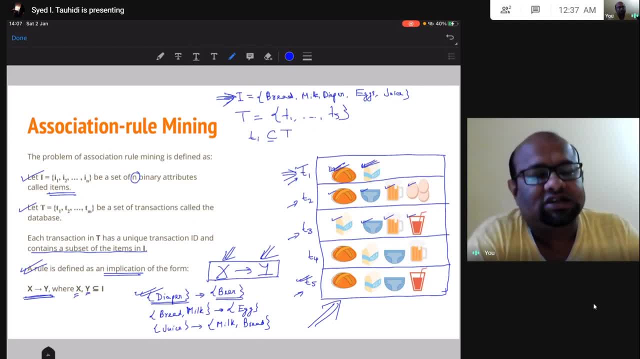 is a set of transaction. What is a transaction? A transaction contains all the items that are bought together by a person. So a transaction will contain: the transaction is a subset of the set of items that are available in the shop. all right, so this is what it is. this is the basic idea behind association rule mining. now we are going to 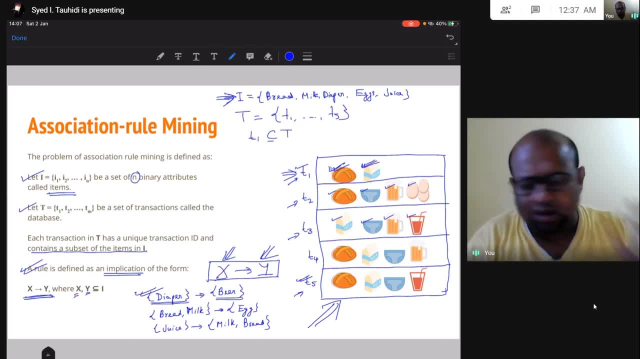 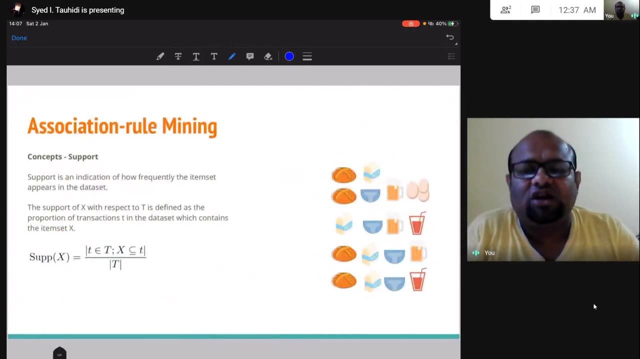 talk about two concepts before we go ahead and talk about what are the algorithms that are available and all these kind of things. the first concept that we are going to talk about is support. all right, so what is a support? a support is an indication of how frequent the item set appears. 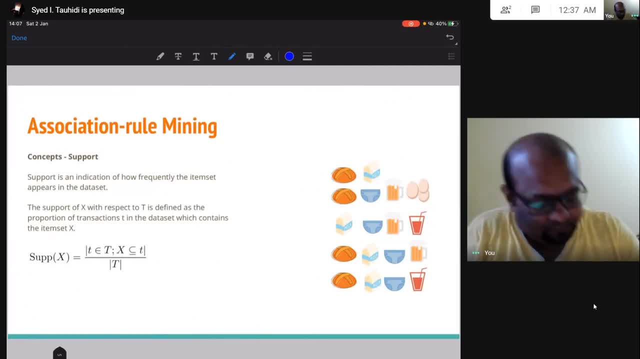 in a data set. so yeah, that is what it is. how many times do something appear in a data set? the support of x with respect to t, so x is a set, a set of items, all right. the support of x with respect to t is the support of x with respect to t, so x is a set of items, all right. 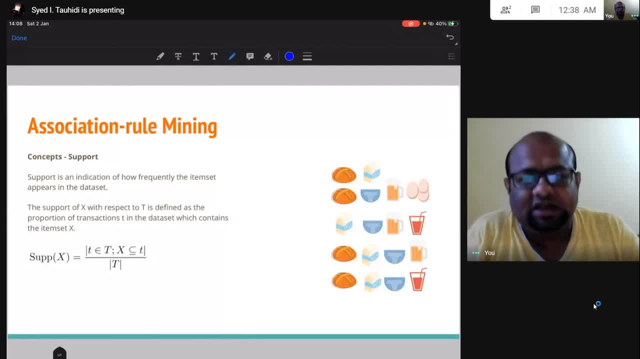 defined as the proportion of transaction t in the data set which contain the item x. all right, this may sound like lots of words, but this is a very simple idea. okay, let me give you an example. say: x is this set containing diaper? all right, x is the set containing diaper. let's work with. 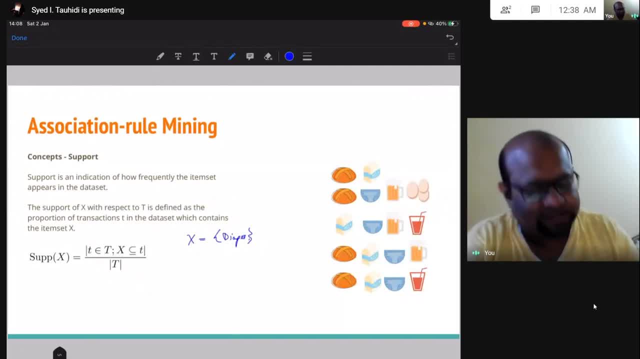 a set containing only one thing first. then we will look at set containing two things. all right, so x is the set containing diaper, all right, what is the support of x? what does this say for each transaction? i will see if x is a subset of the transaction. all right, i will find how many. 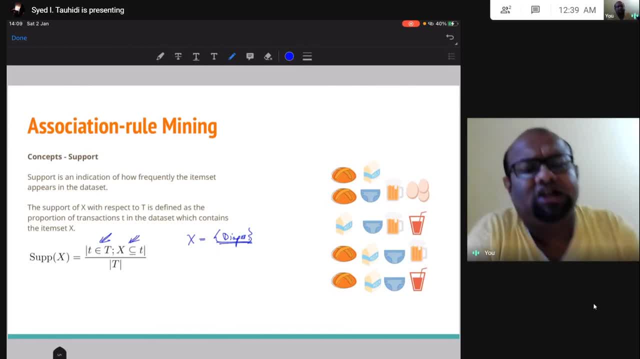 transactions are there and i will get the cardinality of them. let's see this, this, this and this. there are four transaction out of four, total five transaction that contain diapers. all right, so, uh, this, my numerator is going to be four. how? what is in my denominator denominator is the cardinal entity of set t. what is set t? 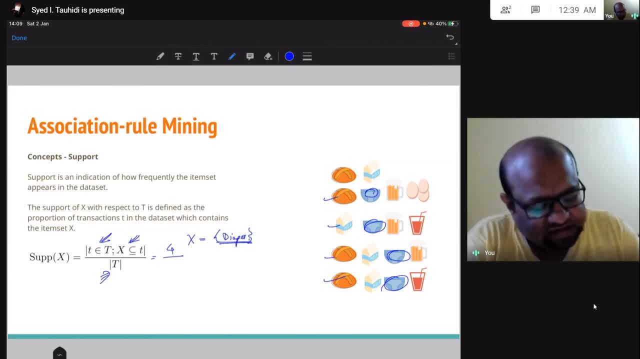 is the set of all transaction. so how many transactions are there in total? there are five transactions in total, all right, therefore, the cardinality of set t is equal to five. all right, therefore. uh, the support of x, where x is the set containing only diaper, is equal to. 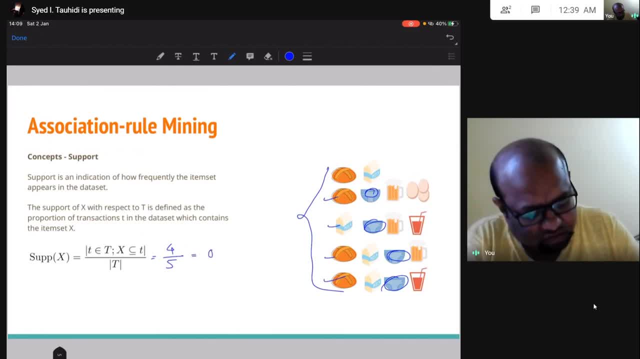 4 by 5 and that is equal to 0.8. all right, so this is support, very simple idea. let us look at another example. let me uh: diaper and beer, all right. so what is the support of x? now? uh, for each transaction. if the transaction contains diaper and beer, we are going to count that, all right. 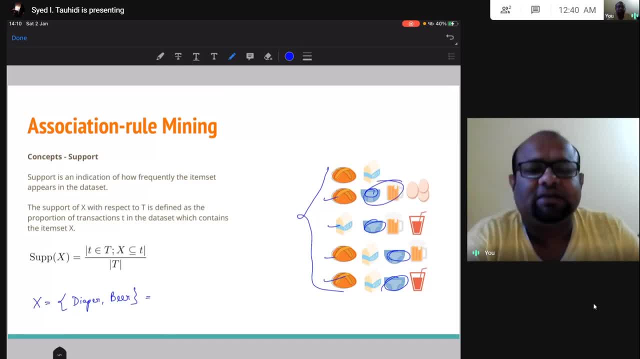 so this transaction contains diaper and beer. these transactions contain diaper and beer. this transaction contain diaper and beer. so there are three transactions that contains diaper and beer. all right, therefore, our numerator is going to be three. denominator, like before, is going to be five, because there are five transactions in total. 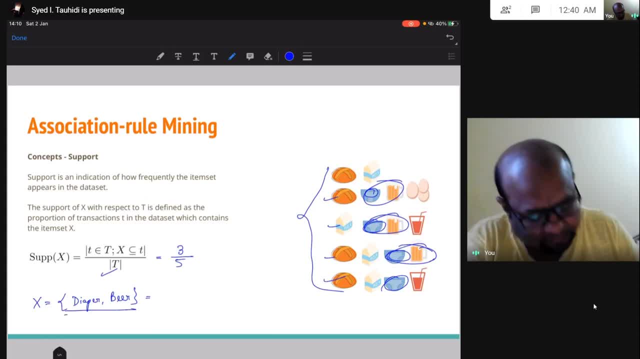 and therefore the support of this set containing diaper and beer is equal to 0.6. all right, so this is support, all right. what is support of some set? uh, uh, the number of times that the set appears in my transaction. it's very simple idea. okay, how many times does the set uh appear in my transaction? 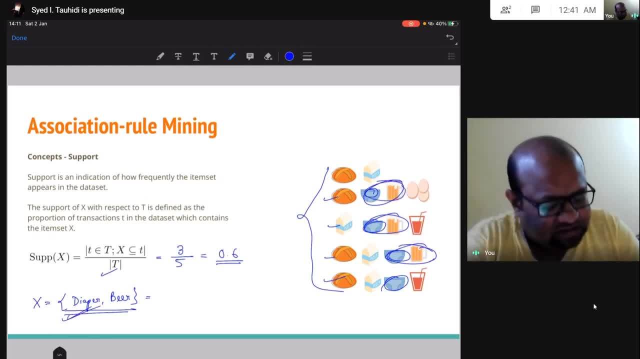 so this is the same diaper and beer. it appears three times here, here and here. so three divided by how many transactions are there in total? there are five transactions in total. therefore, three by five is equal to 0.6. all right, simple idea. this is called support, the next uh concept. 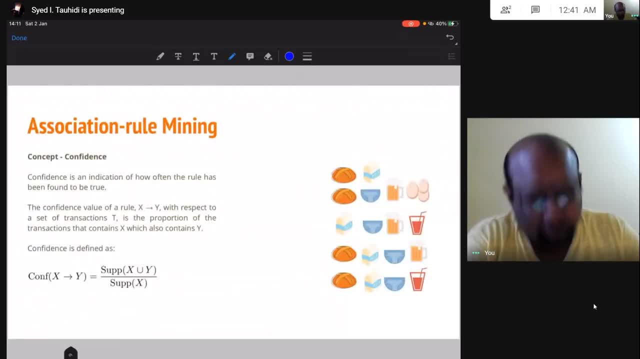 are going to talk about is this concept of confidence. a confidence is an indication of how often the rule has been found to be true. okay, so we have some rule. we created this rule, right, diaper. so if someone buys diaper, go ahead and recommend beer to that person. okay, 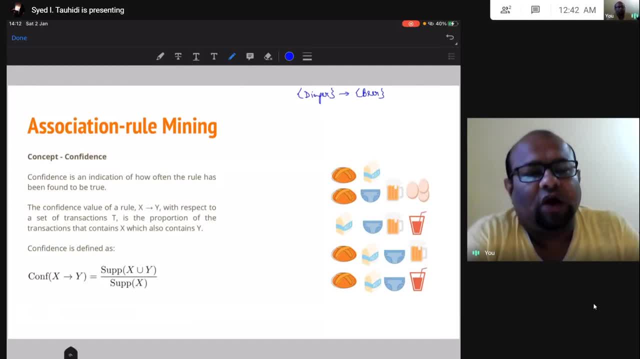 so we had created this rule. now, how confident are we about this rule? okay, so we created this rule, think about it. because we believe that if a person buys diaper, the person is going to buy a beer. okay, now, if we don't believe that, then why are we going to recommend beer to a person who 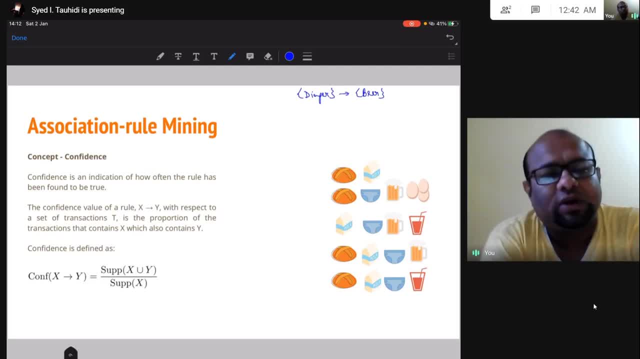 buys diaper. now, uh, i have to do one thing. i have to see how confident am i about this rule that i have made. say, i believe that a person buys, who buys diaper, also buys beer. okay, so diaper and beer are bought together. that is my belief. i have to taste this belief, okay. 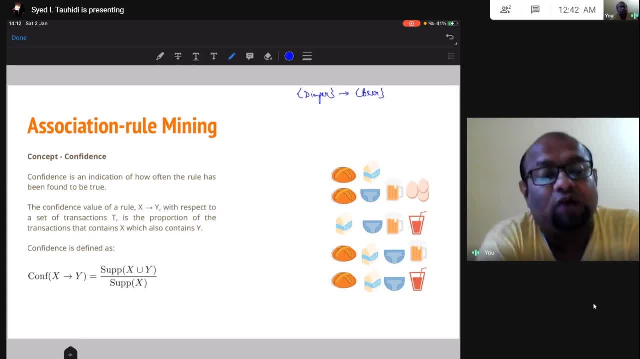 so i'm going to do a very simple thing. i'm going to see how many times is diaper bought. okay, in total, how many transactions are there that has diaper as one of the purchased items? out of all this transaction that contains diaper, in how many of them are diaper and beer bought? 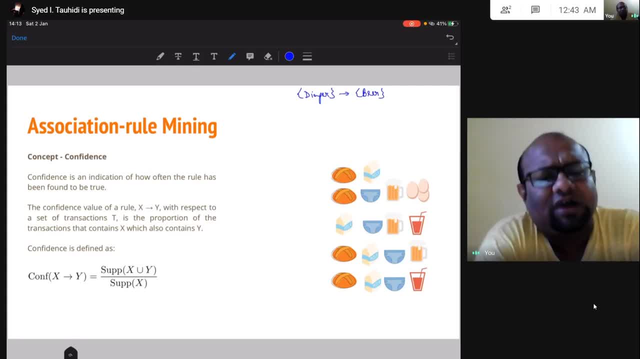 together. okay, so if i have hundred transaction- uh, diaper is bought by 100 different people in 100 different transaction. in 80 of them the person who has bought diaper has also got beer- then my confidence would be out of 100 times. when people has bought diaper 80 times, people have all. 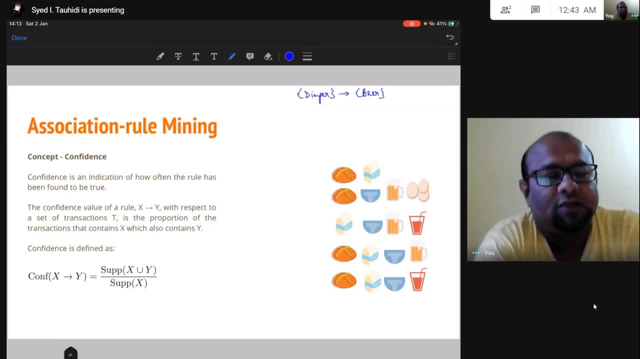 also got beer, so my confidence would be 80 percent. right. this is a very simple idea, and this is called confidence. now, con confidence is an indication of how often the rule has been found to be true. the confidence value of a rule: x implies y with respect to a set of transaction, t. 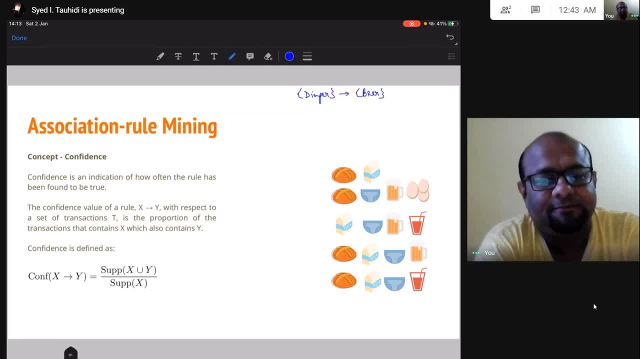 is the proportion of the transaction that contains x which also contain y. so all this transaction that contain x, all right, uh, x equals to non, non-non-non-nononononono. so i'm saying that this is a very simple idea: Out of all these transactions, how many also contain Y? 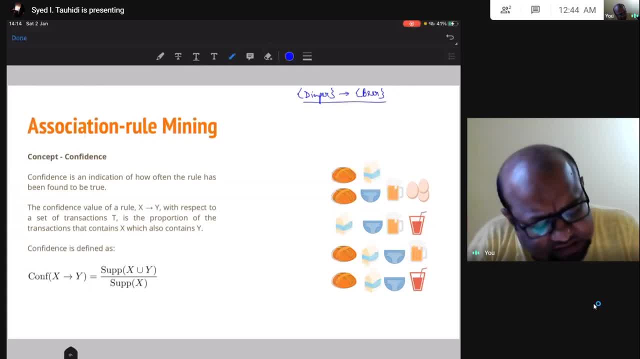 So let us go ahead and figure out what is the confidence of this rule. So to do that first I have to do what I have to find how many transactions are there that contain Y? Let me not do it here, Let me write here itself. 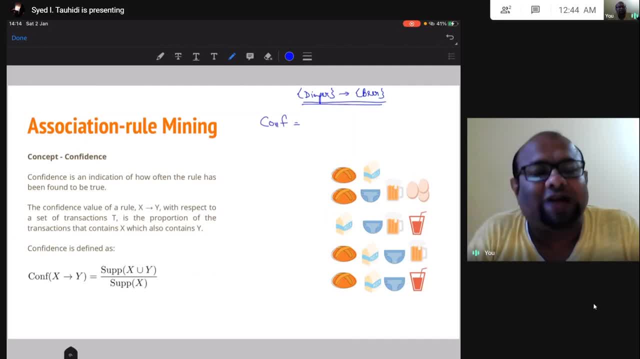 How many transactions are there when diaper are bought. So out of this, find these, these, this and this. There are 4 transactions where diaper is bought, So out of 4.. How many transactions are there when, Among all these transactions where diaper is bought, how many transactions are there? 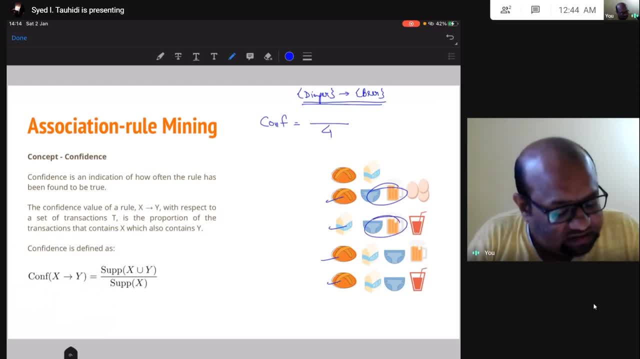 where beer is also bought. So there are this, these and this. All right, So there are 3 out of these 4 transactions where bear is also bound. Therefore, my confidence is 0.75.. Alright, So this is what it is. 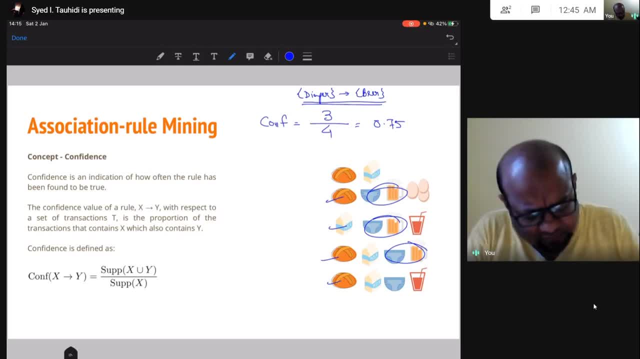 Now, this is the mathematical formula, Just formula using support. But this is essentially the same thing. What is the support of X? Support of X is what is X, X is diaper, Y is bear And support of X is how many transactions contain X. 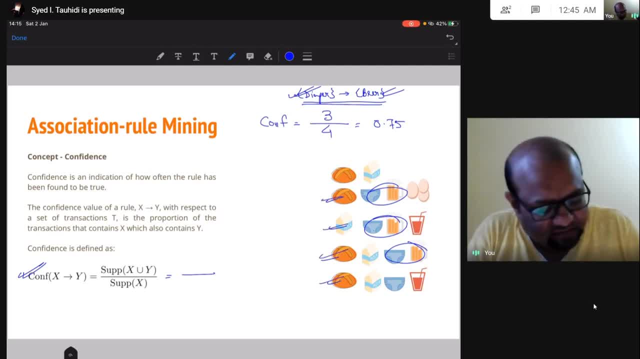 X is diaper. There are 4 transactions that contain X. Divided by total number of transactions, That is 4 by 5.. This is support of X. And what is support of X union Y? X union Y is the set that contains diaper and bear. 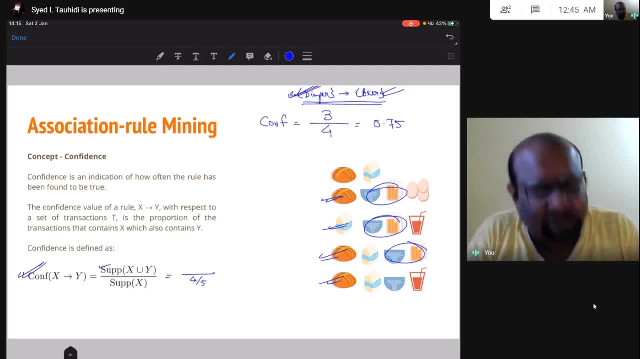 Alright. X is the set containing diaper, Y is the set containing bear. X union. Y is the set containing diaper and bear. So, how many times? What is the support? Support of X union Y. What is the support of this set containing diaper and bear? 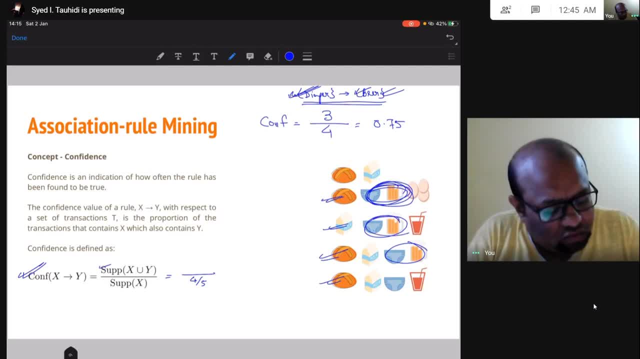 We have to count: There are 1,, 2, 3.. 3 times These 2 are brought together, How many transactions are there? There are 5 total transactions. Therefore, the support of X union Y is 3 by 5.. 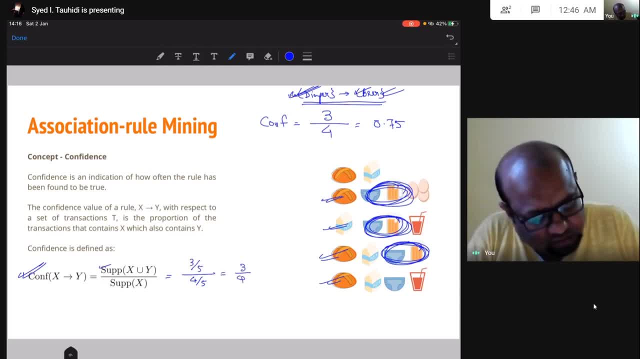 Alright, And this is equal to 3 by 4. And that is equal to 0.75.. Alright, So this is the formula using support: Alright, But then we don't actually need to divide by total number of transactions to find support. 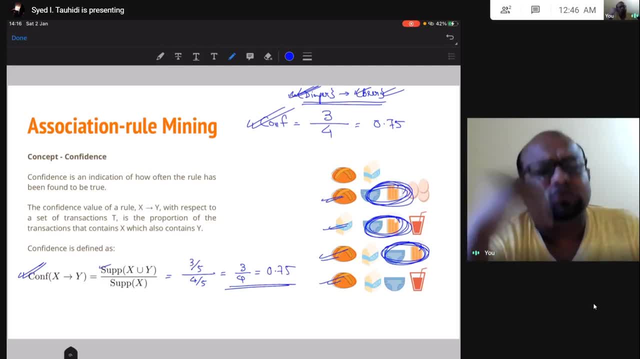 because the total number of transactions is anyway a constant throughout our algorithm. The number of transactions is not going to change. Alright, If we are working with a data set with 1,000 transactions, then throughout my analysis, my data set is going to contain 1,000 transactions. 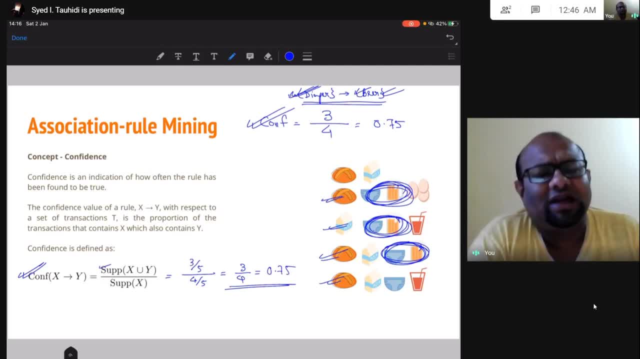 So dividing both numerator and denominator by 1,000, is an unnecessary calculation that I don't need to do. So that is going to cancel out, Right Anyway. So without doing that also, I can go ahead and do this calculation. 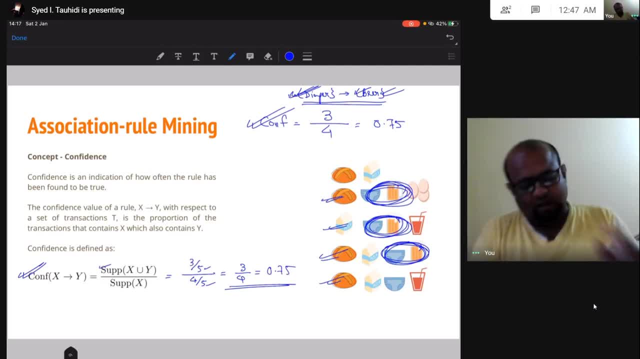 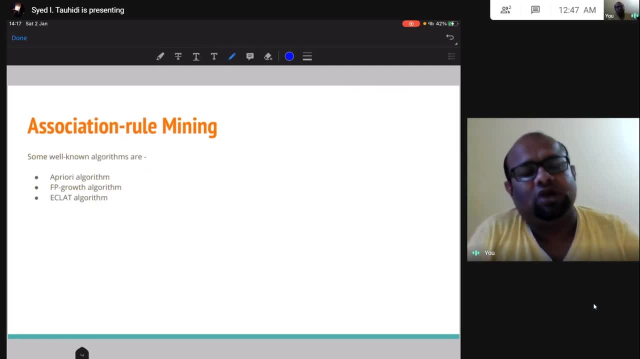 And, yeah, That is what we have. Okay, In this lecture, in this video, we are going to look at 3 different algorithms using which we are going to do association rule mining. Alright, The first algorithm, the first algorithm. 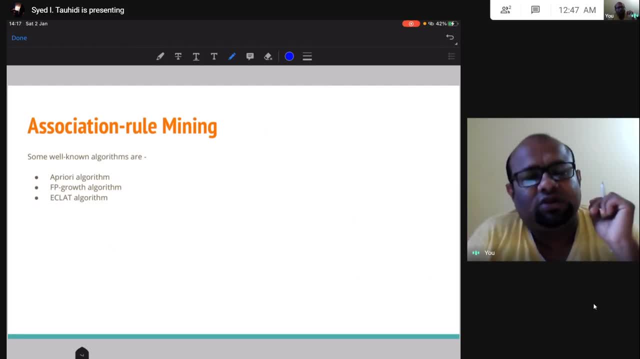 is a priori algorithm. The second algorithm is going to be FP growth algorithm. We are going to talk a little bit about this algorithm. We are not going to look at lots of theory, Don't worry, We are directly going to apply this algorithm on data sets. 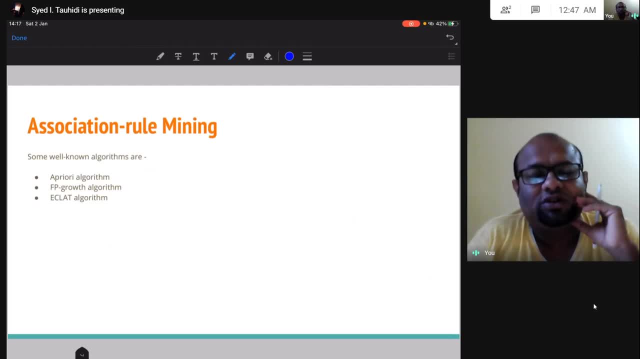 And in doing that we will be learning about how this algorithm works, And then we will be looking at something called FP growth algorithm. So that is my first one, And then I am gonna show you my two algorithms and the ICLED algorithm. 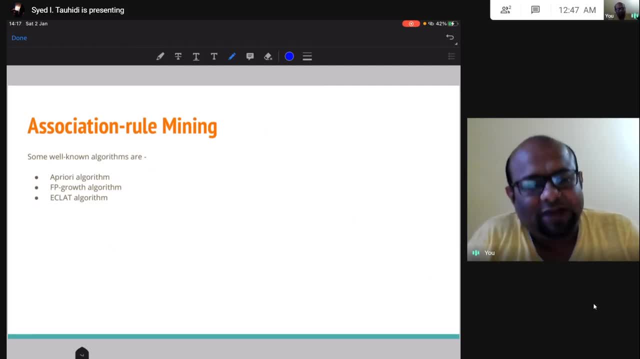 Alright, The ICLED algorithm? I will. Uh, this is also very simple. All these algorithms are simple. FP growth is a bit uh involved. Still simple, Alright. So we will be looking at all these algorithms, But ICLED algorithm. 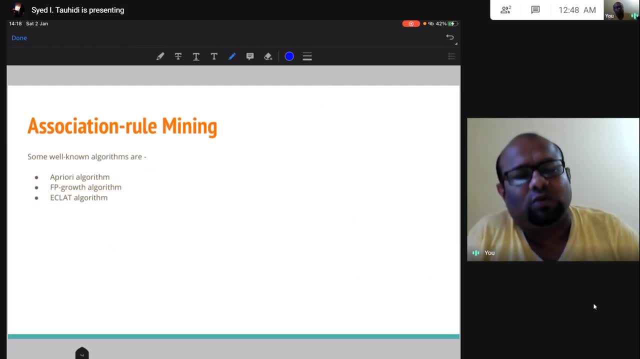 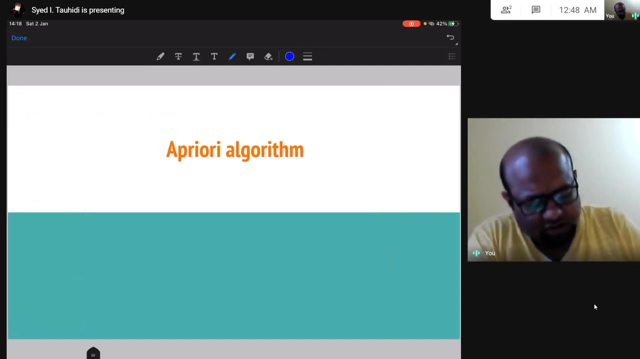 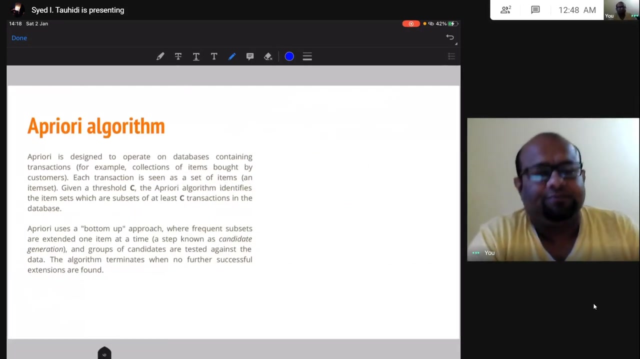 we will not uh, work, uh on a data set. I will just show you a worked example. Right The rest of the uh, the two do this or not? so let us begin talking about a priori algorithm. so a priori algorithm is designed to operate on databases containing transaction, like the. 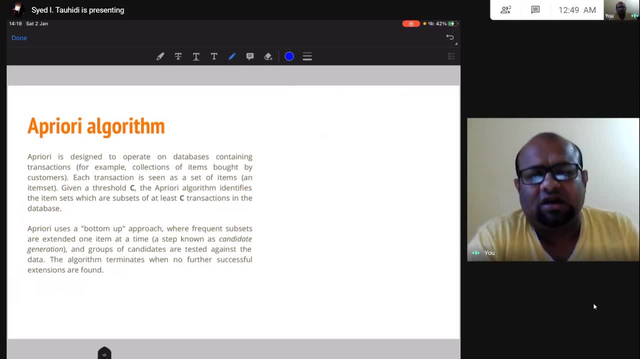 database that we just saw, and each transaction is a collection of item bought by customer. each transaction is seen as a set of items. a set of item is also called item set. all right, now we will be given a threshold. all right, this threshold is called mean support. 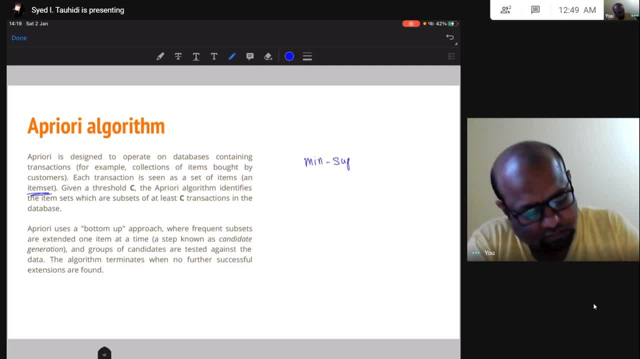 all right, so we will be given a threshold c. this is our mean support. so in a priori algorithm we will work and do this. anything below this threshold we are going to ignore values support greater than this threshold we are going to use in our next round of analysis. all right, what does this? 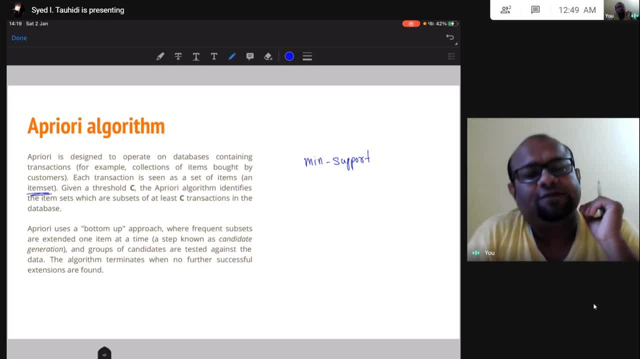 mean. you will see soon when i work on this data set, but imagine this all right now. here is this shop, my shop, in my shop. i want to do analysis. okay, what is the analysis that i want to do? so i want to do a general analysis of the buying pattern of my customers. all right now. 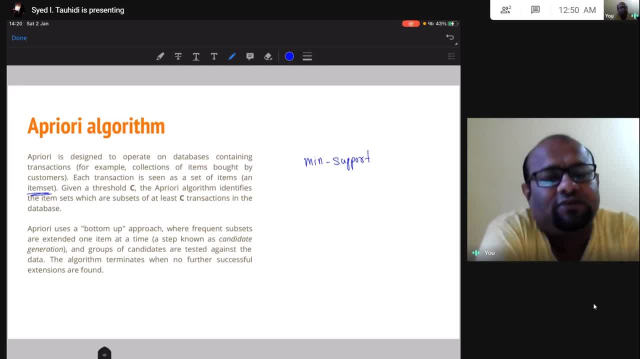 if, say, a item is bought two or three times, only very few times, all right. so i am selling, i am doing thousands of transactions every day and there is this item that is bought only twice or thrice, say a television, a very expensive brand television, smart tv, that is. 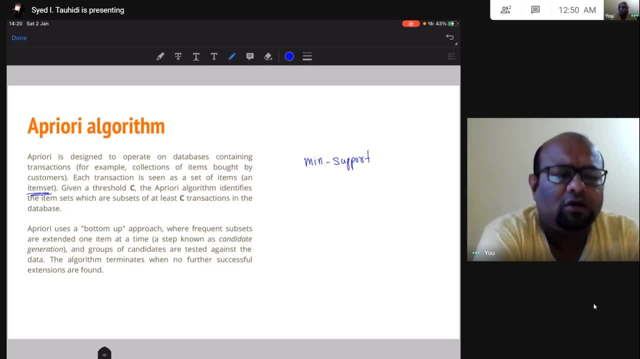 not sold very often all right now. the problem if i try to do analysis with this television is this: i want to know about the general buying pattern of the entire population, of lots of people. all right now, if i use this particular television, that is bought by only one or two. 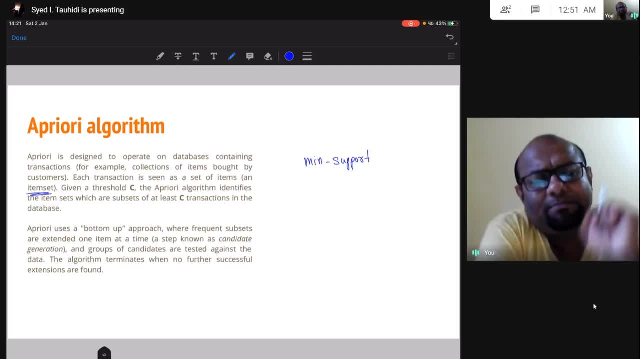 people. what will happen is i will learn about the buying pattern of only those one of two people. all right, therefore, uh, things that are very rarely bought, okay, things that are bought very rarely, uh, i am not going to try finding patterns of those things, all right, so i will be having some. 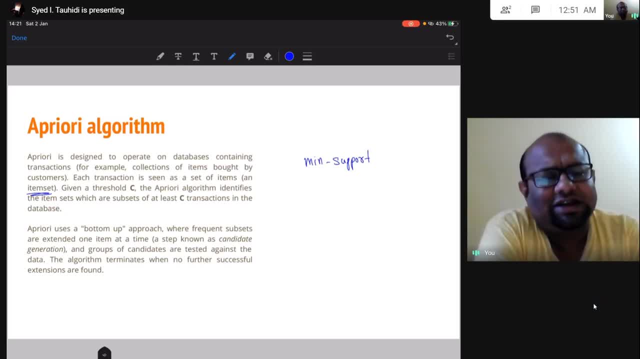 threshold. this means about: so things that are bought less than the mean support. i am not going to use those things for further analysis and that is the basic idea behind this threshold, all right, so only items that are bought together frequently, items that are bought often- okay, not often, but, uh- more than this threshold level. so only those items i am going to. 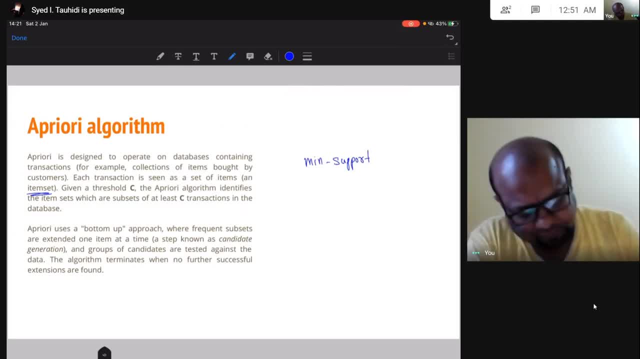 do an analysis on all right. so, given a threshold, a priori algorithm is going to identify item sets which are subset of at least three. this many number of transaction, all right now, a priori is going to have a bottom-up approach, so what i am going to do is in my shop. 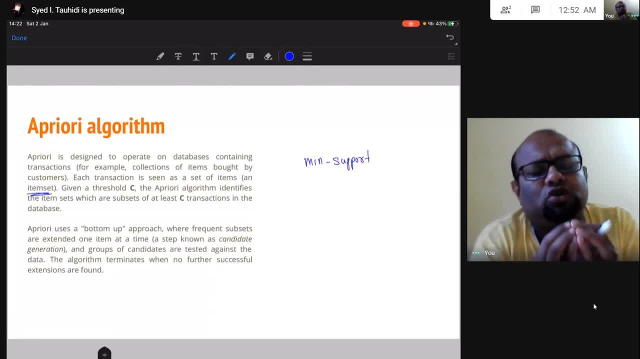 first i will start from the bottom. so what does this mean? i am going to see items one at a time, okay. so first i will see how many mobiles are. so if uh say iphone, okay, so iphone 12, so how many uh iphone 12s are? 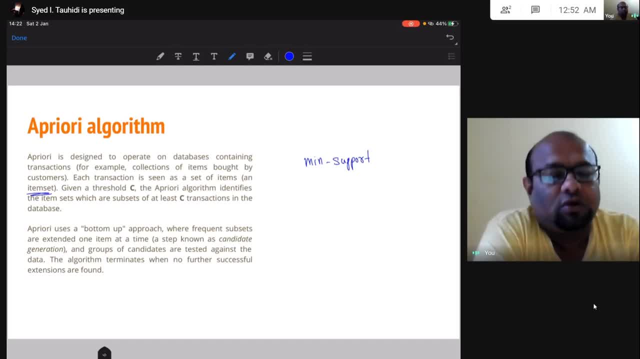 bought. say there are 50 iphone 12s that are being bought. okay, say, my threshold is 25, so i mobile is above this threshold, so i am going to consider mobile for the next round of analysis. okay, and my very expensive smart tv? okay, is bought only once, so my threshold was 25.. so smart tv is 25.. 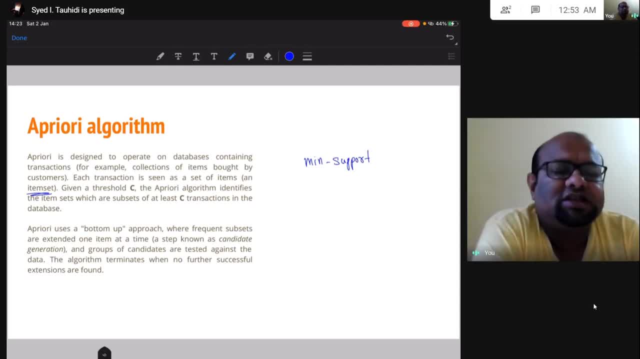 i am not going to consider for the next round of analysis. all right, because it is below my threshold. now i am done and i'm looking at one item at a time. okay, so i looked at mobile. it was bought more than 25 times more than my threshold level, so i'm going to consider it for the next round. 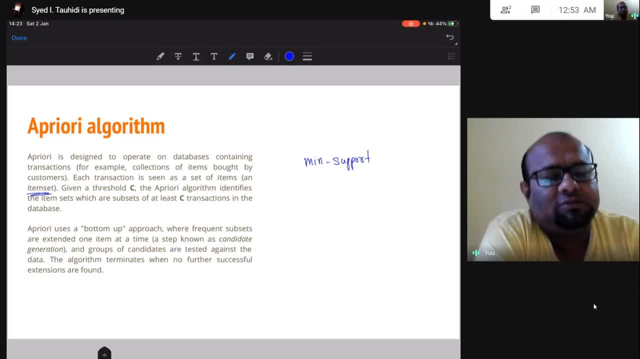 smart tv less than the threshold number of times. uh, purchase less than the threshold number of time. i'm not going to consider it for the next round. all right, so i'm done looking at items one at a time now. i am going to next look at items two at a time. so i see i am going to consider this iphone. 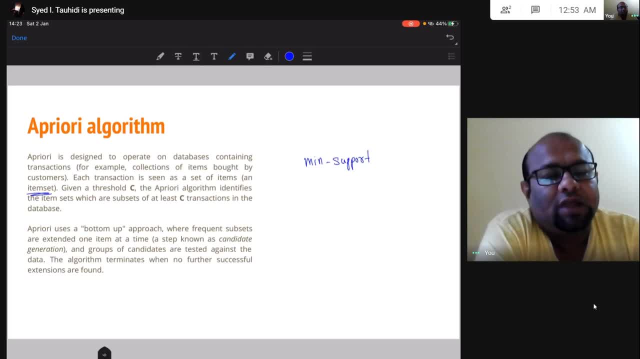 right. so i'm going to see that iphone and uh iphone cover is bought maybe uh 40 times. so iphone was bought 50 times iphone and iphone out of all these 50 times when iphone was bought, i see that iphone and mobiles- they are bought together. 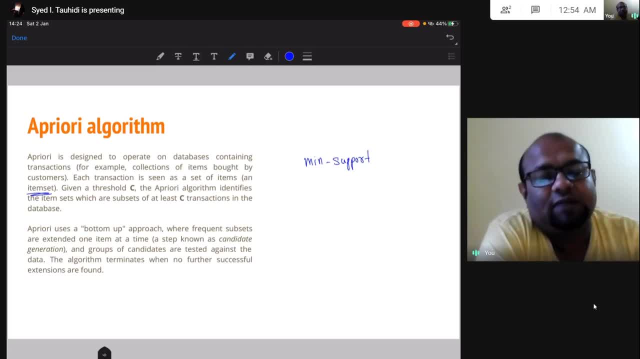 40 times? all right. iphone and cover are bought together 40 times, so this is greater than my threshold. my threshold was 25. so iphone and mobile, i am going to consider, uh, it all right. then i see iphone and banana. this fruit, banana, is bought together only two times or five times. 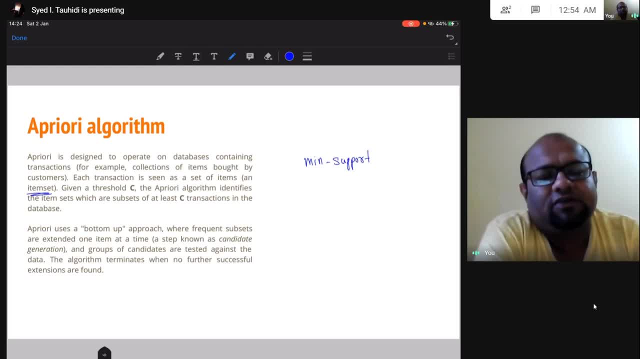 okay, some customer, maybe he was hungry and after buying the iphone he did not have much money left, so he bought a banana. okay, so i see it was bought only two times. so it is below my threshold so i am not going to consider it for the next round. all right, so in this round i am. i looked at items two at a time. item set containing: 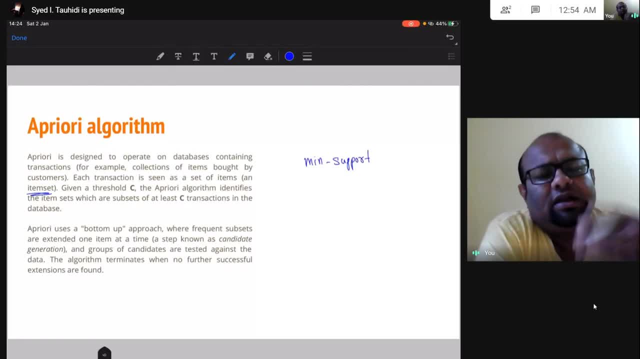 two items. all right, then, uh, in this round, what did i do? i eliminated iphone and banana. i am going to consider iphone and iphone cover. all right, then i am going to go into the next round. in my next round, i am going to take items three at a time. so i am going to say, consider mobile phone. 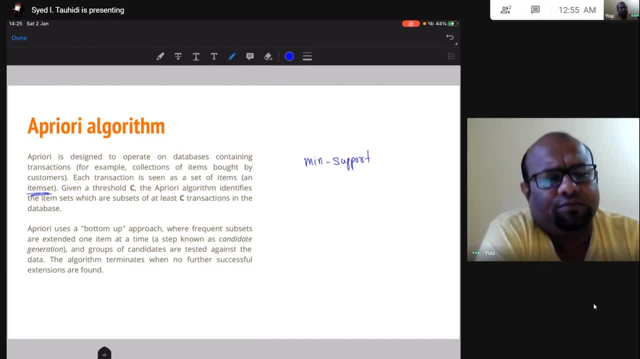 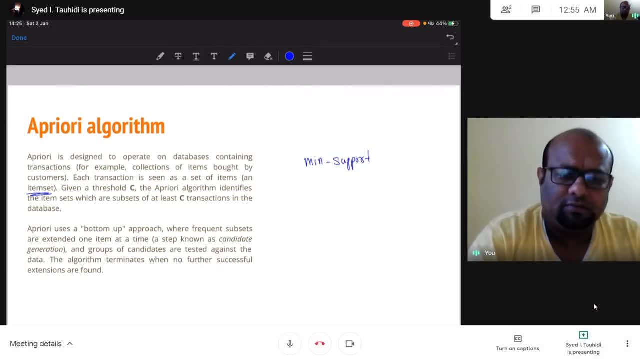 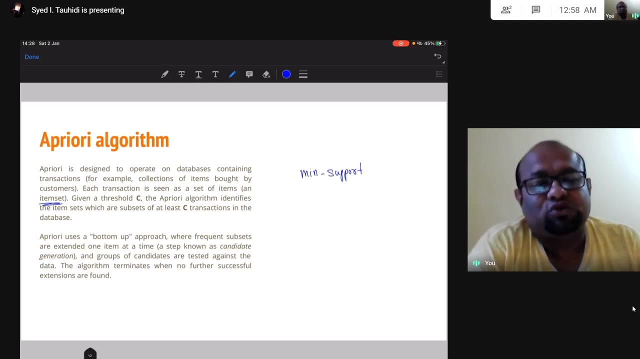 this iphone, then mobile cover and headphone. okay, uh, hold on. okay. uh, my house is by the side of the road and there was some announcement. uh, so sorry for the interrupts and you did not see it. okay, my house is by the side of the road and there was some announcement. uh, so sorry for the interrupts and you did not see it. 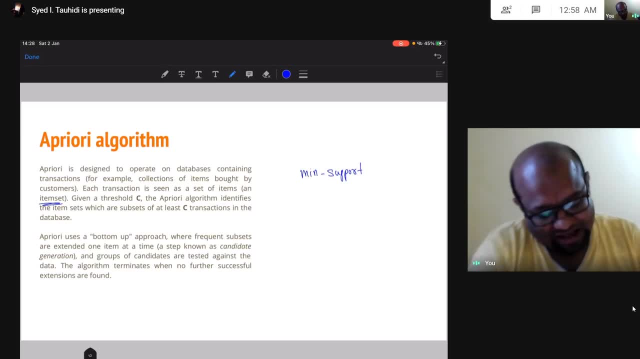 an interruption because i've also done recording anyway. uh, yeah, i was talking about working with uh two sets. right, we ignored this set: uh containing iphone and banana. we are moving ahead with this set containing item set containing uh iphone and uh iphone cover. now we are going to look at. 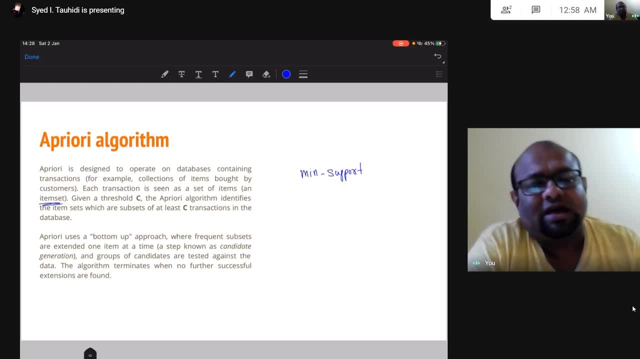 item set containing three items. all right, and then we will eliminate uh three item sets, say: iphone, mobile cover and refrigerator bought five times less than my threshold. going to eliminate them: iphone, uh mobile cover and headphone bought together more than uh say 30 times more than my. 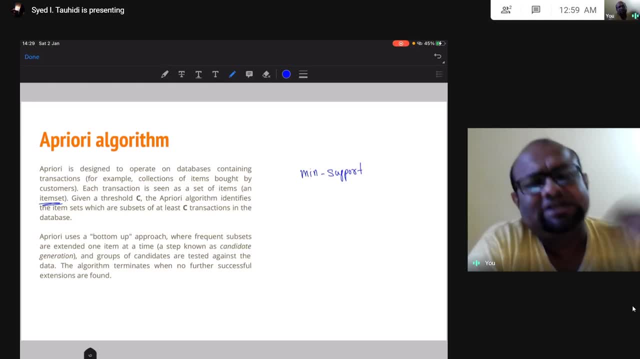 threshold, so going to consider it for the next round. so this is a iterative process using which we are going to generate these item sets that are bought frequently together. okay, so what is our idea of item sets that are bought frequently together? items say that has, uh, that are bought. 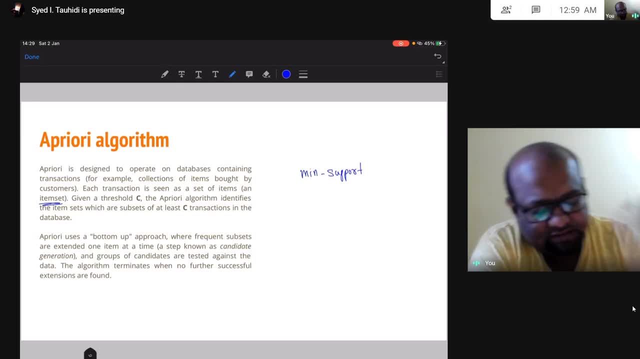 together more than this threshold number of times. this means a good number of times. we are going to say that those are frequently bought together. uh, item sets that are less than threshold number of times, we are going to say those are not frequently bought together. all right, so in this way, we first consider item set of only one item, item set of two item, then 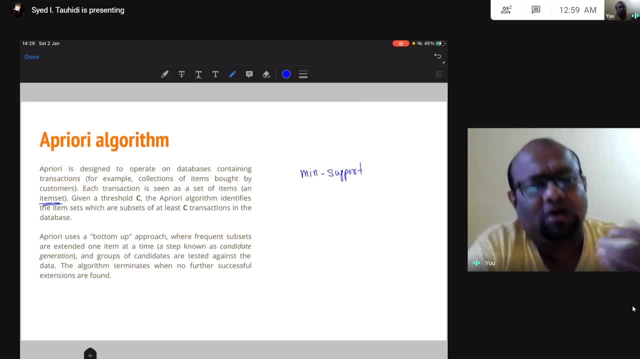 three, then four. we are going to iteratively uh increase the size of our item set by one item in each round. all right. and when we stop, we stop. when we cannot create an item set of larger size, all right. so say, we have come to this point where uh item set uh containing iphone mobile. 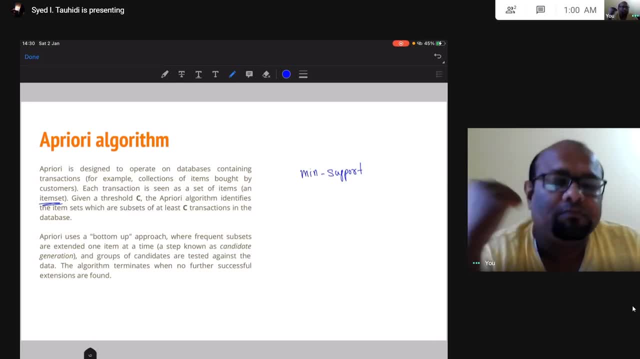 cover and headphone. okay is uh above my threshold? uh, we found that in our last round. okay, then in the next round we try to create item set with these three items and more item. one more item. okay, now we are trying to create item set with full item. now, what do i see? i see that no matter which four item set i make i can, my count is not going. 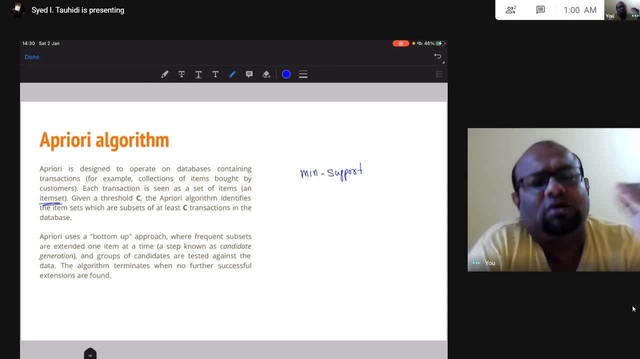 above this threshold. okay, so i and my algorithm at that point now, uh, there is one more thing that i want to talk about. okay, say, iphone and banana is bought less than the threshold number of times. okay, but only two times. so iphone and banana purchase together only two times. now do i consider a set? 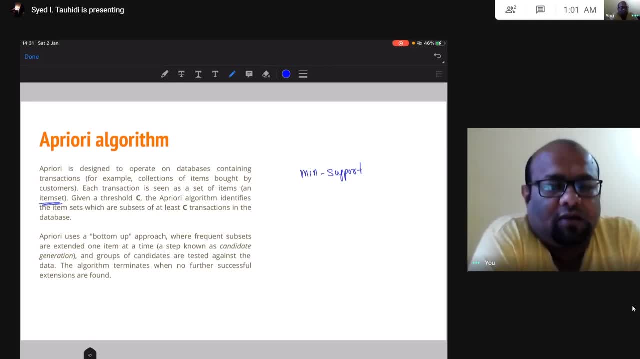 iphone, banana and headphone- okay in the next round. in my previous round i saw that iphone and banana- those things together do not cross my threshold. so if i consider a three set, okay, even iphone and banana is not bought 25 times. so is it possible that iphone, banana and headphone 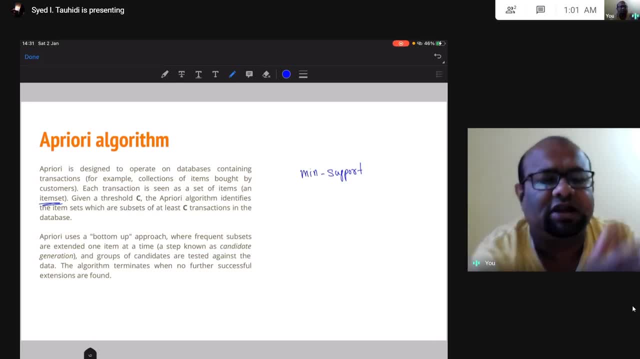 will be bought more than 25 times. it is not possible, right? because iphone and banana itself is not about about more than 25 times. so, uh, the set that i eliminated in my previous round, okay, any set that contains those set that i eliminated i am not going to consider in the next round. so 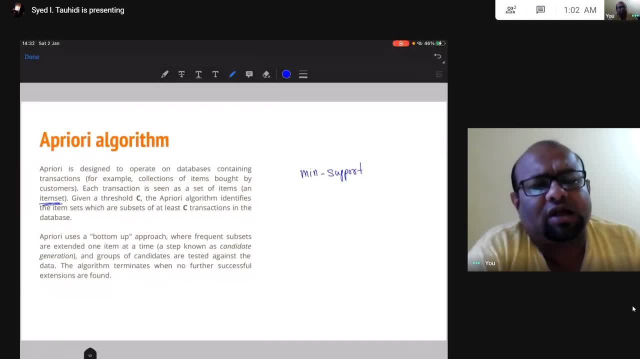 in this way, i do a little bit of uh saving on my computation, all right, so this is called tuning. we are going to do those things as well, you know? uh, this is the basic idea behind a priority. if you did not understand it properly yet, don't worry, we will be applying this on a data set and apply. 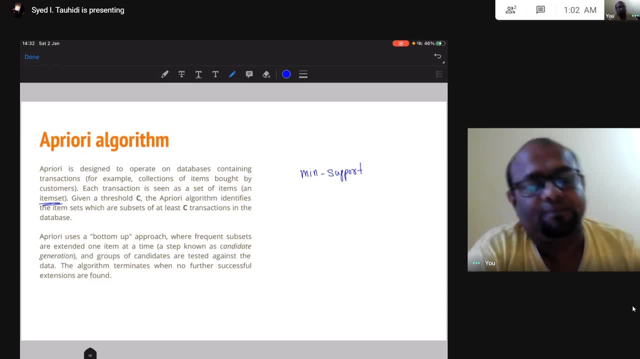 after we apply this on a data set. i hope your understanding of the algorithm will be more distantly. so: a priori uses a bottom-up approach where frequent subset are extended one item at a time. so a priori uses a bottom-up approach where frequent subset are extended one item at a time. so 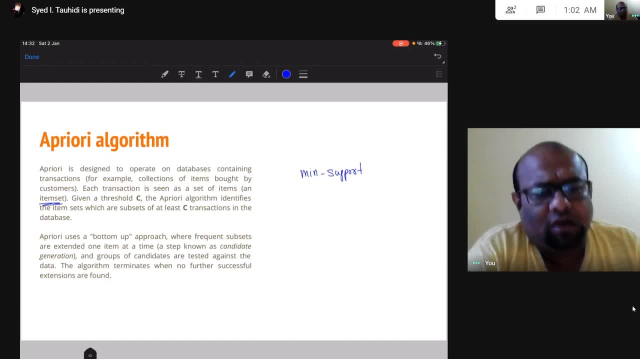 this process of generating sets: uh set of one item, then set of two item, item sets of three item. all right, uh, this is known as candidate generation, all right, and then, uh, we test this uh group of candidates. so how many times uh this item set occurred in the data set? 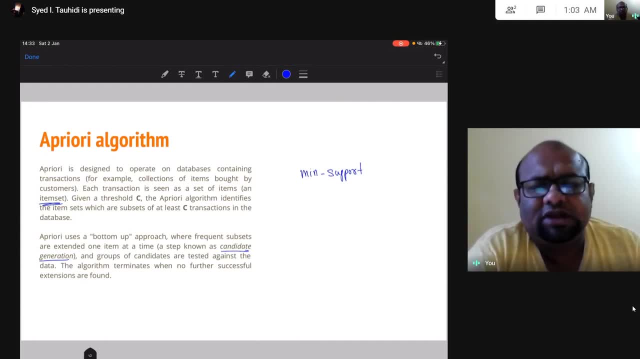 we do those testing, uh the algorithm terminates with no further successful extensions are found, and this is uh the things that i just talked about is written over here. so, yeah, this is uh a priority. let us go ahead and apply a priority on this data set, all right. 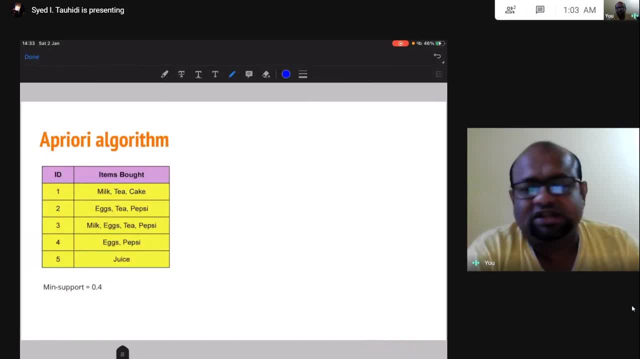 this data set contain five transaction transaction id: number one, two, five. all right, then we have these items: uh, milk tea, cake c and juice. okay, our mean support is 0.4, so our mean support is 40 percent. okay, now let us remember what is support. support is: 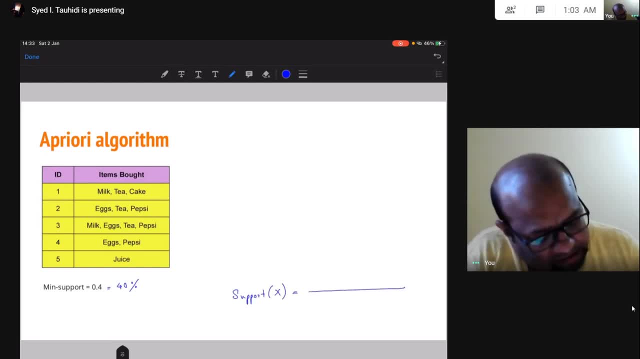 support of x is the number of times this item, set x, will be appearing in my data set in different transaction. in how many transaction does x appear? all right, divided by total number of transaction, all right. so that is the idea behind support. now understand one thing: uh, we are going to divide everything by. 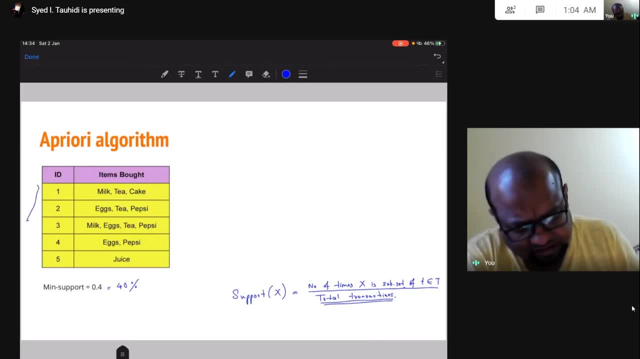 the same number. right here we have total five transaction, so to find support we have to divide everything by five. okay, so we are going to look at: uh, this, uh, this station mean support is our threshold, so we have to find support of every item and every item set and, uh, if the support is below my threshold then i am going to eliminate it. if 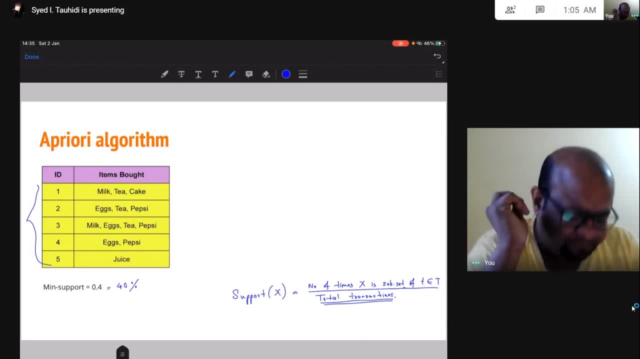 it is above my threshold. i am going to consider it okay. so, yeah, that is something that i am going to do, but i am going to save a little bit of calculation by not dividing by total number of transaction, okay, so anyway, uh, to not divide by transaction, okay, so i have to. 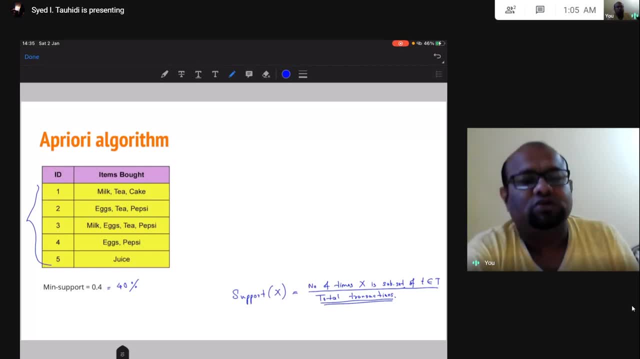 uh, convert this mean support to support count. so i am going to find mean support count. okay, so 40 percent. uh, what is my mean support? what does this say? it says that i have to convert this mean support to support count. okay, so i have to convert this. 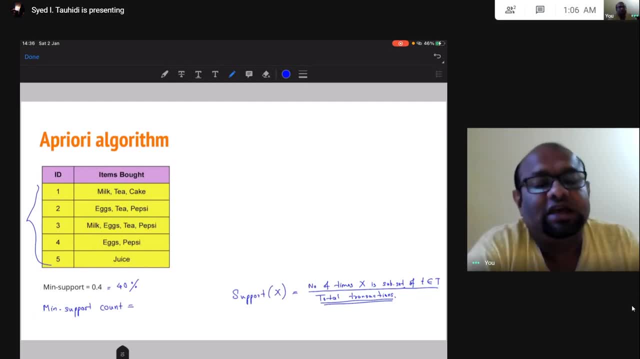 that my, uh, my threshold is 40 percent. okay, so my item set must appear in 40 percent of the transaction. all right, so what does, uh, this correspond to? i have five transaction and 40 percent of five transaction is two. therefore, my mean support is equal to two. okay, mean support. 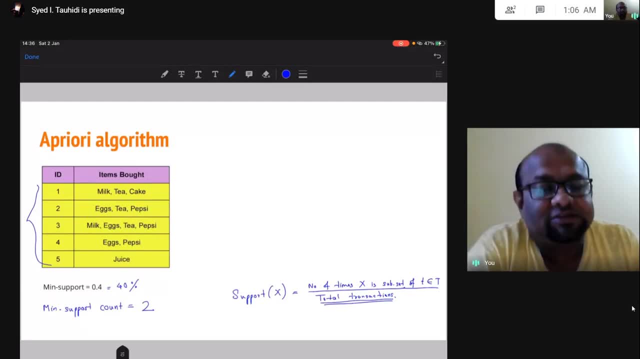 count is equal to two. if uh a item set appears two times, that means uh, it has uh appeared in 40 percent of the transaction. so my threshold is satisfied if it appears two times or more than two number of times. if it appears less than two times, that means my. 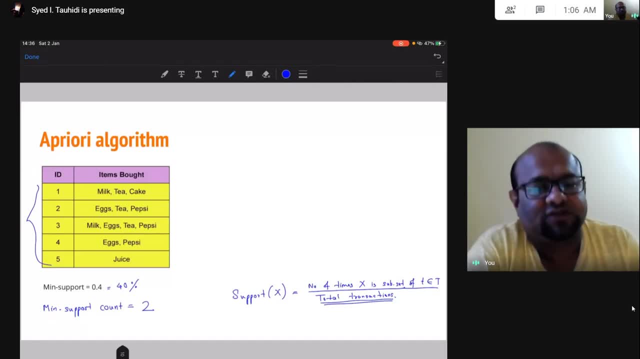 uh, support, uh, my threshold is not satisfied. i am going to eliminate that, right. so that is basic idea. we will talk more about this in the next slide. okay, now, what i am going to do is i am going to take all this item, okay, and write it in this table. so in this table i am going to write all the items. 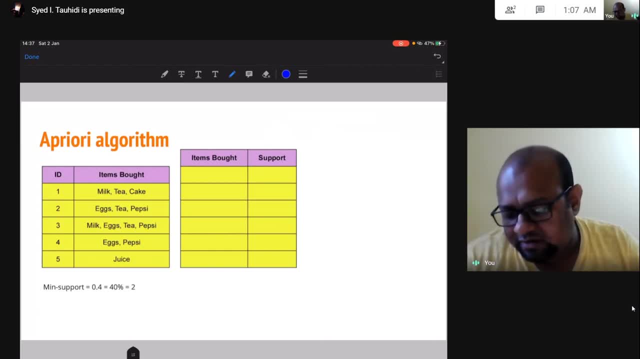 that are available. okay, so what are the items that are available? i have milk, then i have eggs, tea, pepsi juice, cake. so in my first round i am going to consider item set containing only one item. these are item sets containing only one items each. all right, so now i am considering item set. 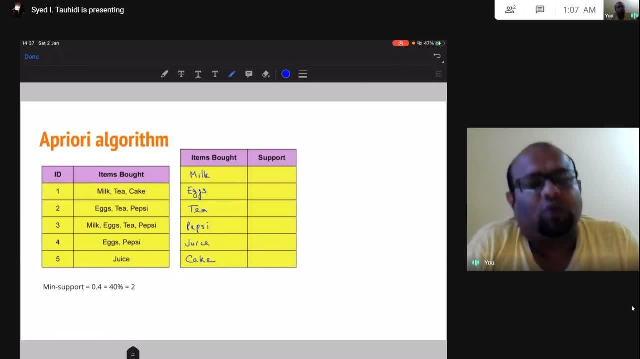 containing one item. all right, now what do i have to find? i have to find support of each item. okay, i am going to find support count of each item. so support, uh, of milk. support count of milk is: how many times do milk appear here here? yeah, two times. 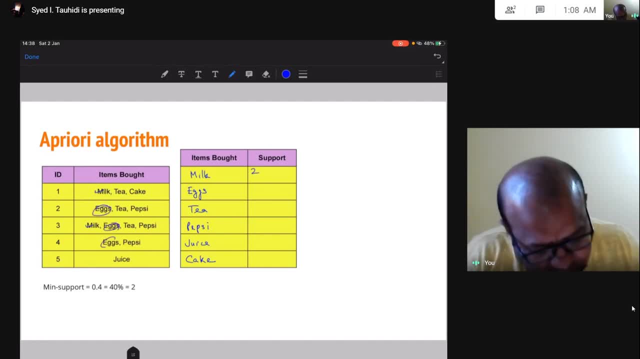 how many times do egg appear one, two, three, three times? how many times do t appear one, two, three, three times again? how many times is pepsi appearing in my data set? one, two, three, three times? all right, Alright. How many times is juice appearing Only once? How many times is cake appearing Only once? Okay, My mean support is 0.4.. I have to find support. Alright, I am not going to do this, but using only support, Not using support count. Let me show you once, and then I will be using the easier technique of using support count instead of using support. 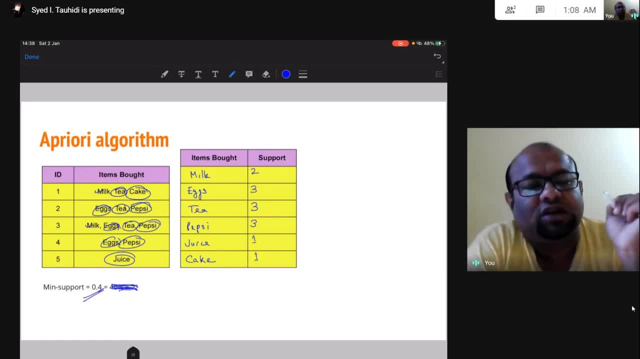 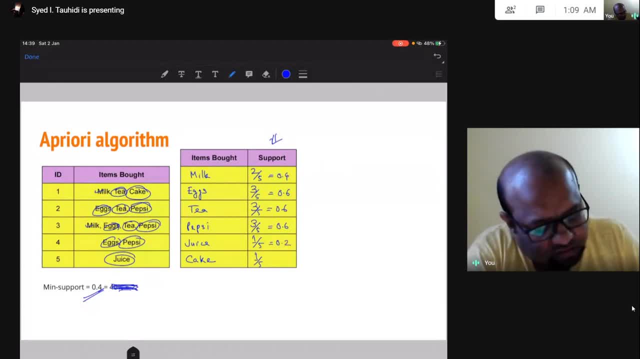 This is equal to 0.6.. this is equal to 0.2 and this is equal to 0.2. all right, so i have found all this support of all this item, all these item sets right now, this item set contain only one item. 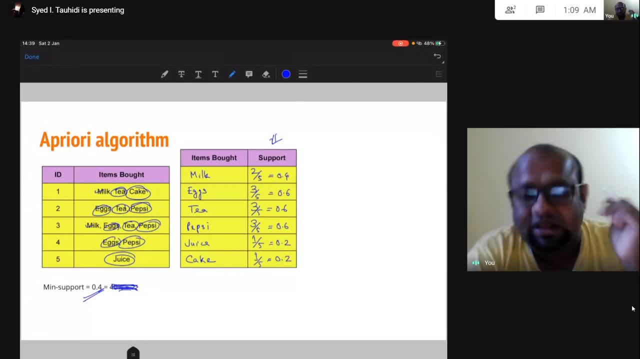 how many of? uh, how many of them satisfy my threshold? this is four. uh, milk is four, so is it uh greater than or equal to my threshold? yes, therefore, this satisfies my threshold. this is greater than my threshold. it satisfies, this satisfies and this satisfies my threshold. okay, 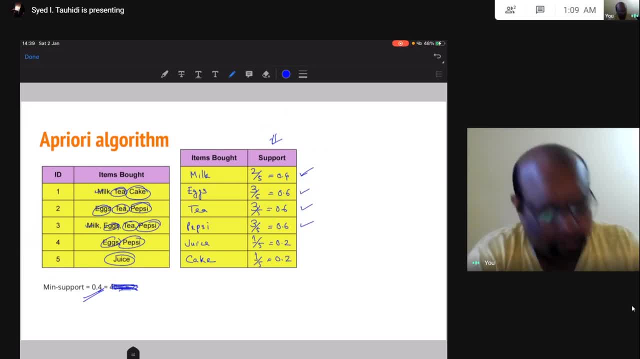 juice and cake. what is the support? 0.2, okay, so support is 0.2. uh, my mean support is 0.4. so juice and cake. the support is not satisfied. all right, the support count is not satisfied. therefore, this and this i am going to eliminate in the next round. okay, so this is what i do, this. 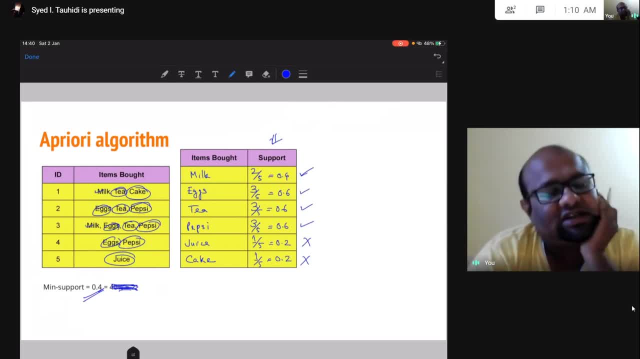 is how i generate item set and then test the item set, and then test the item set and then test the in my data set and, uh, whether it satisfies this testing and whether it is equal to or greater than my threshold or not. all right now, uh, let me mix thing a bit easier. 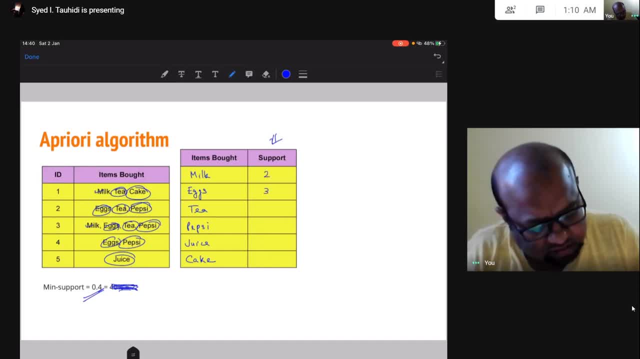 this has a count of two. this is a count of three. three, is this also three? yeah, three and one and one. okay, let me not divide by five. uh, what i am going to do? this support, i am going to find support count. so support count was equal to five. so 0.4 support in this. 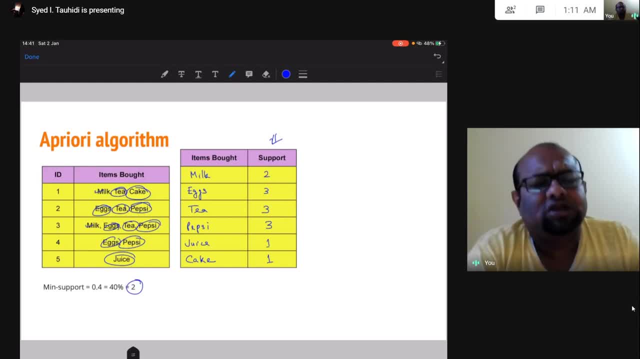 transaction uh means 40 percent of my transactions- should contain the item. that means 40 percent of five. transaction means two transaction. two of these transactions should contain my item. all right, so milk is satisfied like before. all of these are satisfied. these two are not satisfied like before. now only thing is. 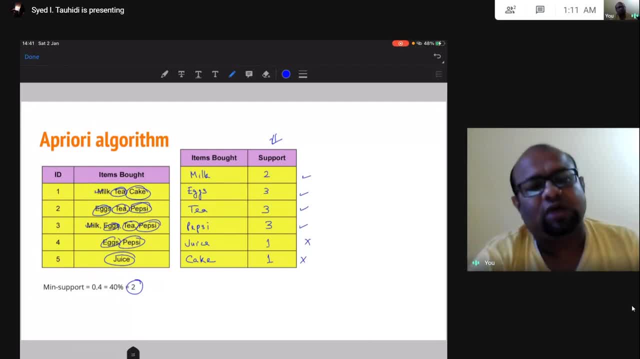 that. uh, previously i found support. now i am working with support count. i did not divide by five, all right, so simple. uh, saving on computation, all right. so this is what i have done. what is the next thing that i have to do? i have to eliminate juice and cake. okay, so i am done. 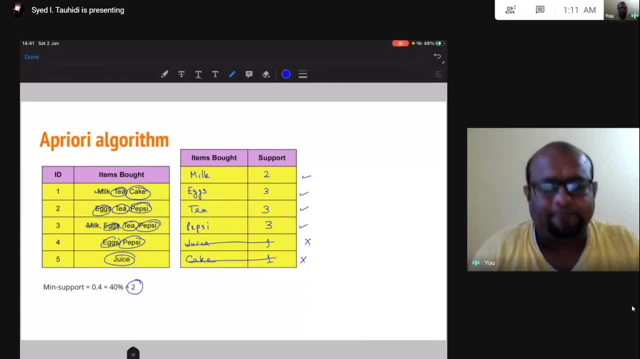 with my first round of- uh, a priori algorithm. all right, right now i have items that are free item sets. okay, all of these are. i'm calling this item easy to call this item because there are only one things, but these are actually sets. each of them is a set containing only one item. okay, so these 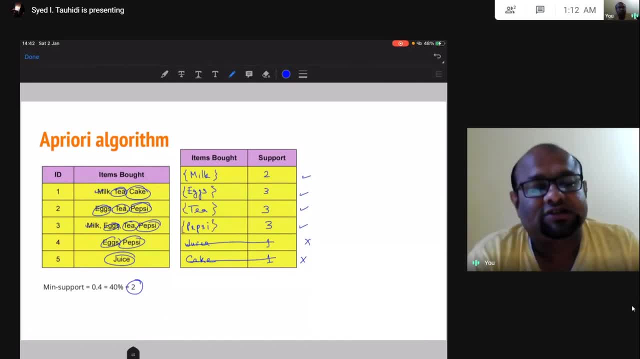 are item sets. think of this as set, not as item. okay, but then there is only one, so easy to say. right? the next thing that i am going to do this round is over. in my next round, i am going to consider set this item set containing two items, so let us go ahead and do that, okay. 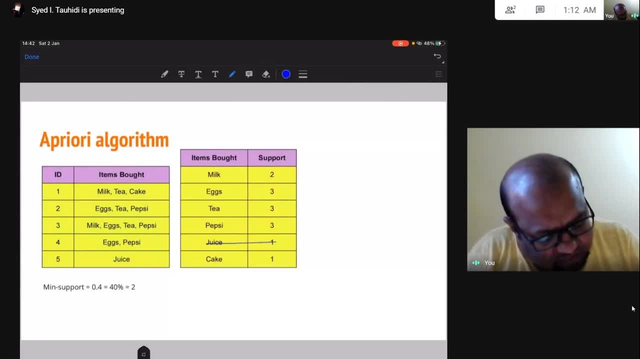 one thing that i have to do is i have to eliminate okay, done eliminating, okay. now i am going to consider items. uh, of two sets. okay means item set containing two items. so let me create this. first milk and eggs, so set containing milk and egg, then set containing milk and tea. 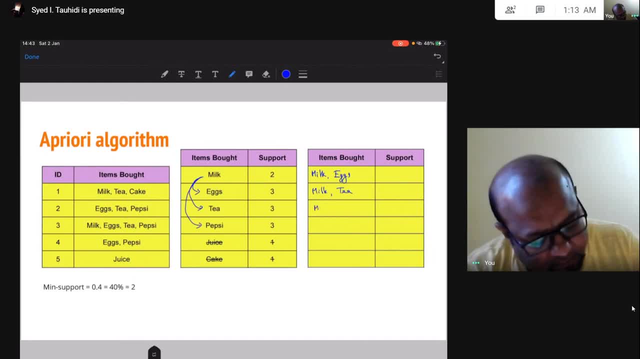 then set containing milk and pepsi. do i consider set containing milk and juice? okay, what am i going to do? i am going to find items that are frequently bought together. wow, what is my measure of frequent, if this means about count, if items are bought together, item set. 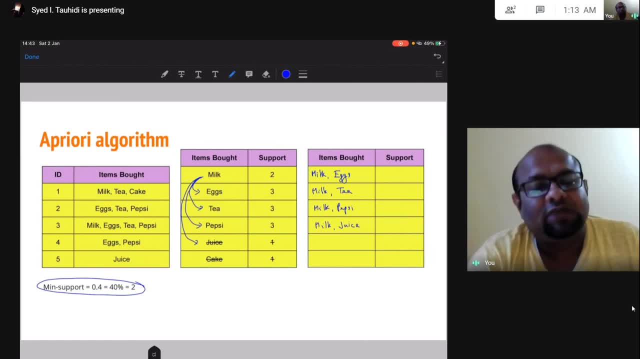 is has a support count of two. if item is bought more than this item, set is purchased together more than two times, then i am going to say that, uh, it is frequent, using some sense of frequentness. okay now, uh, here is uh something to consider. okay, juice is bought only once. 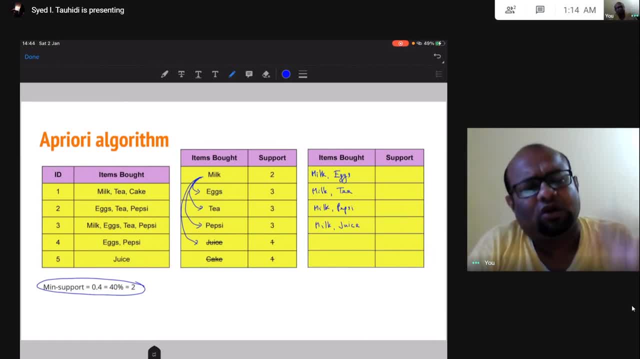 all right. out of all this transaction, only one transaction contained this item, juice. so juice by itself did not satisfy my threshold. my threshold was two. okay, i am trying to find item set that are going to satisfy my threshold. so is it possible that milk and juice will satisfy my threshold? think about it. juice itself is. 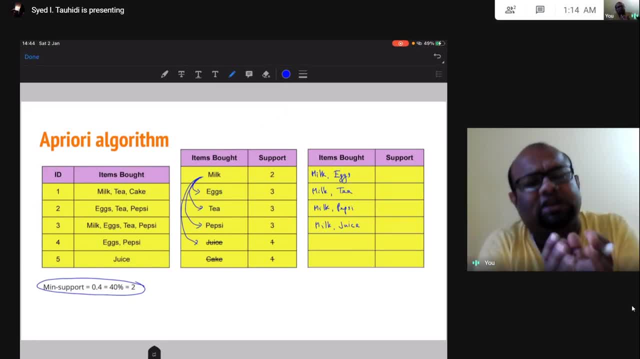 purchased once. so milk and juice together can be purchased only once. right, it cannot be purchased more than once, otherwise juice purchase will also be more than once. so juice itself did not satisfy my threshold, so milk and juice together. juice alone did not satisfy, so i am making it more. 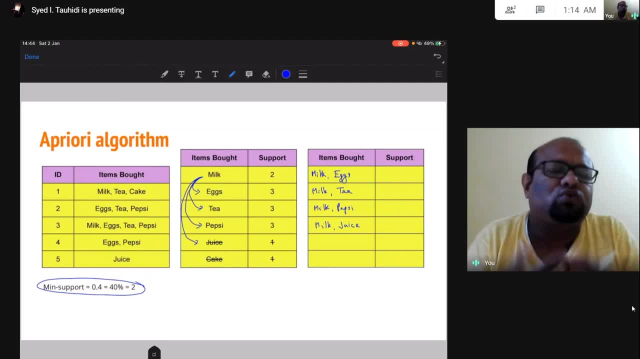 restrictive by combining milk and juice. these two together, how can it satisfy? okay, therefore, i do not need to consider this. any set that contain juice and any set that contain cake can never satisfy my threshold. all right, because this item alone did not satisfy my threshold. so So this item combined with something else, how can it satisfy my threshold? 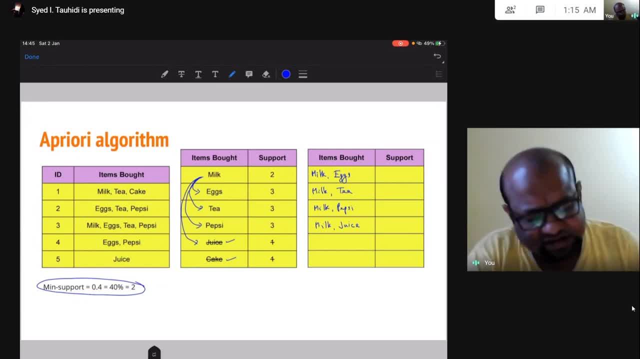 Therefore, I do not need to consider any set containing milk or any set containing juice. I do not need to consider this item set. Alright, let me remove this Fine. Next, what is remaining? I have to make this item set. 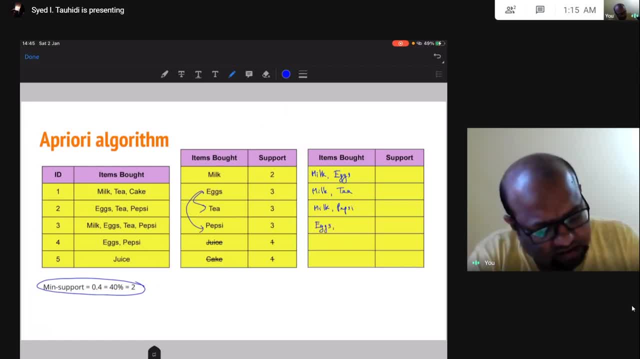 Eggs and tea and eggs and Pepsi Done. Next, only one is remaining: Tea and Pepsi Done. These are all the possible two item sets. Alright, Now I have to find support Support count I can use find support. 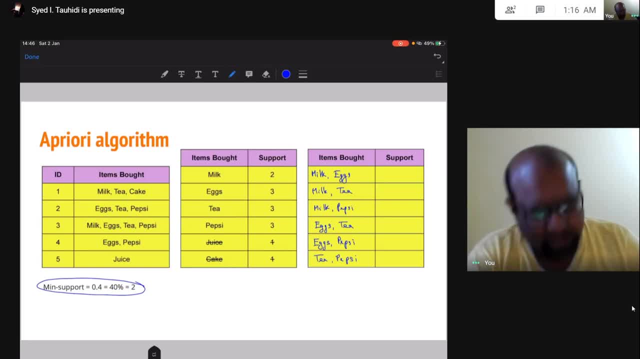 That is, divide support, count by number of transactions, Alright- And then compare with mean support. But, Like before, I am going to find support, I am not going to do this division. So let's go ahead and find the support. 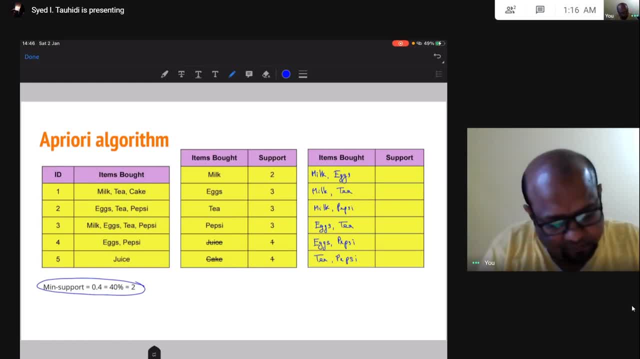 How many times is milk and egg appearing in the data set? So milk and egg first. Milk and egg is appearing here only once. How many times is milk and tea appearing together? Milk and tea is over here. Milk and tea is over here. 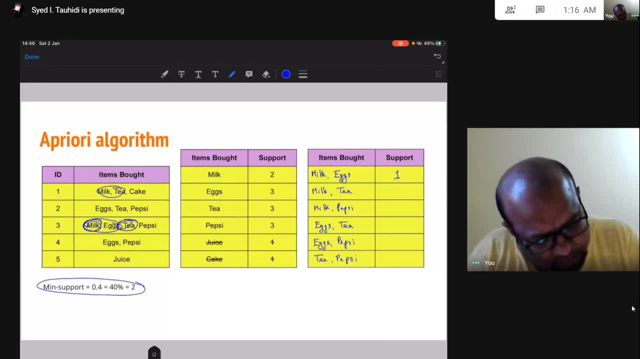 So two times. Yeah, How many times is milk and Pepsi appearing together? This is milk and Pepsi over here only one time. How many times is egg and tea appearing together? Egg and tea is over here. Egg and tea is over here. 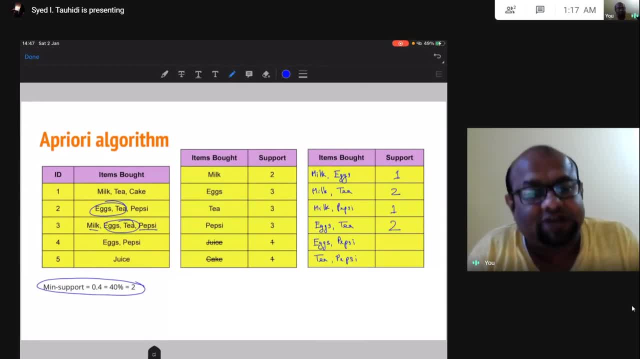 Two times. How many times is egg and Pepsi appearing together? Egg and Pepsi is over here. Egg and Pepsi is over here. Egg and Pepsi is over here. okay, so three times. how many times is t and pepsi appearing together? two times, all right. so do this count for yourself. t and pepsi over here. t and pepsi over here two times. 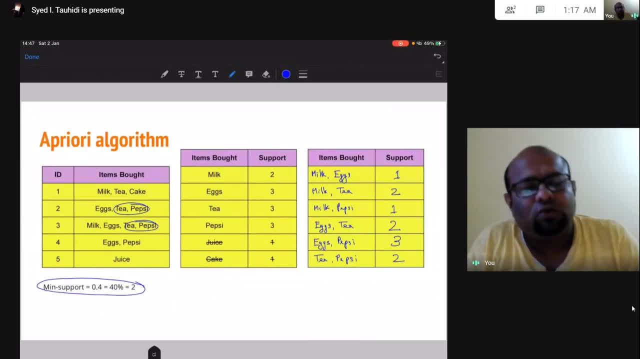 okay, so i have found the support. now what do i do? i do this test, test against this threshold. what is my threshold? two. so, uh, support count mean support count is two. so item set with support count less than two: i am going to eliminate them. so i am going to eliminate this item set containing 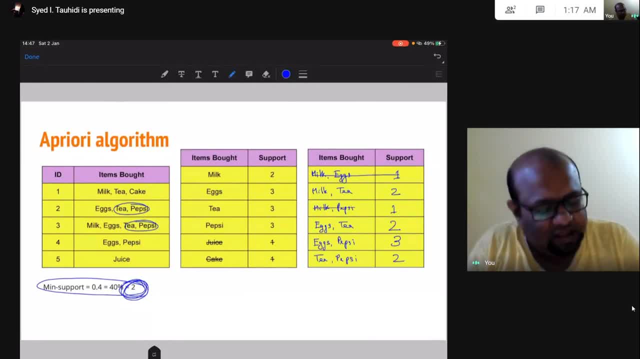 milk and egg and i am going to eliminate this item set containing milk and pepsi. all right, so now i have generated this frequent item set containing, uh, this four frequent item set. so this, this, this and this. what does this mean? i see that eggs and pepsi are often bought together. okay, so i 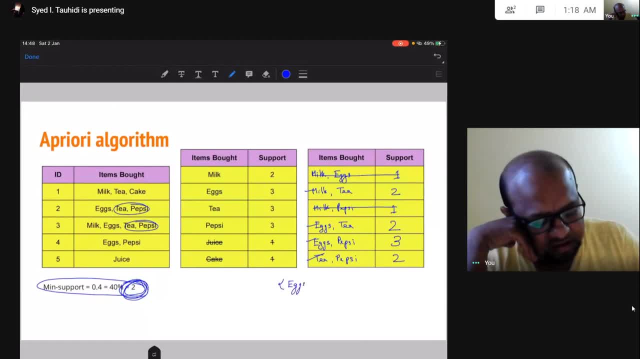 am going to say eggs and pepsi. these are frequent item set, okay. these are frequently bought together, okay. so this is uh brought together three times, then egg and tea. this is brought together two times, then milk and tea, two times, then tea and pepsi, two times, then tea and pepsi. 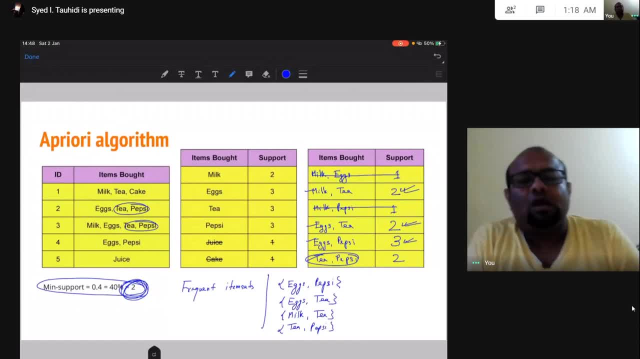 two times. okay. so this is how i have generated the item sets which are frequently bought together. right now in this round, i am looking at item sets that contain two items. all right, so i have this now. uh, let us consider this frequent item set, okay. uh, did i generate association rule yet? 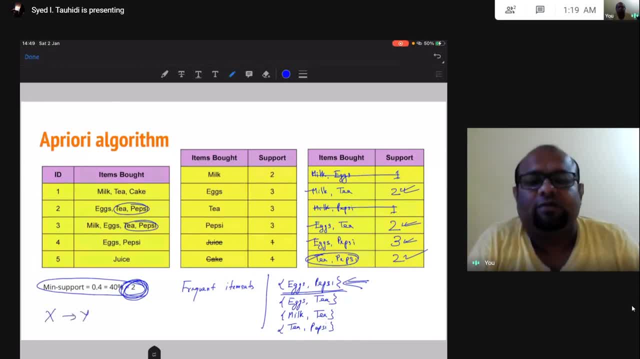 a rule is a implication of this form: x implies y. i still do not have x implies y. okay, so there are two possibilities over here. i can do x implies pepsi. i can do pepsi implies x. so a person has got x, also got pepsi. a person who got pepsi also got eggs. okay, these are two. 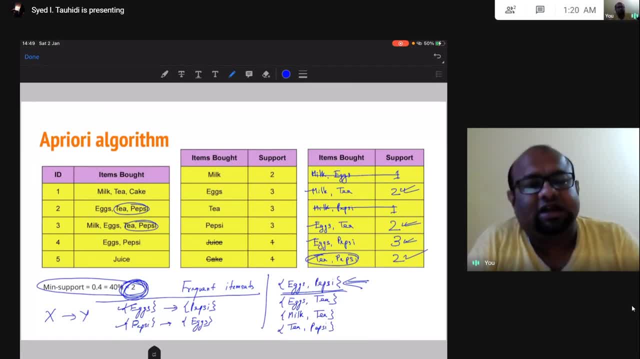 uh, rules that i can generate using this frequent item set. similarly, using this frequently, it attempts, and i can generate other rules as well. okay, so that is how i generate rules. now there are more intricacies over here. okay, is both of them? do i select both of them or do i prefer one over the other? all right, so if i have, 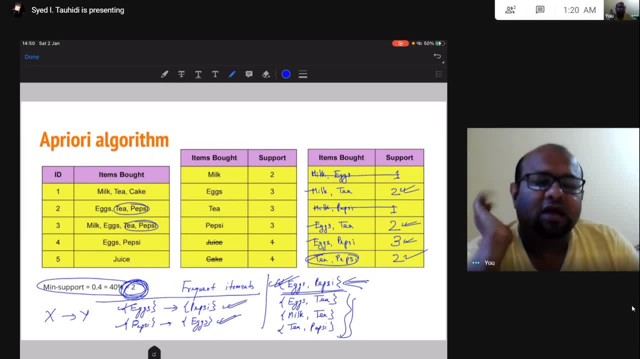 to select one boot. which one do i select? and there are more examples that we have to take and look at a few internet details that we will talk about at the very end of this video. okay, now our focus is on getting this set of items that are frequently bought together. we will be looking at how to 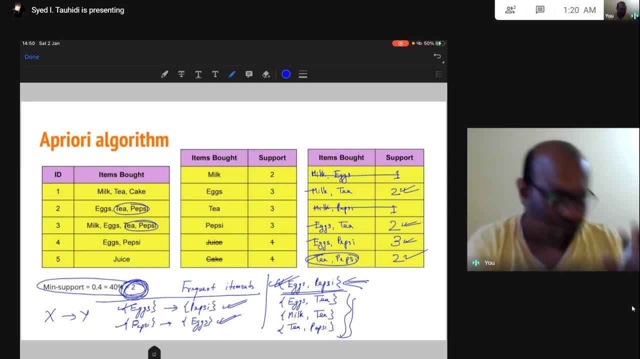 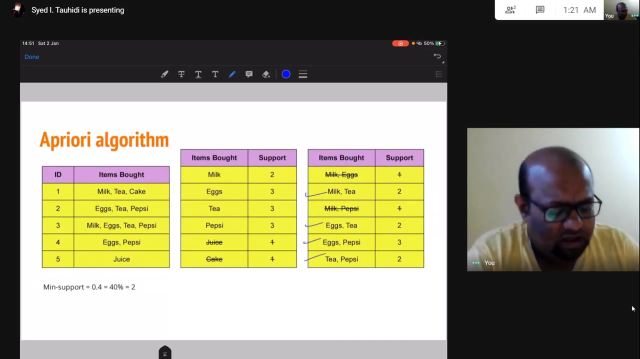 generate rules later on. okay, so let us go ahead. we have generated item sets. these, these: these are these that are frequently bought together: this item set containing two item. next, let us go ahead and do this. okay, so done. we have created four item sets. now let us go ahead and generate item set containing three items. okay, now let me. 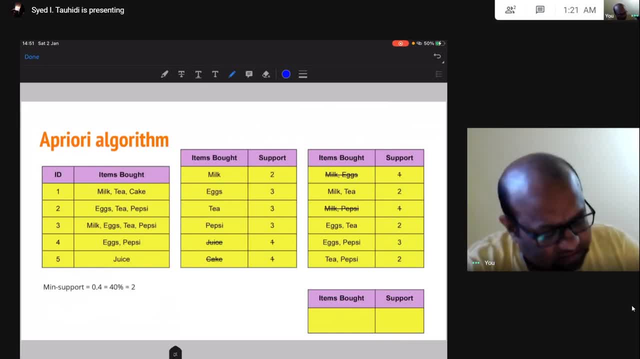 try to create the first item set, say item set containing milk, eggs and tea. do i consider this item set? do i scan my data set to find how many times this appears in my data set? what is the support count of this? i have to find the support count of this and then i 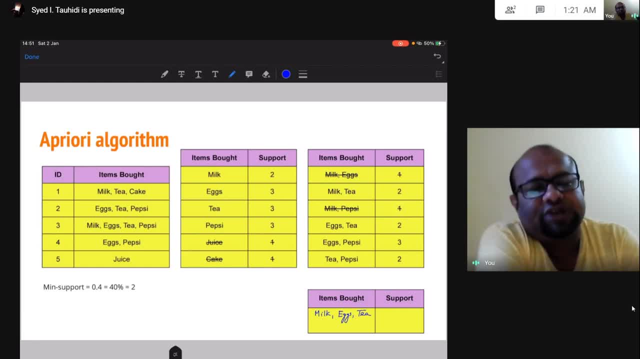 have to check, against my mean support, to see if the threshold is satisfied. okay, do i do all this calculation, or lots of computation, has to be done. see milk and egg. these two together is bought only once. okay, so milk, egg and tea, this three item, cannot be more than once. that has to make sense, right? milk and tea itself is bought only. 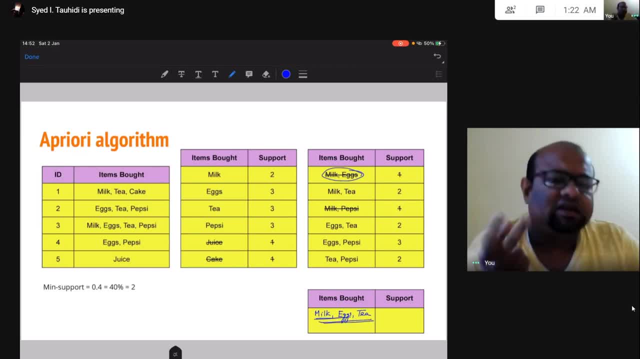 one time. so milk, egg and tea, these three item together cannot be more than one time. okay, so i do not need to consider this. what do i consider? anything that contain milk and tea? any set that contain milk and pepsi, i can eliminate, all right. any set that contain juice, any set that contain cake, i can eliminate. so i will take only 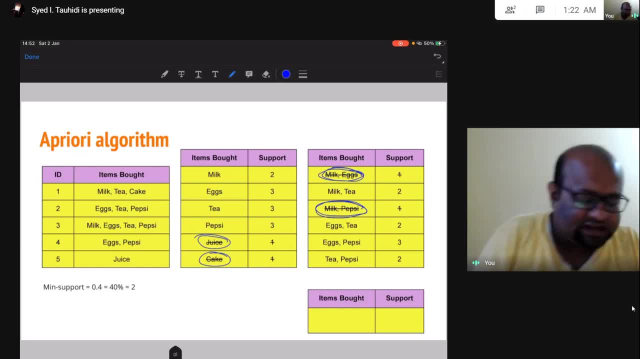 those sets that do not contain any of this item. okay, so let me go ahead and find one of those sets. there is only one set that is possible, okay, and that is eggs, tea and pepsi. okay, let me see how many times these three appear together. xd and pepsi is bought together here once. 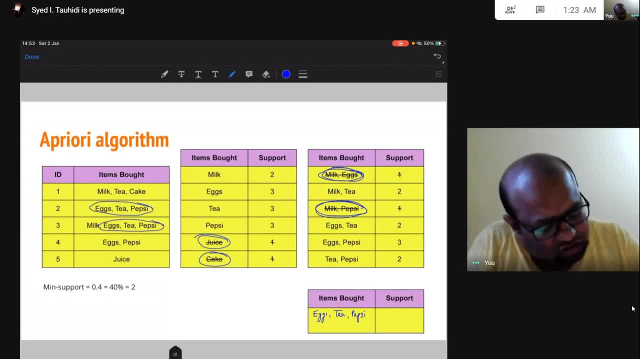 so support is true means support is satisfied and we can. we have this frequency. you can try for your uh, for yourself, and try to find other frequency, other item set containing three items down. we have a product name and a product type that has a support greater than or equal to 2. greater than or equal to the threshold. 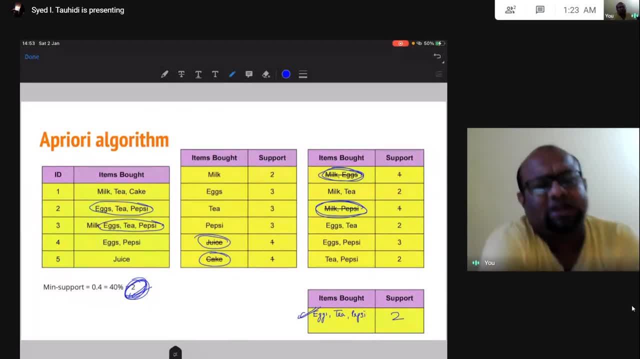 so do that for yourself, okay. and when trying to generate this item set, remember this thing: if you take the item set containing juice or cake, okay, you will not be able to satisfy the threshold. if you take item set that contain milk and egg or milk and pepsi, you will not be able to satisfy the threshold. i hope you think about it. 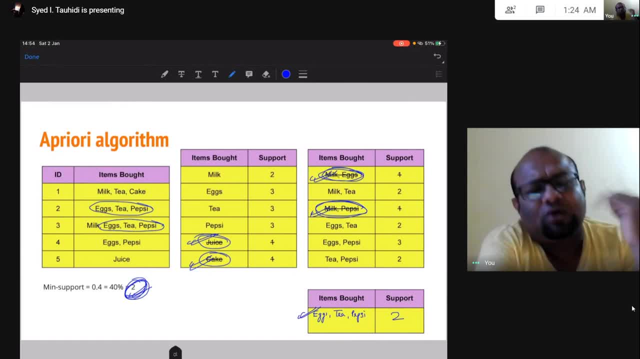 what support means, how we are calculating support. okay, don't just uh look at method to calculate, to calculate. try to understand what we are calculating, okay. so i cannot force that into your mind. you have to really uh sit with a pen and paper and think, okay, there is nothing that can. 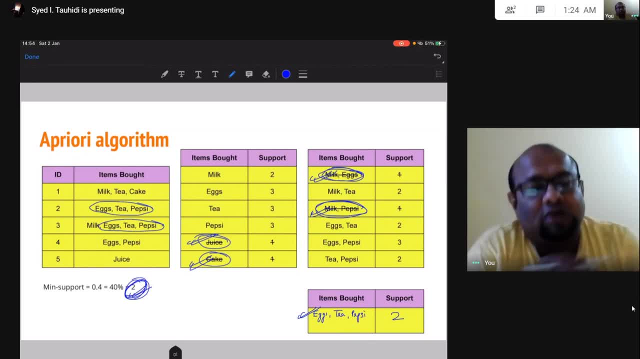 substitute for thinking: okay, i cannot, i can just teach. i cannot do the thinking for you. you have to think on your own. so think, okay, why we are doing this pruning, why we are doing this elimination, why we are not taking any three item set containing milk and egg. okay, so try to find some other three item set. 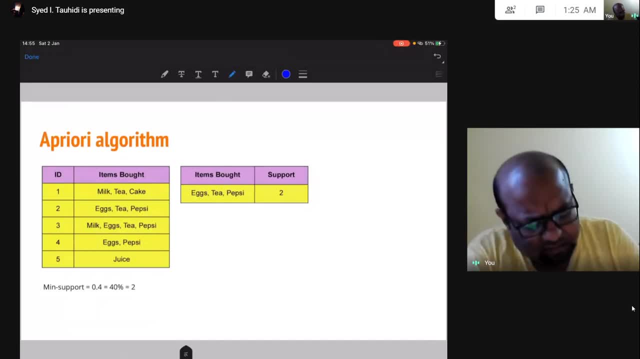 and i found only one, and then i am unable to find any four item sets. so if i take eggs, tea, pepsi and anything, okay, uh, say milk, milk, so this contains egg and milk, and egg and milk was already. if i buy egg and milk together, then i will not be able to satisfy, so i can satisfy them as well. so now let's see the another. 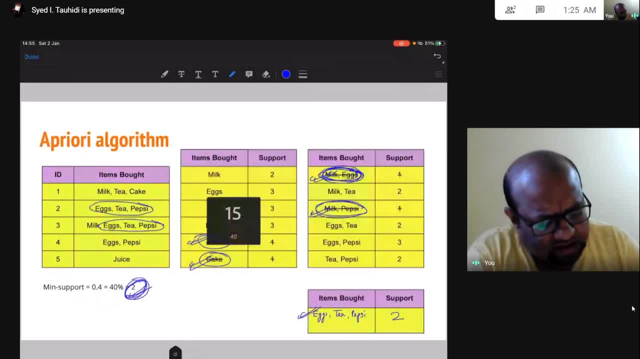 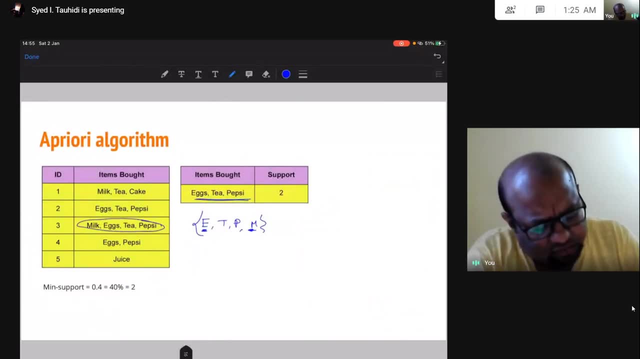 things which have been done so far. that means the product has been given the right amount of time. egg and milk. this contain egg and milk. i am not able to satisfy this support is only one. okay, my threshold will not be satisfied. and if i take anything else, my instead of milk, if i take 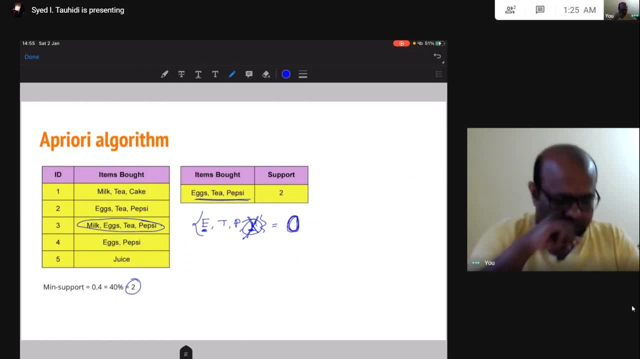 anything else, my support will be zero. that will also not satisfy the threshold, so there is not going to be any four item set that i can generate. okay, right now i am able to generate this one three item item set, so i will be able to do this if eggs and 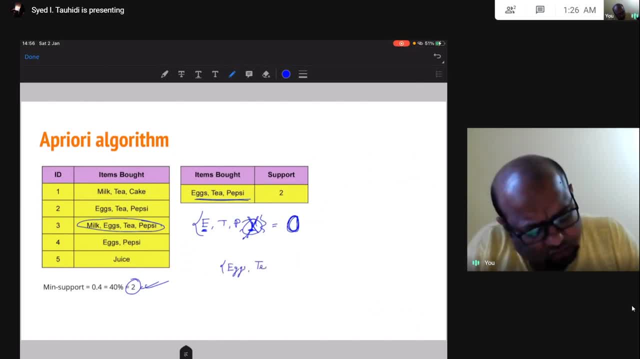 tea are brought together. so let me create a rule: suggest pepsi. or if eggs and pepsi is brought together, suggest tea. if pepsi and tea is brought together, suggest egg. okay, these are the kind of rules that i will be able to generate, or in a extreme case, i can do this if pepsi is brought. 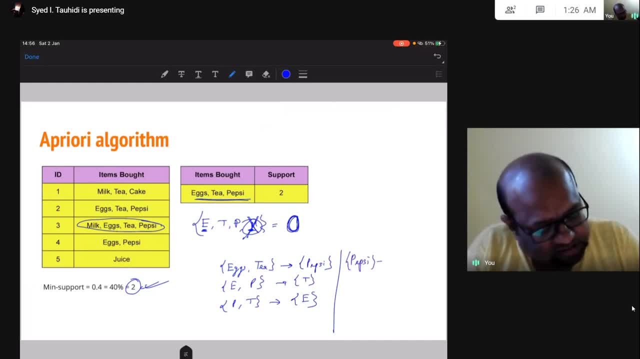 suggest eggs and tea. okay, these are also rules that i can generate. okay, now, if i keep on generating rules like this, i will be ending up generating lots of rules. okay, so not all of these rules are going to make sense. out of all these rules that are. 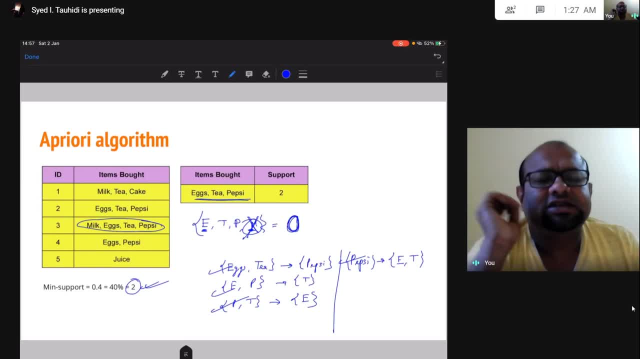 possible. i will be able to generate lots of rules. okay, so not all of these rules are possible. which makes sense and which do not make sense? we are going to talk about that at the very end of this video. okay, so fine, this is a priory algorithm. okay, up to this point. what? 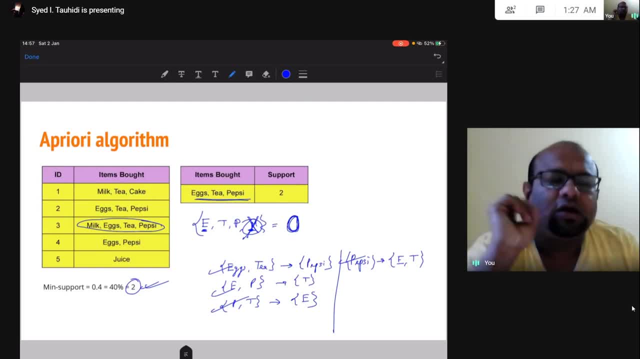 we have done. first, we looked at item set containing only one item. okay, we found their support. we tested against the mean support count. then we eliminated- uh, this item set containing only one item. we eliminated those which did not satisfy this the threshold. then we created two item item set containing two item. we did this test again. we 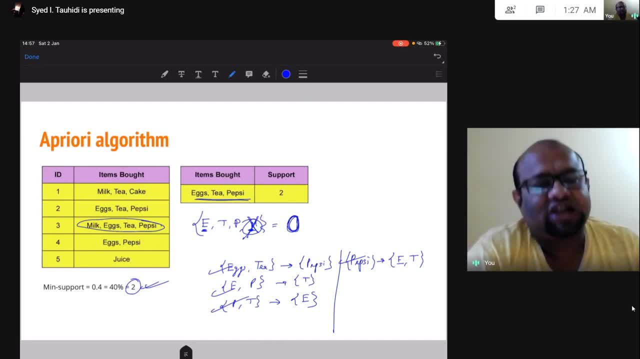 eliminated again. and then we created item set containing three item. did the test again, eliminated again. then we saw that we cannot create any item set containing four item. okay, at that point we are stopping our algorithm. we have created item set, frequent item set, item sets that are: 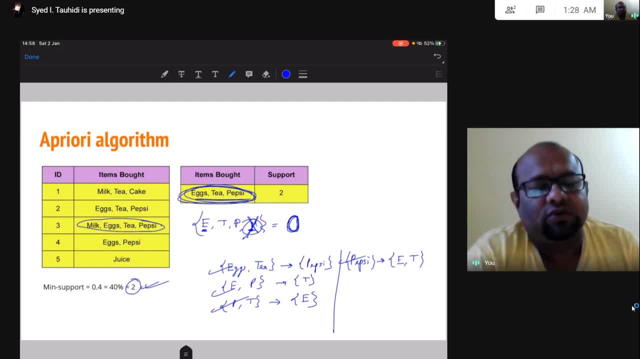 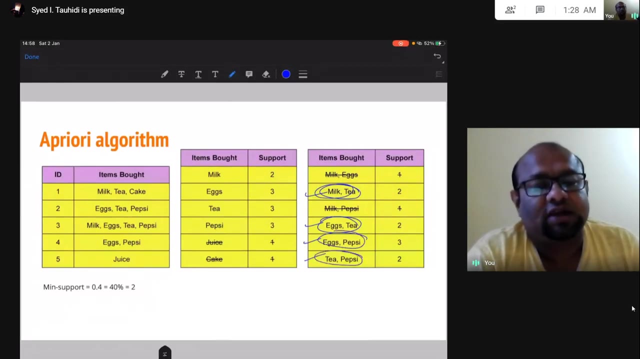 frequently brought together. okay, items that are frequently brought together. this item set of three items and this item set containing four items. sorry, two items. this four item set containing two item. all right, so this is what we did up to this point. this is what we are going, we have done. 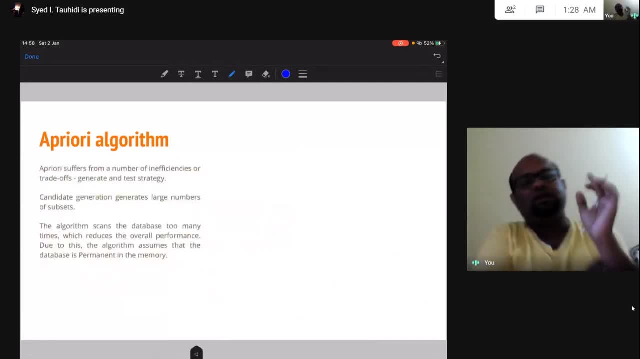 in a primary algorithm. now let us talk a little bit more about a priori algorithm before we move on to the next topic. okay, remember, we did not generate rules yet. okay, our main target in this video is to generate association rules, not to generate frequent item set. frequent item set is: 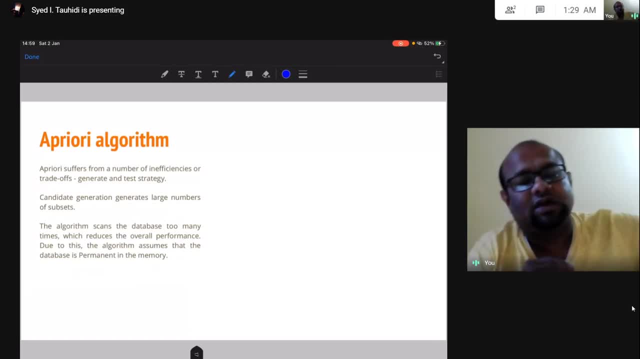 the meat station of what we are doing. okay, our ultimate aim is something else that we will do at the very end of this video, but let us generate this frequent item set right now. okay, because all this item, all these algorithms, are going to generate frequent item set. so these algorithms are different, but 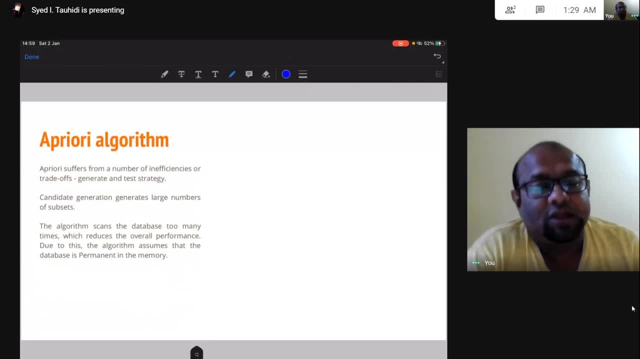 which, from this frequent item, set which rule to generate that is common between all this algorithm. okay, so lots of items, yes, in there. we are going to talk about that at the very end. now let me end this part about a priori algorithm by talking a little bit about some issues that are there. okay, a priori is very 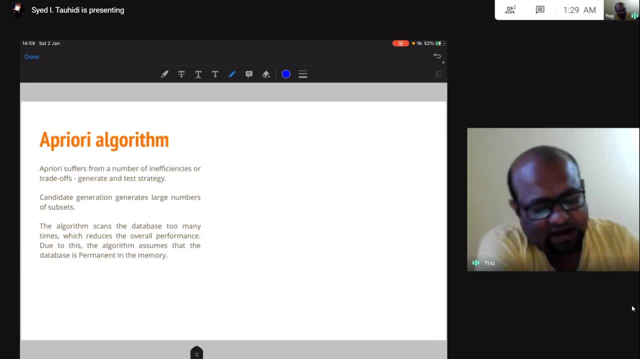 ineffective. why? because if there are n number of items, then there are going to be two to the power n number of possible subset of this item. so there might be two to the power n number of different uh items sets that we can generate out of this n. now, this is not exactly two to the power n because uh. 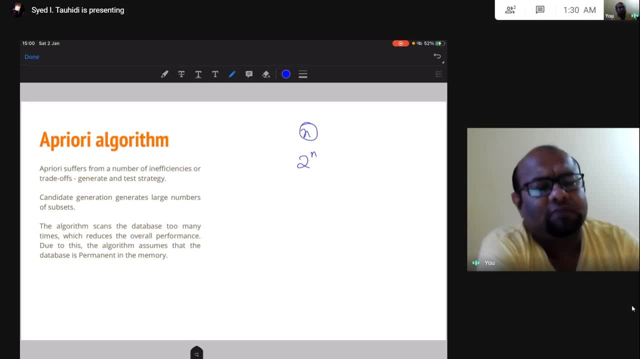 we are never going to consider an item set containing no item. so null we are never going to consider. so it is actually at max going to be two to the power n minus one, but then for all practical purpose, uh, it is still exponential, not going to make a major difference to the number of 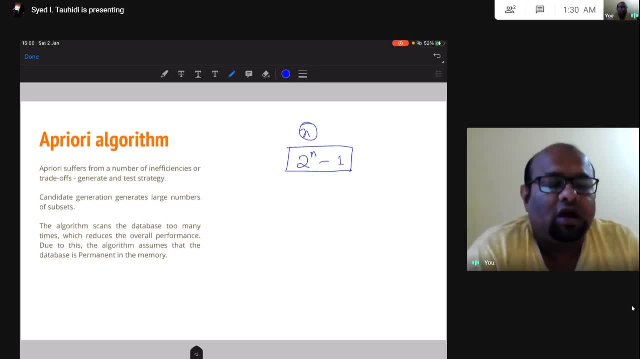 computation that we have to do. all right now, yeah, this is true that we will do. pruning, this is true that we are going to do. we are going to stop much earlier. we are not going to create all 22 to power n, but this is still a large number of calculation. all right, this strategy of generating this candidate, candidate. 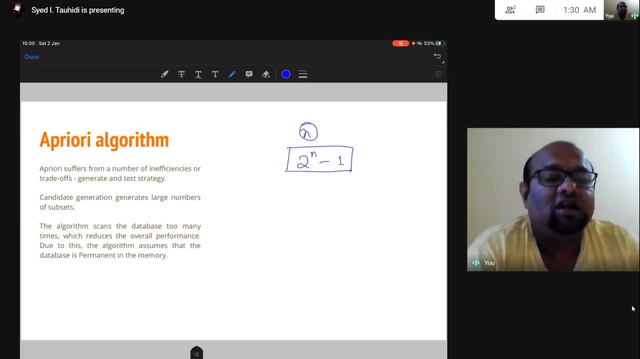 generation, generating this item set and then counting, finding the support count and then testing against the mean support- much faster than what is connected with typography charging. lots of task is there and for each item set that we generate we have to scan the data set once and find the count. so we have to do lots of scanning of the data set. all right, that is. 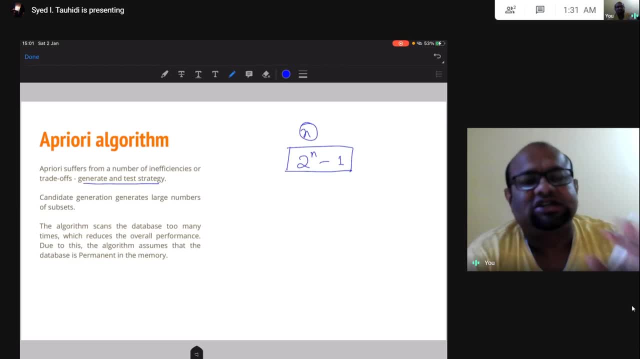 another problem. so generate and test is a large uh is a ineffective thing, then candidate generation will generate a large number of subset. exponential number of subset. that is another problem. and then this: the algorithm is going to scan the data set to count, to find the support count. we 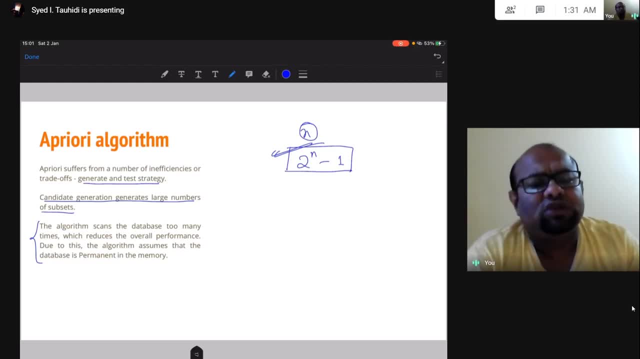 have to scan the data set, all right. and we have to do this for each generated item set. so this is also problematic. all right, uh, if our data set is in hard drive, then what is going to happen in our secondary memory? we have to take it to our ram, and then we have to from ram. we have to take it to cache, but forget cache. 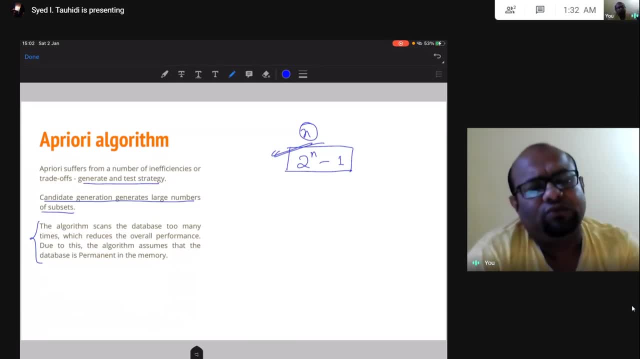 say we are counting directly in ram, still we have to bring everything from hard drive: count, remove it, then take more from hard drive. okay, if we have tbs of data and we have, say, only a few gb of ram, okay, then uh, several times, if we scan the data set, we have to bring everything to. 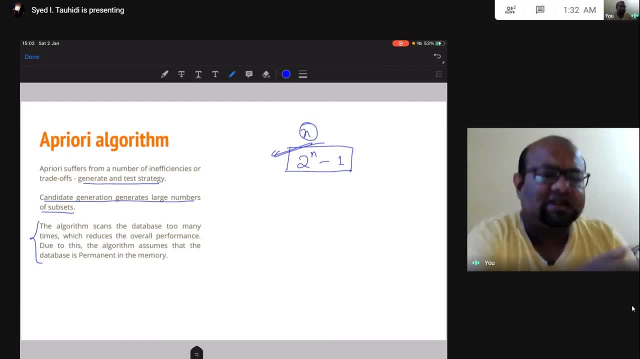 ram several times do computation and then it's in the next one. we have to bring it to ram again do computation. but this is this is very ineffective. okay, the algorithm assumes that the data set is there permanently in our ram. okay, so if the data set is entirely there in our 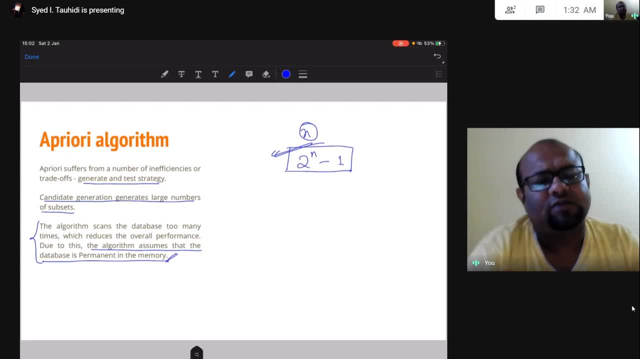 ram, then this transfer of data from hard drive to ram that is going to be saved. and now remember one thing: hard drive is very slow. okay, it's a mechanical device that rotates, all right, unlike electronic. electronic device works in light speed, but mechanical hard drive is mechanical, it is a physical thing that rotates. it cannot be that fast light speed. 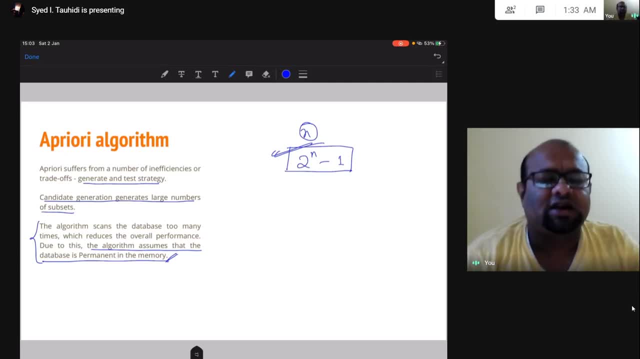 okay, now we have ssd. that's a different type of hard drive. that is electronic, no mechanical part inside. but then ssd is so expensive. you cannot have big data kind of calculation in ssd. okay, that does not make sense. okay, you cannot spend that much money on doing this computation. so if you 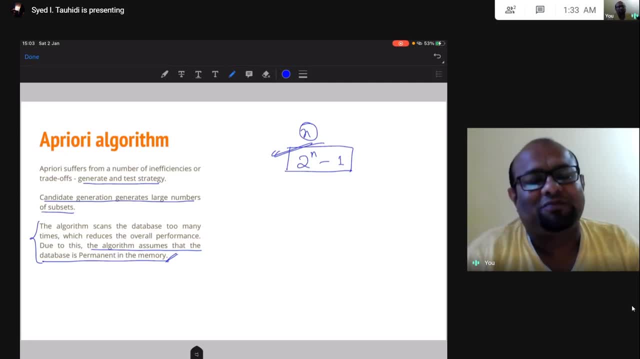 uh, if your computation takes more money than the profit that your company is going to make, that that would not be efficient thing to do. so these are some problem with april, all right. so because of this problem, we are going to look at a different algorithm that uh tries to minimize some of these problems. okay, so we will be looking at the next algorithm. 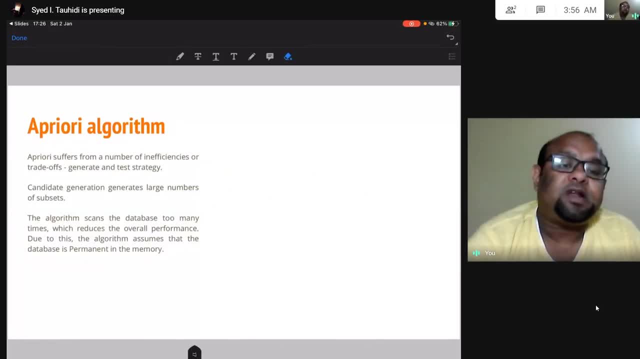 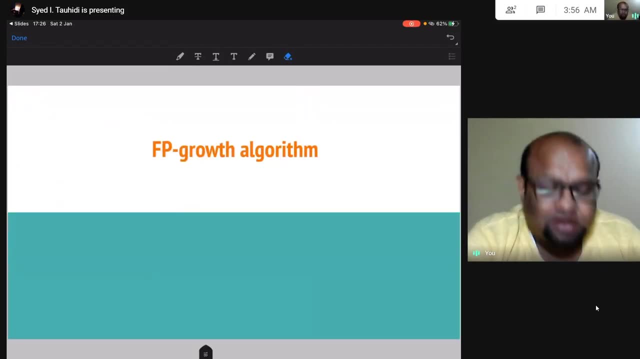 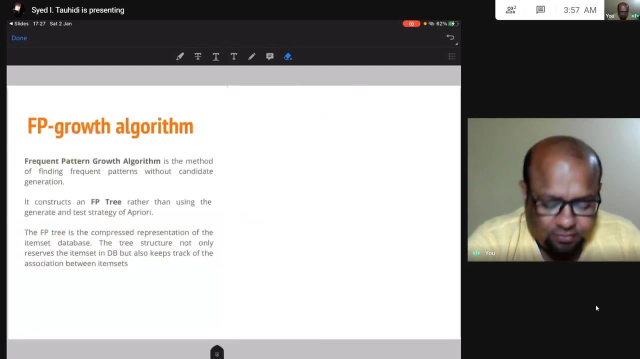 now, the algorithm that removes the problem, that a priority has, is the fp growth algorithm. i mean, there are other algorithms, but we are going to look at fp growth algorithm, all right, so let's talk a bit about fp growth algorithm. uh, the full form is frequent pattern. 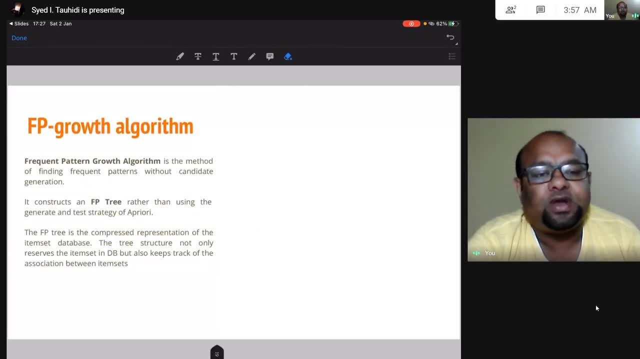 uh growth algorithm. it is a method of finding frequent patterns. this frequent item sets that we found in april. we can find them using fp growth as well. but, uh, the difference is that, uh, here we do that using uh, without doing this. candidate generation- all right, so we could potentially 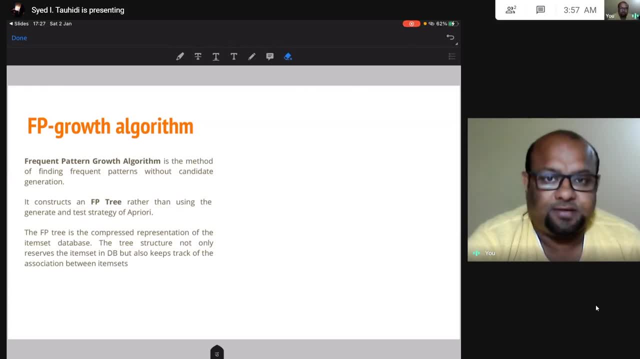 generate a exponential number of uh item sets in april. here we are not going to do that. so that is a very big saving in uh computation. right in april we generated up to a max of uh 2d to power n minus one uh atom sets. we will not generate that, okay, because we will stop early. we are going to do. 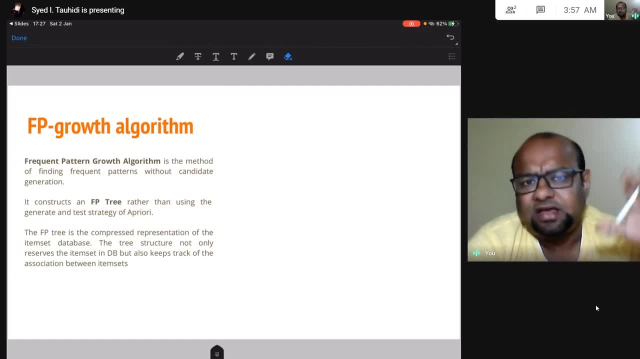 pruning in a priority. there are lots of techniques in a priority, uh, because of which we do not reach this theoretical maxima, but then that is a possibility. we could reach that maximum right and then for each of the item set that we generate each of these generated candidate. 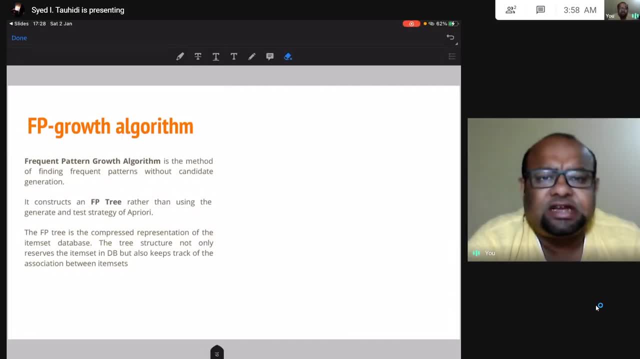 okay, what we did was we scanned the data set and then, uh, we counted the support right and then we did a testing against this mean support. now we are not going to do all those kind of things in fp growth. all right, we are not going to generate uh candidates. 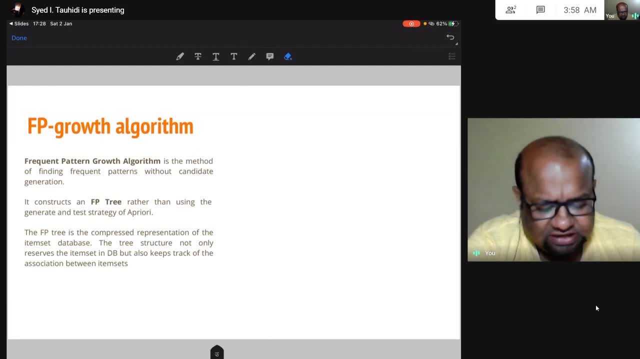 all right, so that is one major advantage in a pig road, right? so here, instead of doing all those things, we are going to create something called a fp3- frequent pattern tree, so we are going to create a tree-like structure rather than, uh, this generate and test strategy that we did in april. 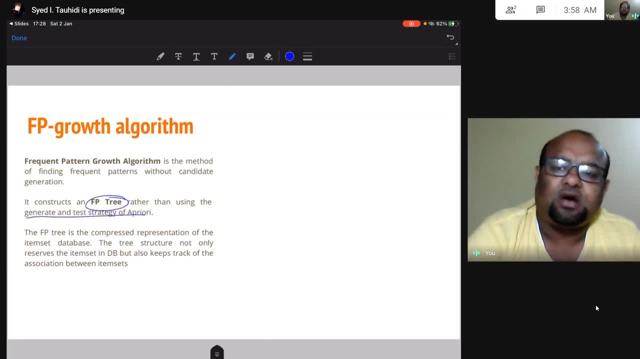 so the fp3 is the compressed representation of the item set uh, this database. so all these generated uh item sets that we have in april, we put that into a data set and we use that data set to generate uh association rule. so all these kind of things we are not going. 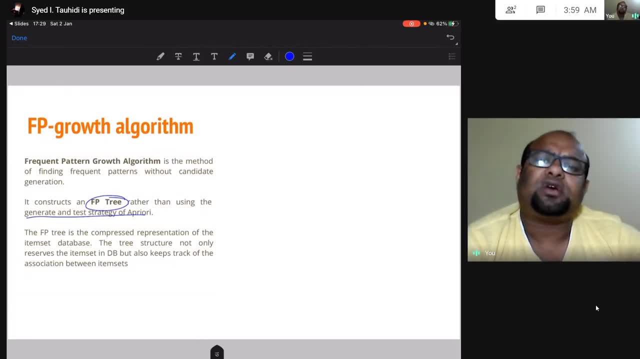 to do. we will have a tree. the tree is going to be a compressed representation. the tree is going to contain all this information already. that is one big advantage. the tree structure not only reserves the item set in uh the database, but also keep tracks of the association between uh these item. 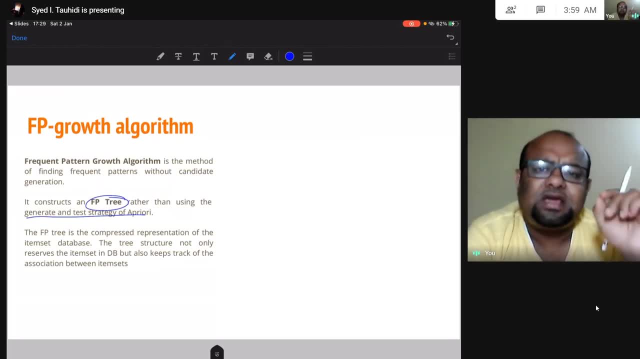 sets. all right, so yeah, we are going to create a tree and we are going to use this tree to generate association rules in fp growth. so let us look at a data set and let us apply a p growth algorithm on that data set in order to find frequent item sets. this is the data set that we will be working. 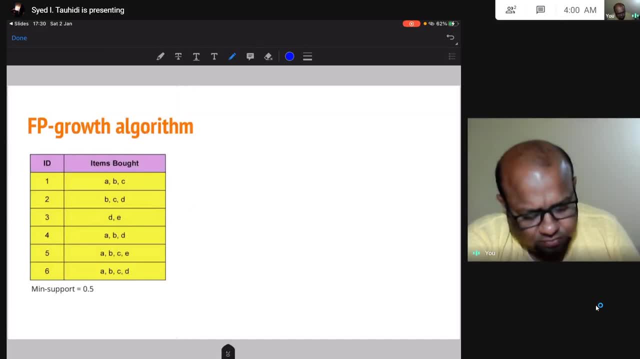 with uh. the mean support we have decided is going to be 0.5, so 50 is going to be the mean support and since there are six transactions in my data set, uh, 50 of six is equal to three, so mean support count is going to be three. all right, now i have five items in my data set. my item set is equal to: 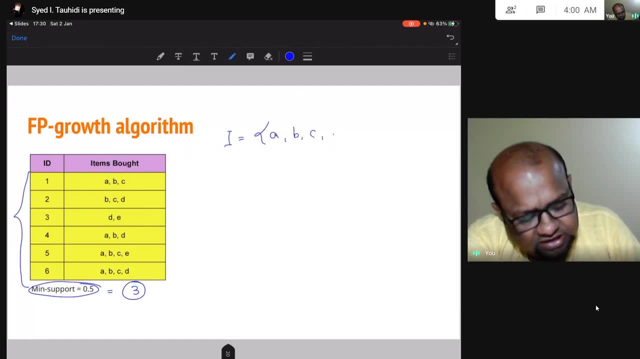 a, b, c, d, e. these are the all the items that are available in my shop. all right now, the first thing that i have to do is i have to create a table with this item set and find the support of each item, the support count of each item. so let us go ahead and do that, all right? so this is the 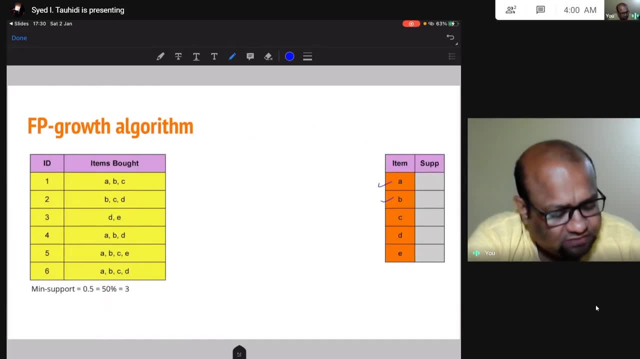 table that we have created. i have all the items over here, all these five items that were there in my item set. let me go ahead and calculate the support of a. so a occurs here, here, here and here. so a occurs four times in my uh data set in my. 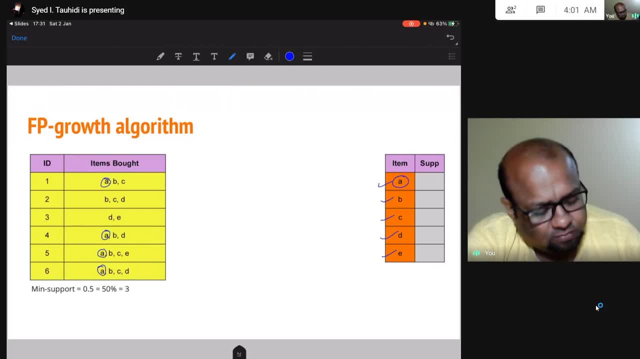 set of transaction. so my support is going to be support count is going to be four. b occurs here, here, here, here and okay, not here. this is not b, this is d and here- okay. so b is occurring five times and in this way i am going to count how many times each of the item is occurring in my data set. 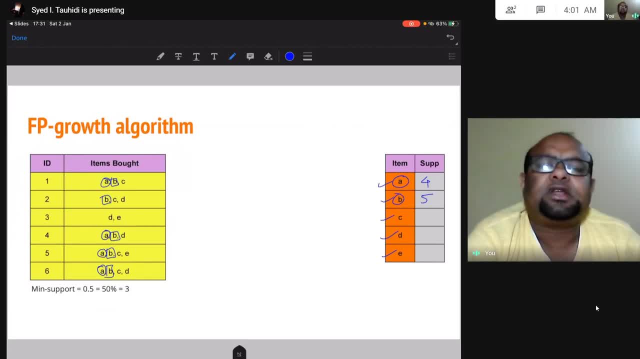 and after counting, i will be filling up this table. so let's go ahead and complete this table. and this is the count that i got. but next, what i'm going to do is i'm going to see what are the counts of each of the item. this is the count of four, this is the count of five, four and four respectively, and then i see: 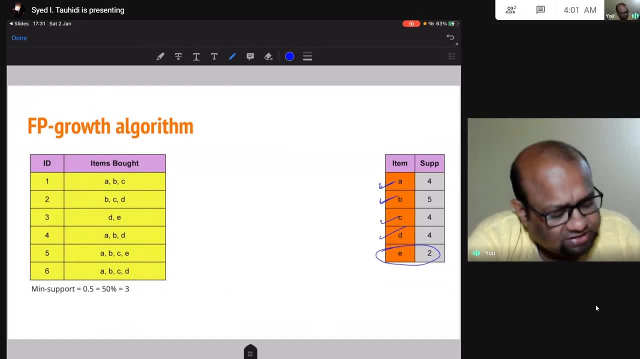 that e has a count of two. all right now, each count is: uh, each support count is less than the mean support that you have taken. mean support was fifty percent, which was equal to three, but he is a support count of two. therefore, i am going to remove e. okay, i am not going to take e any more. 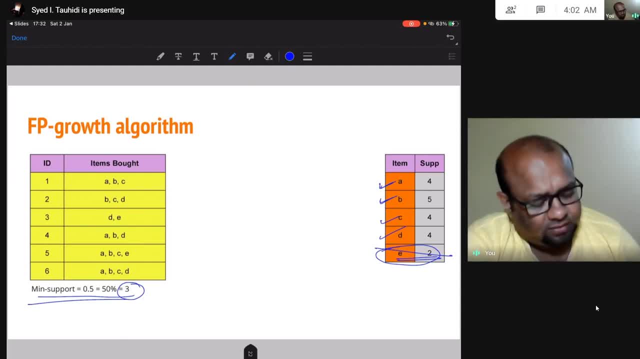 in my calculation. so let's go ahead and do that. i have removed e from my data set. going to remove. i have crossed out e. at least that is something that i have done. next, what i am going to do is i am going to sort this table in a descending manner. 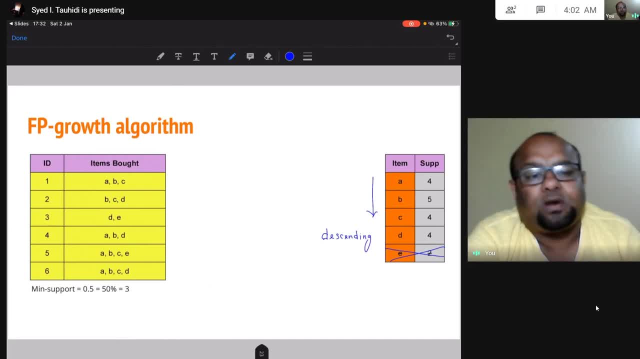 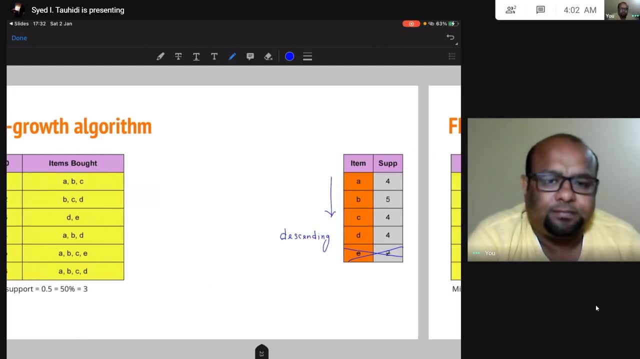 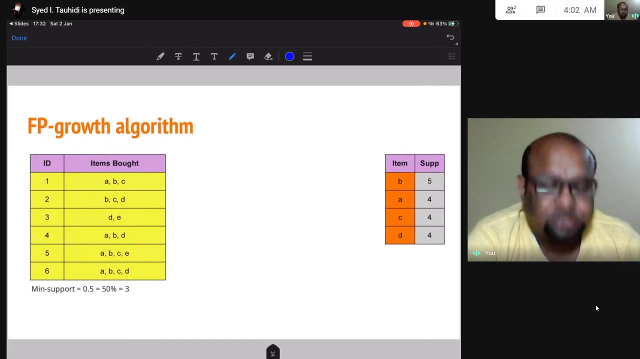 all right, uh, using this support count, right, based on this support count, i am going to do the sorting of this table. so let's go ahead and do that. i have done the sorting. okay, this is the sorted table. now you may uh have this uh question. this is one sorted order. that is fine. first, i have 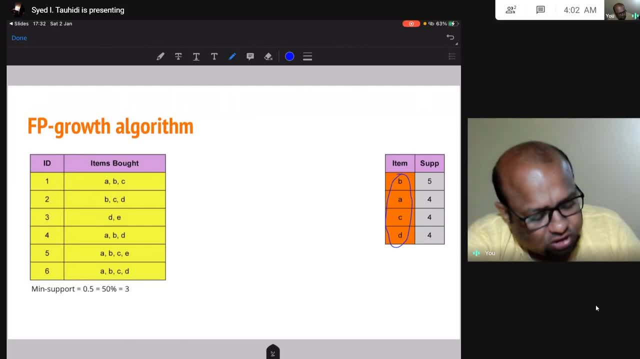 b, then a, then c and d, but this is also sorted right. b, c, a, d- this is also sorted. b has a, a support of 5c, a and d. all of them have support of 4. all right, so this is also sorted now. uh, why do i? 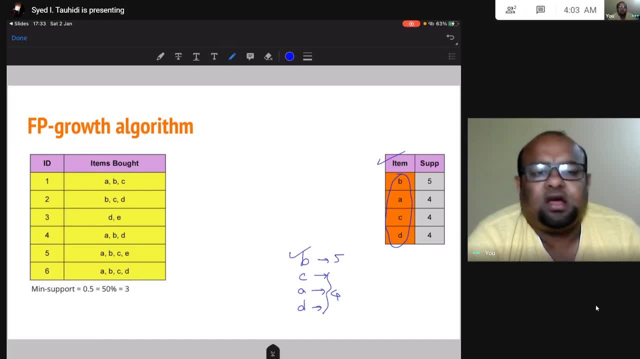 prefer this over this? why should i prefer this or this? there is no reason. you can as well choose this order, all right. but here is the thing: once you have chosen an order, whether you choose this to be a sorted order or this to be a sorted order, whichever order you choose, you have to stick to it. 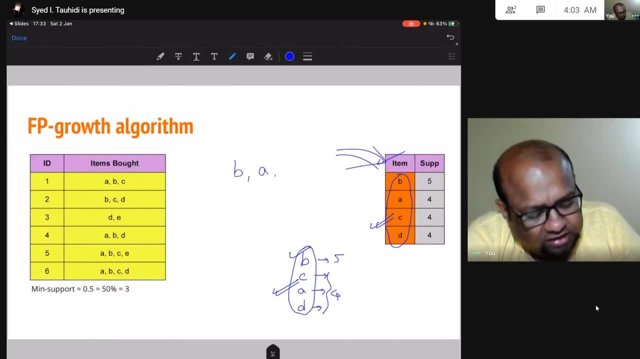 Alright, so I am going to stick to B, A, C, D. This is the order in which I have sorted my items And, till the end of my algorithm, I am going to stick to this order. Now, I am not going to do this. 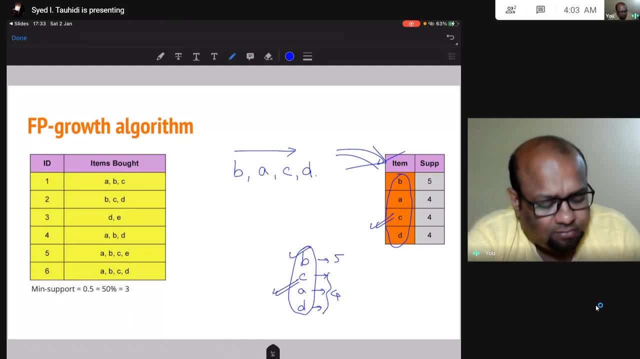 So, somewhat in the middle of my algorithm, I am not going to change my order. Say, for some time I am using this order and some other point of time somewhere in the middle I start using this order. That is something that I cannot do. 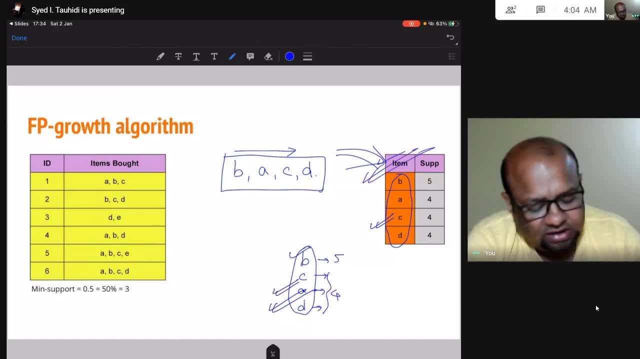 Alright, once I have chosen an order, I have chosen this order, this order, this is the same order, the both of them. Once I have chosen an order, I have to stick to that order till the end of my algorithm, Till I finish running this algorithm. So this is the order that I have chosen. Now what I have to do is all these things that are there in my data set, all these transactions that are there in my data set. I have to reorder them according to this order. 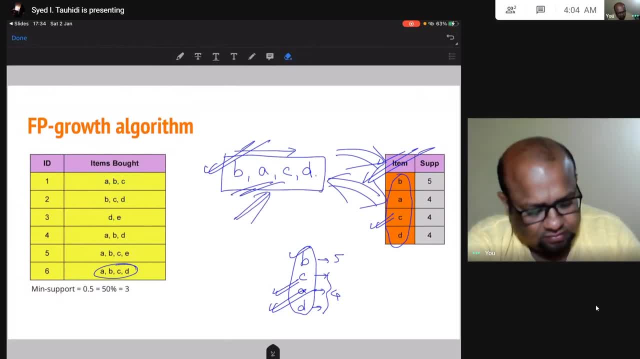 Alright, for example, there is A B C over here, Okay, but here, according to this order, I have to reorder them. So, according to this order, B should come before A and C should come after A. Alright, so I am going to do that. Instead of writing A B C, I am going to write B A C, because this is the order that is given to me by the sorted order, the order that I have decided. 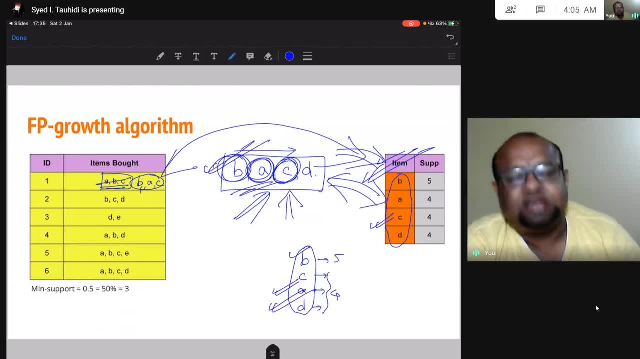 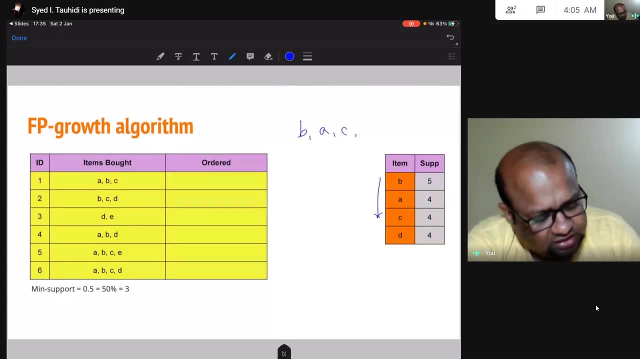 Alright, so let's go ahead and do that. Let's order each of these transactions. The order that I have chosen is B A C D, So B A C D. That is the order in which I have sorted my items. Now let us go ahead and order my transaction according to this order. 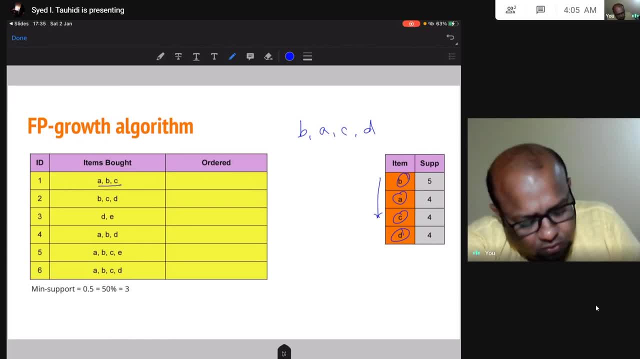 Alright, so here A, B, C will be ordered to B A C. B C D will be ordered to B C D. This was ordered D. E will be ordered to. this is interesting E. I am no longer considering right E. I have removed. E was purchased very few times. 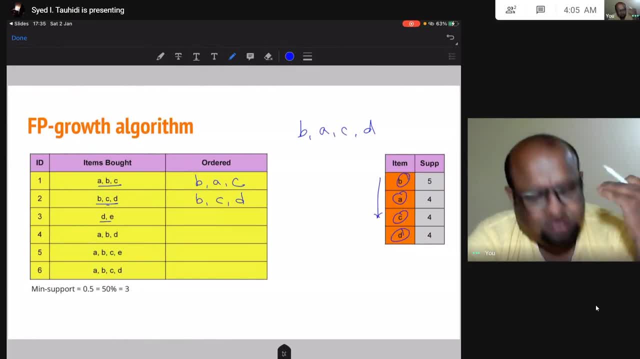 E I have removed. E was purchased very few times, A few number of times, So I cannot- I believe that I cannot- get any meaningful idea of the buying pattern of people who buys this item. This item is rarely purchased, So no point trying to find the pattern in which people buy this item. 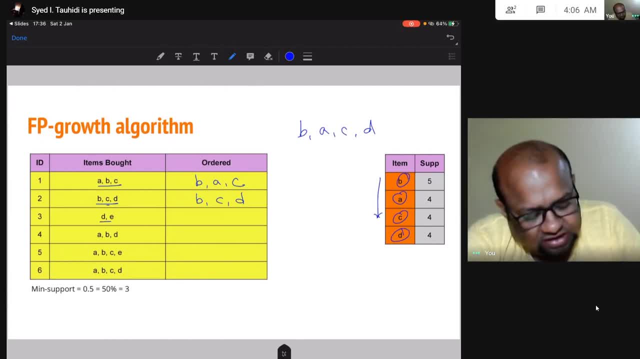 Alright, so E I am not going to consider. D is the only item that I am going to consider in this transaction, In this transaction. Alright, fine, Let's move ahead In this transaction. I have A, B, D. I have to order according to this, So first will be B, then A and then D. 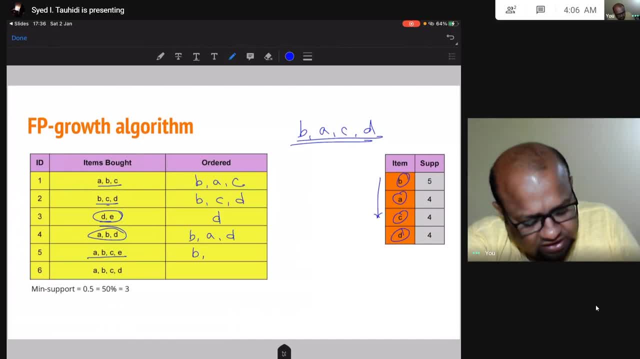 Then this I have to order: First will be B, then A, then C and E. I do not consider. Alright, we already talked about this, So E I am not going to consider. Then I have A, B, C, D. So first will be B, then A, then C, then D. 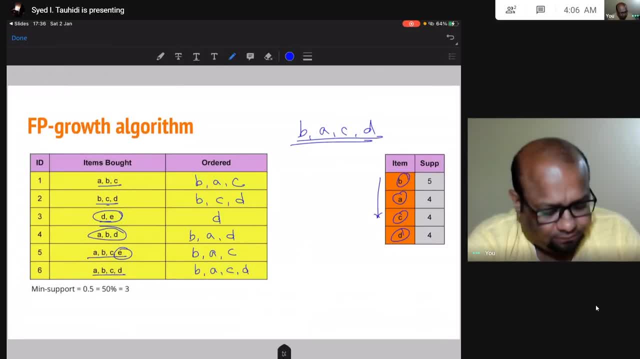 Right, This is the order that we have. Okay, fine, We have done ordering. Now we are ready to create a tree. This is the order in which we had ordered all this transaction. This was our original set of data set of transaction. 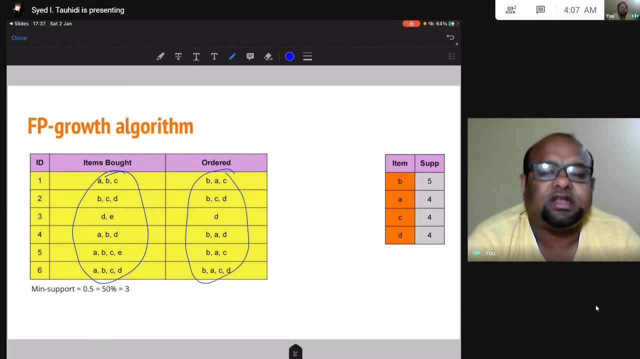 This is our new order set of data set of transaction, And we have removed the items whose support count is less than our, our threshold, our mean support, Alright, so we have done this. Next let us create the tree. Okay, 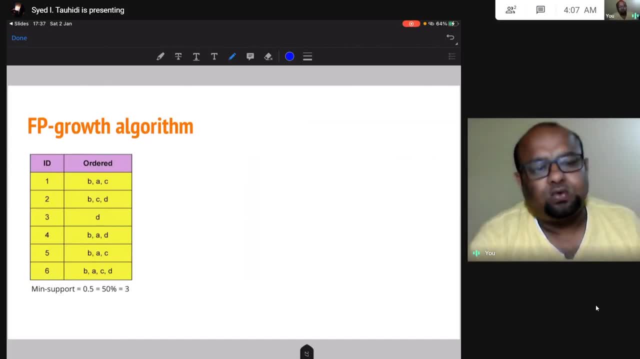 First thing first. Our root node in fp tree is always going to be null. Root node is not going to contain anything. Okay, You will understand the reason, the semantic of this very soon, But let's go ahead And work right now. 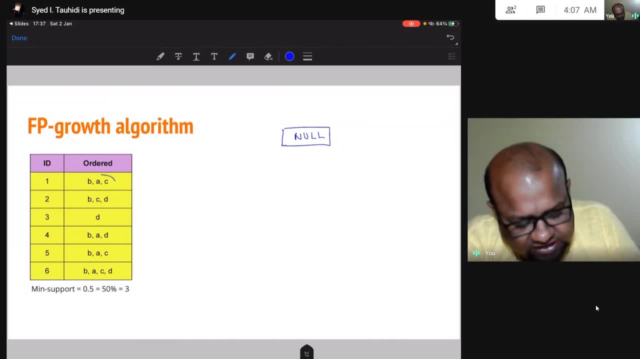 Work on creating this tree. The first transaction I am going to enter into this tree. First transaction contain B, A, C, And what I am going to do is I am going to insert each of this item into the tree, one by one. 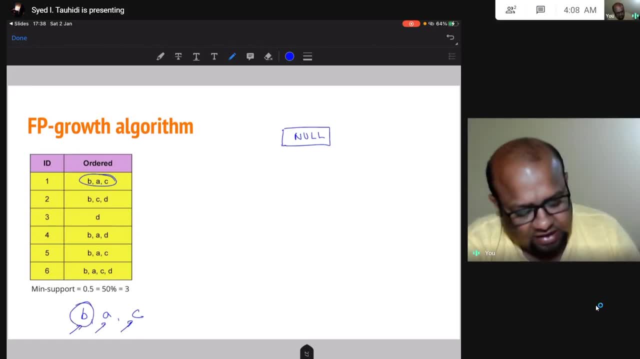 First I am going to insert B. Okay, So is there a child of this root node containing B? There is no child of root node at all, Right, So there is no question of a child node containing B. So let's go ahead and create this child node of B. 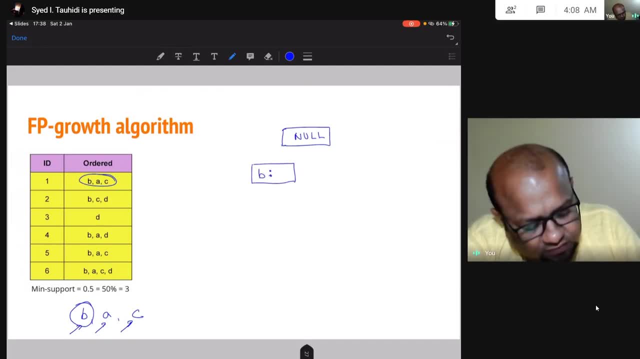 With B, This will be the child of the root node. Now, this is the first time that I am reaching this node. Okay, Therefore the count. how many times did I reach here? Only once. Okay, Now I have done, inserting B into my tree. 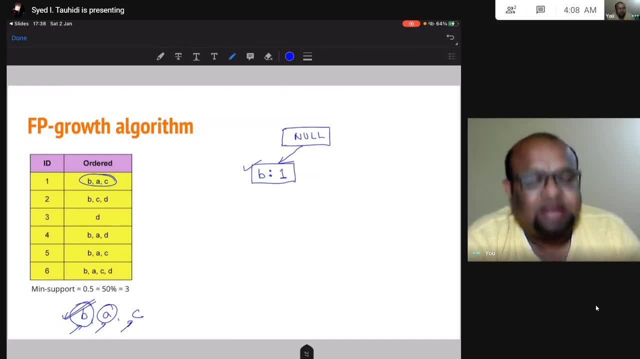 Next, I am going to insert A- Okay, And A comes after B, So A's parent will be B, Okay, So I am going to create A over here. B does not have a child called A, Therefore I am creating this node. 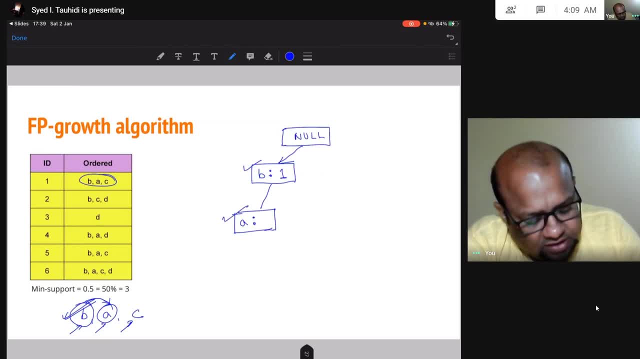 Okay, I am reaching this node for the first time. I am going to write 1 over here. Then I have to create this node C. Is there a node C that C's parent will be A? Is there a node C? Does this A have a child with level C? 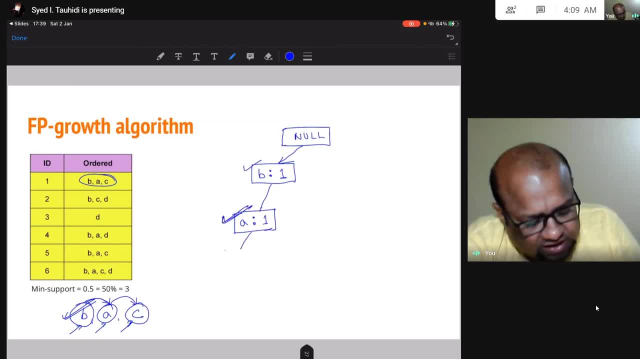 It does not. Therefore, I am going to create a node C, And I am reaching this for the first time. Done, So B A, C, I have entered into my tree. Fine, Next, let me go ahead and enter the next item. 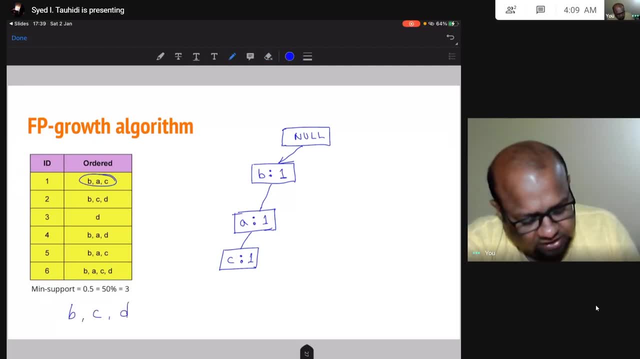 Next item is B, C, D. D's parent will be C, C's parent will be B And B's parent will be NULL. Okay, So let's start with NULL. Does NULL have a child with level B? Yes, NULL has a child with level B. 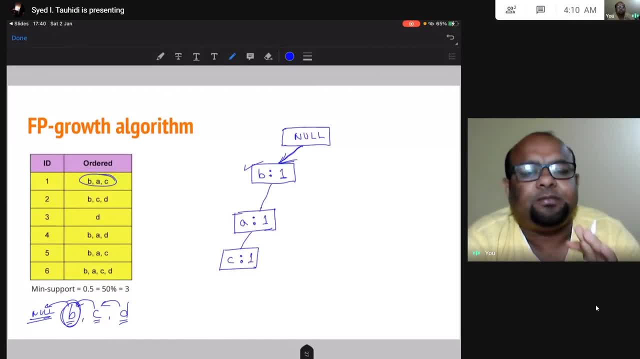 So I reach here. I am reaching this again. Okay, I had reached this once before, So that is what this count represented. I am reaching here again, So I am going to increment this count by 1.. So let's go ahead and do that. 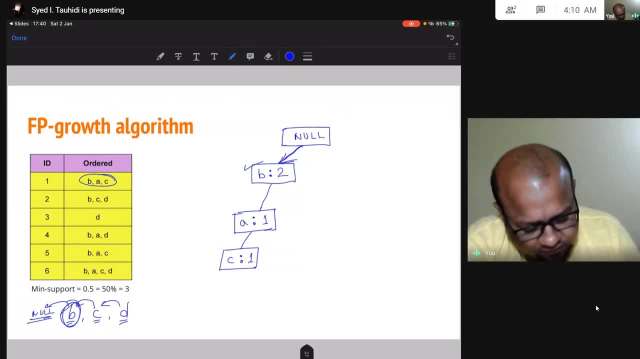 This is now 2.. Okay, Done, I have handled this B. Now I need to handle this C. So is there a C that is a child of B? There is a C over here that is a child of A And A is a child of B. 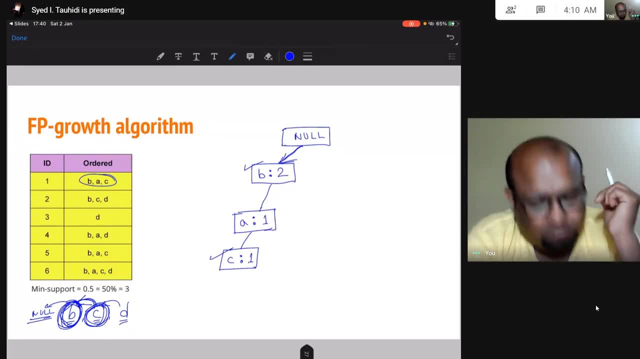 But I want a C that is a child of this B, But B does not have a child called C, Right? So I am going to go ahead and create this child C And I am reaching this node for the first time. Now I have to enter this D. 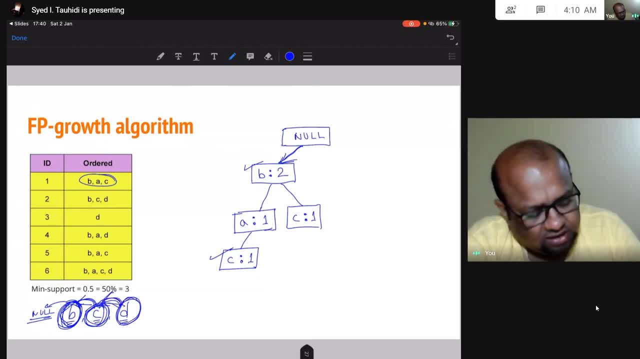 And this D's parent is C. Okay, So this C's child. I am going to have a D over here And I am reaching this as well for the first time. I am done handling this. Now I am going to insert this D. 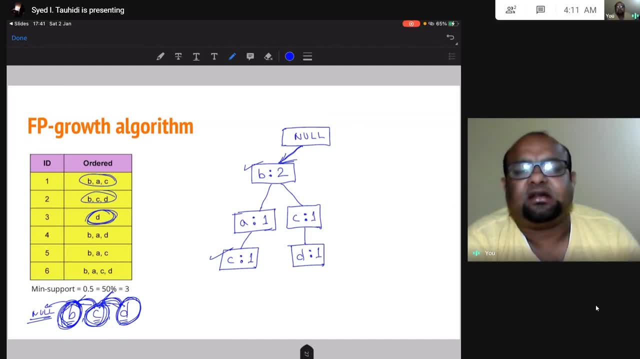 Okay, This D's parent is NULL. Okay, So is there? does NULL have a child with the level D? No, it does not. So I am going to go ahead and create a child of NULL with level D, And I am reaching this node for the first time. 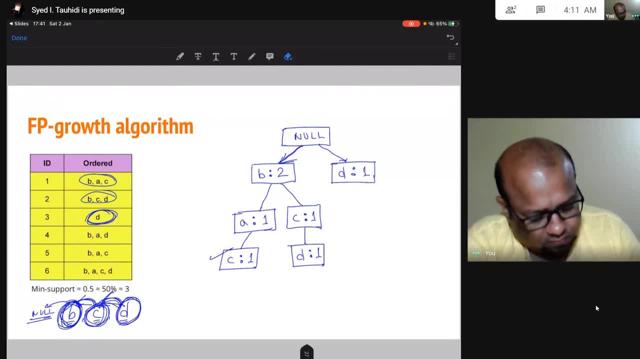 Okay, So I am going to put 1 over there. Okay, And I am reaching this G, Right, This is done, handling this. Then I am going to insert this B AD. So let's go ahead and do that. I am going to insert B, then A and then D. 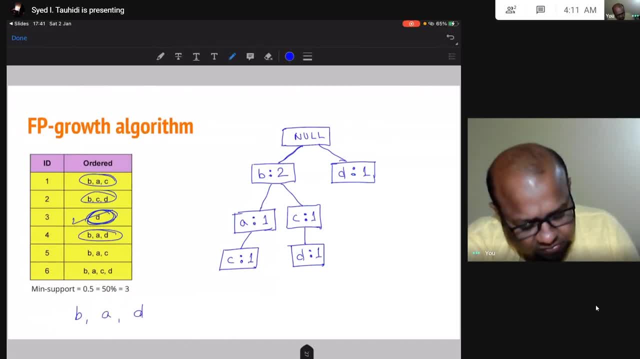 B's parent will be NULL. Okay, So B's parent is NULL, A's parent will be B and D's parent will be A. Does NULL have a child called B? Yes, NULL has a child called B, So I am going to put this NULL over here and insert this child over here. 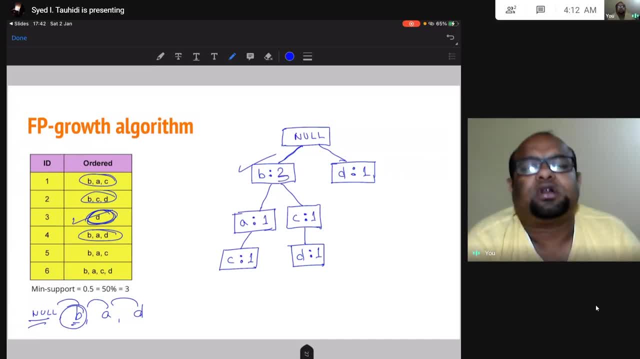 B. So I am going to increment the count that we had associated with this node. I am reaching this again. I am reaching this node for the third time. Then, does B have a child called A? Yes, B has a child called A. Now I have reached here. I am reaching this for the second. 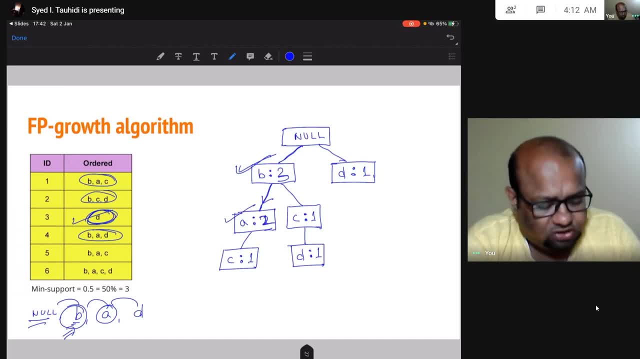 time. I increment this from 1 to 2.. So you may have guessed, this number keeps track of how many times I have reached this node. Alright, Next, let us insert D. So does A. this A. I was here, This is the parent. So this D I have to insert now And this parent will. 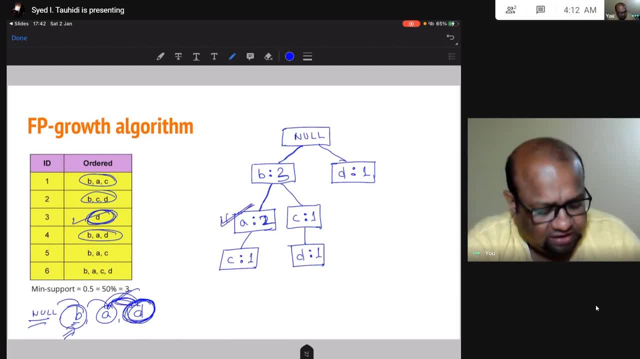 be A, So does A have a child called D? It does not, So let us go ahead and create this child. And I am reaching This for the first time. Fine, This is what I have. Then let me insert this: B A, C. 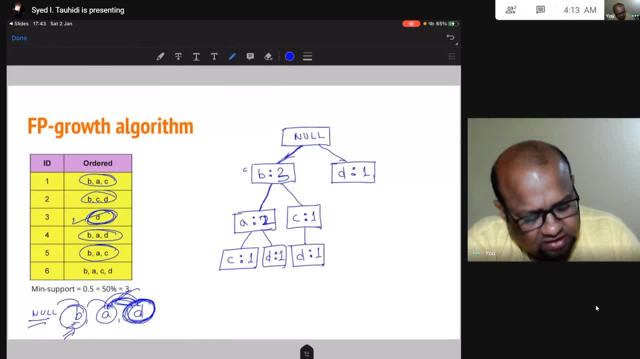 So first I will go here to this B: I have to increment. I am reaching this for the fourth time. I am incrementing this. Then I have to reach this A. I am reaching this for the third time. Let me increment this. Then I am reaching this C, And so from 1, this will 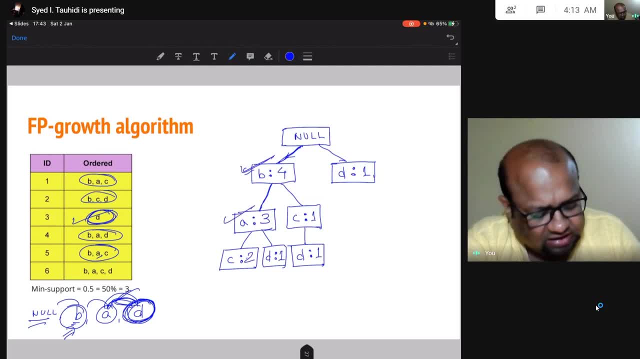 be 2.. So I have reached B, Then A, Then C, And once I have reached a node, I have incremented the count. Okay, Now let me handle this. B, A, C, D, So first I have to insert B. B's parent is nobody. 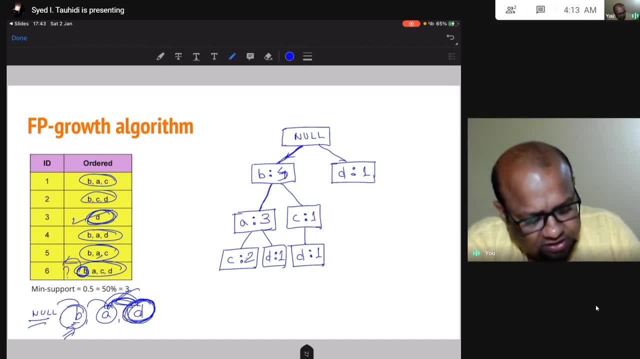 So null. So I have reached here. I am incrementing this count to 5.. Then A A's parent has to be B, So B b has a child called a. so i'm incrementing this to four. then c c's parent is a. so from two i'm. 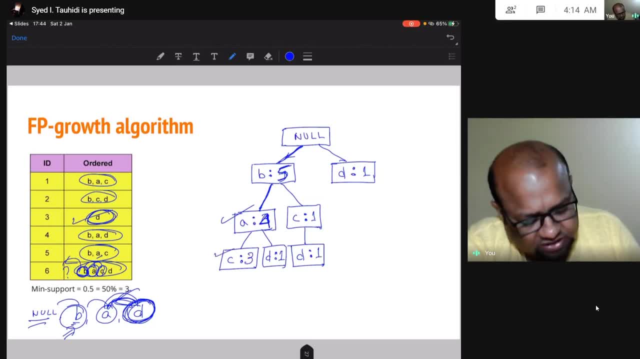 going to increment the count to three. i've reached here, and then i need to reach this node d. this parent is going to be this c, okay, but c does not have a child called d, so i'm making this child d and i have set this count to one. all right, so this is how i have created this string now. 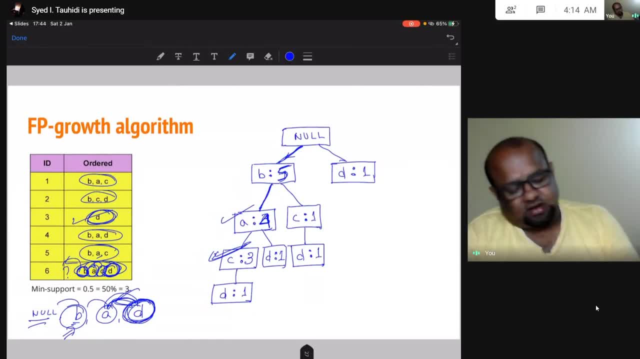 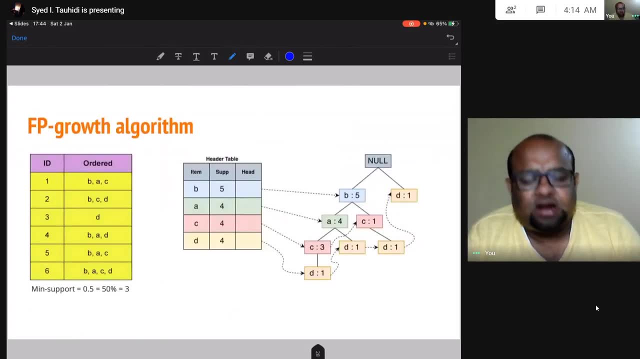 let us look at this string in depth a little bit. so let us look at a proper diagram representing the string. all right, so this is what we have now. uh, all these nodes and edges are same as what we saw in our previous slide that we just drew. but then, apart from 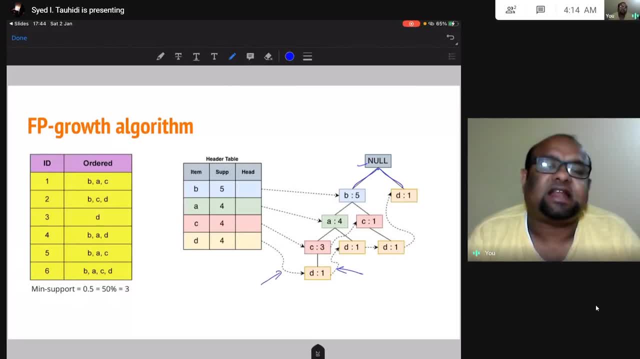 the you may see edges, dashed, edges like this. don't worry about this right now. okay, you will understand what these are very soon, but let's look at the tree and this table. this table is called a header table. this contains all the items in the order in which we had sorted them: b, a, c, d. it contains: 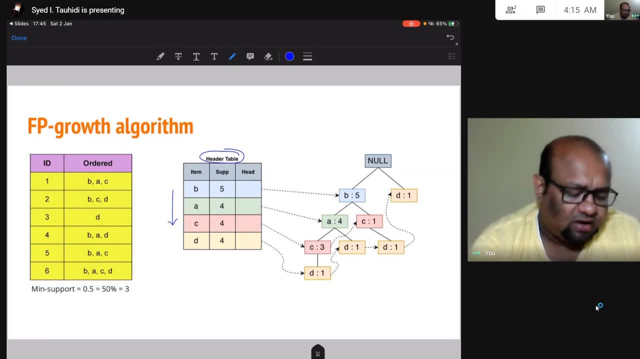 the support. fine, and then we have this tree. now let us understand what this means. okay, if i look at this node right, how am i reaching this node from null? i am reaching b, then from b i am reaching a, and then from a i am reaching c. okay, so b, then a and then c. 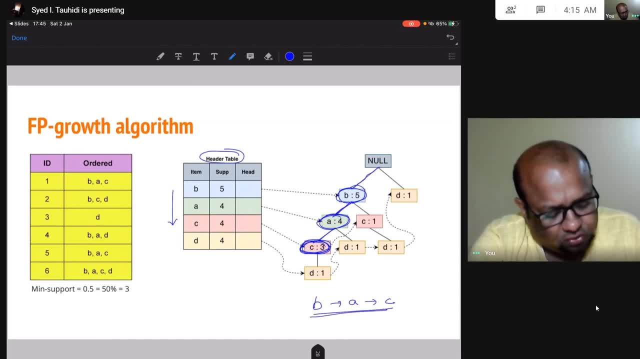 this is the part of the path that i am taking to reach this node right. and what is the count associated with this node three? what does this mean? this means that there are three transactions where a, b and c are purchased together. so this is one transaction. so this is one transaction, and this is one transaction with b, a, c. all right. 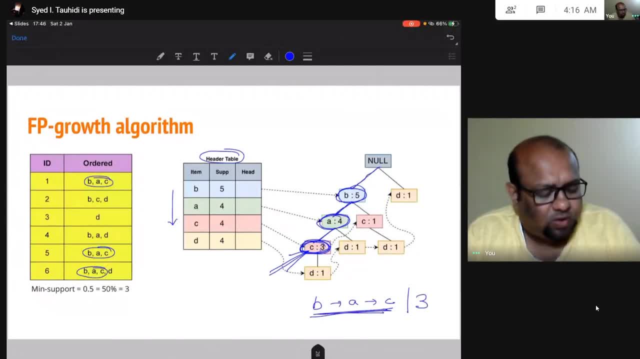 so there are three transactions where b, a and c are purchased together. all right, so that is what this means. now, uh, let us look at what this means. okay, if i look at this node, uh, its parents is b. okay, it has a count of four. that means there are four transactions where b and a are purchased. 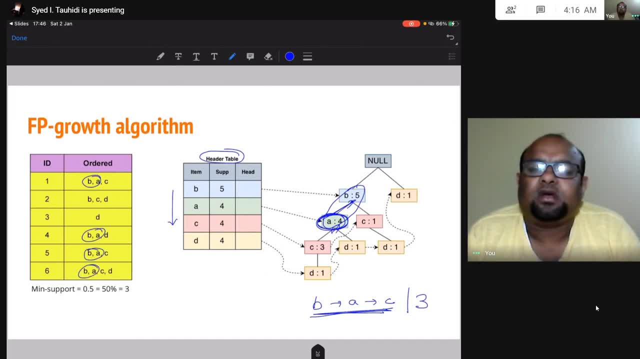 together. okay, so this is one transaction where b and a are purchased together. know, another interesting thing to observe would be this: so this is what that means. this is what concept says. so this is what that means. let's look at a List of demons played by evil spirits. 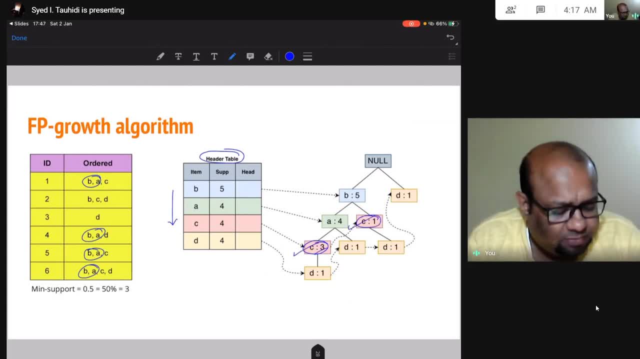 another interesting thing to observe would be this: to observe would be this: so this is a mate, so this is a love text. so if I write up my name, then I should have written three, N, that means, but then first of four of my sex, as this big itself. so this is a c and this is a c. this is a value of three and this is a value of one. three plus one is equal to four and that is the support of c. right, this is D, this is D and this is D. there are four we so, uh, when i add down N, any so 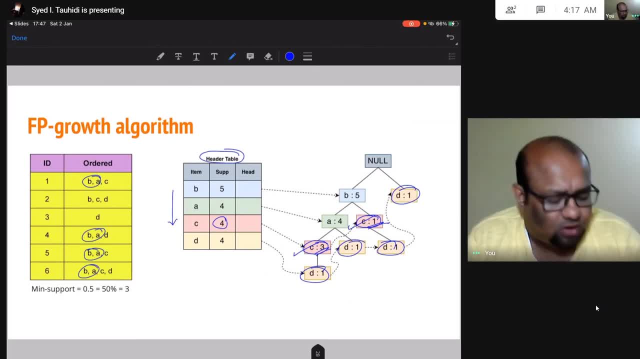 So when I add all of these, all of these four, these have value equal to one, count equal to one. Okay, when I add all of them, I end up with four, which is the support. Similarly, four is over here and five is over here. 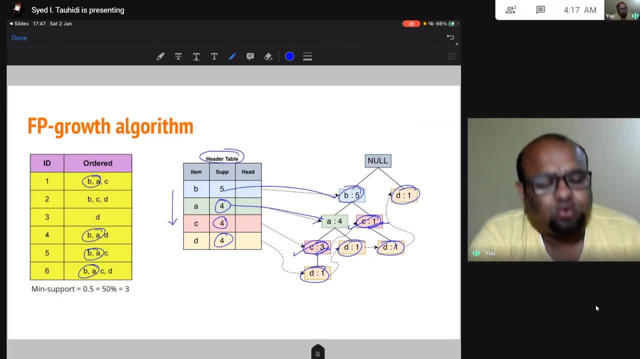 So if I have more than one node representing one item, when I add all of these nodes I will end up with the support All right, when I add up the count to all of these nodes. Okay, now let me repeat what I just said with one more node, 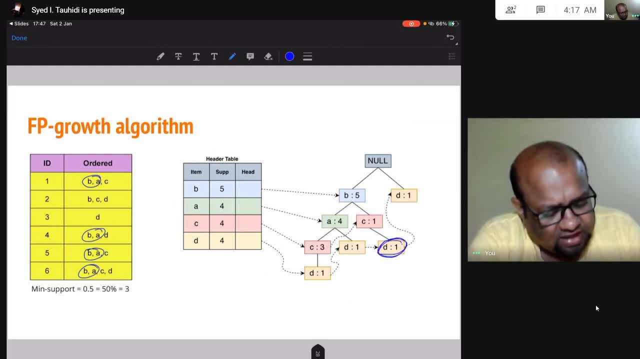 See this D. how did I reach this D? I went from null to B, from B to C and from C to D, So I took B C D. That means what This B C D is purchased together in how many transactions. 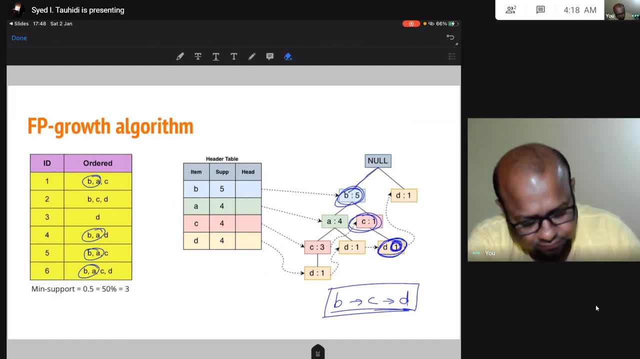 In only one transaction. So B C D is purchased. B C D is purchased together in one transaction. Yeah, B C D is purchased once together in one transaction, but then B C D is purchased here as well. but that is four item frequency. 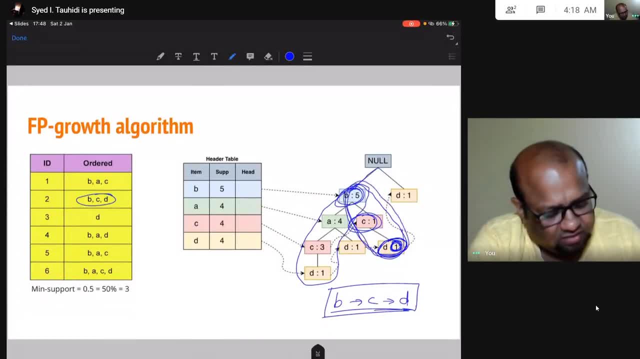 In three item frequency. it is purchased once over here. Okay, so this is what it means. This is how, Now, this three is giving us this information of what are the items that are purchased together and how many times. Now, yeah, this is one thing to observe. 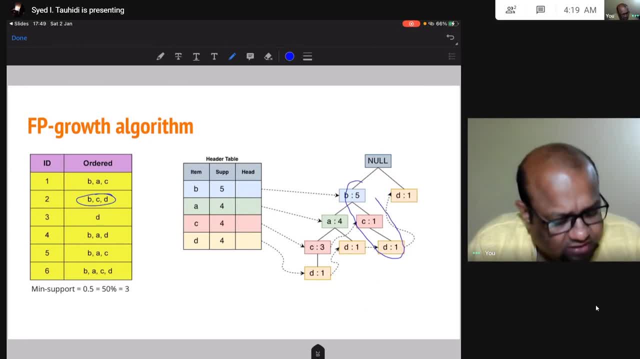 B C D is purchased together once over here. B C D is purchased together once over here. Okay, in this four frequency. So this B C D, the fact that B C D is purchased together in two transactions, 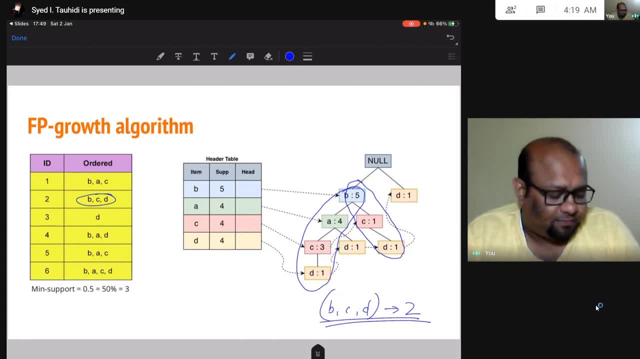 Is not yet recorded properly. Okay, so we have to do that. So let's go ahead and try to compress these different branches into one information: The fact that this transaction is once when B C D is purchased together. The fact that this four transaction contains B C- D purchased together. 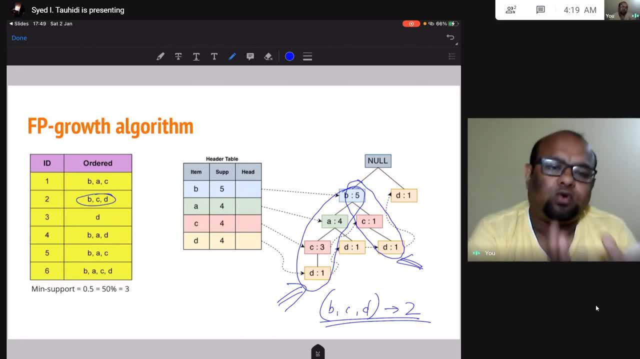 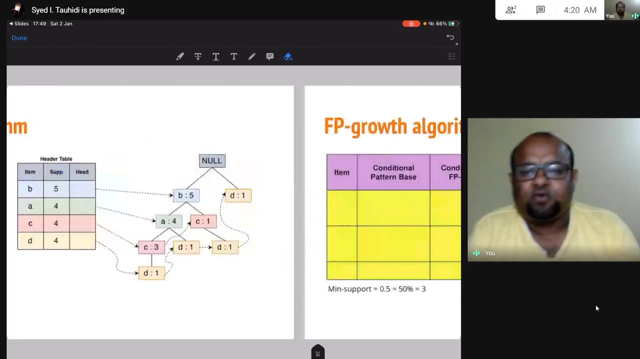 Let's go ahead And work more with this tree and try to find more information from this tree. Okay, and to do that, we have to create a table. Now, this table. there is no name for this table, but there are four headers. 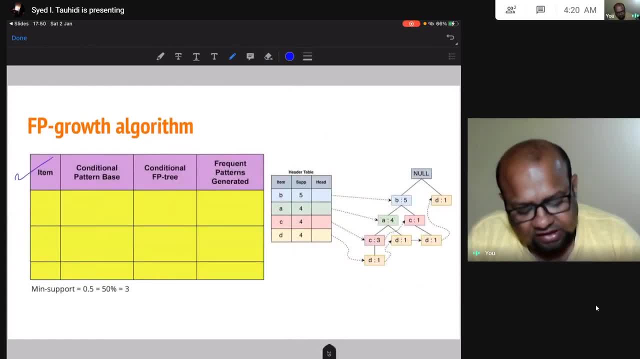 All right, One is the item, Another is conditional pattern base, conditional FPT and frequent pattern generated. So this is our ultimate aim. This, Again, item sets that we have to generate. Okay, along with the support of this frequent item set. 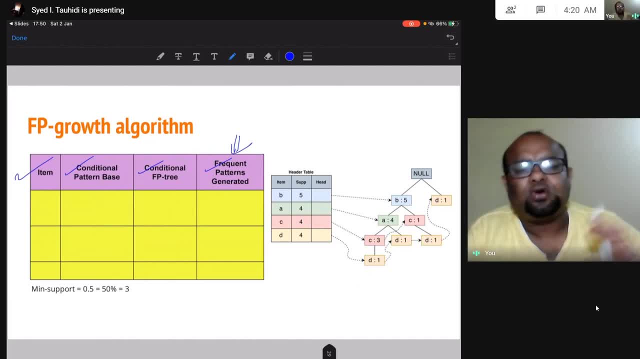 So let's go ahead and handle one column at a time. All right, The first column that we have is the items, So we have to fill this first column. And the way to fill this first column is simple. We had sorted in this order: descending order. 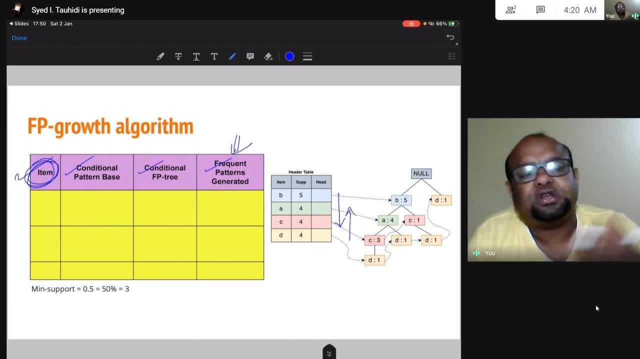 We have to fill this column in the ascending order, in the opposite order of in which we had sorted our order list. we had an order. we have to now fill the items in the opposite order, all right, so first thing will be d, then there will be c, then there will be a. 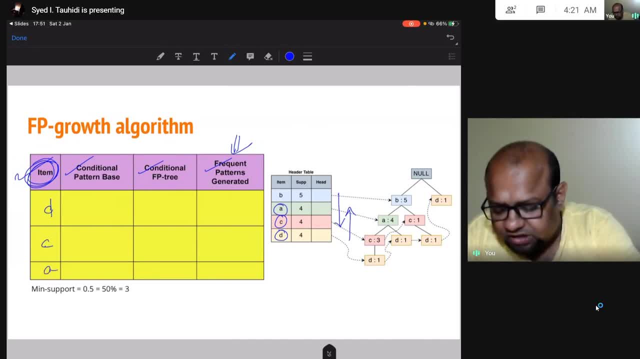 d. okay, done. next we have to find the conditional pattern basis. this means this d. there are several d's. okay, how did we reach this d? or for this c: this is a c and this is a c. how did we reach this c, this a, how did we reach this a? and how many times did we reach this a using this path? that? 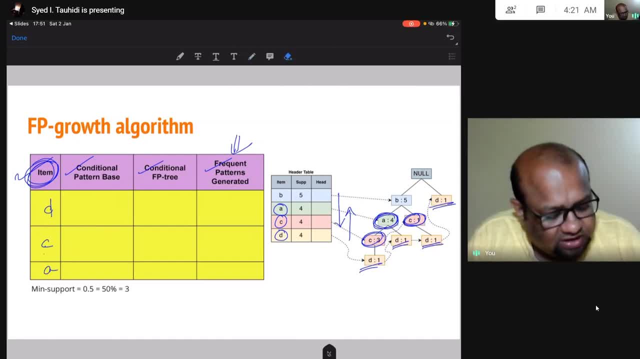 is something that we have to find. okay, so let's go ahead and find it. uh, i should find b first. sorry, i should find d first, then i should feel c, then a, but i am going to do it in the opposite, uh, manner. right, there is no reason, just for the sake of. 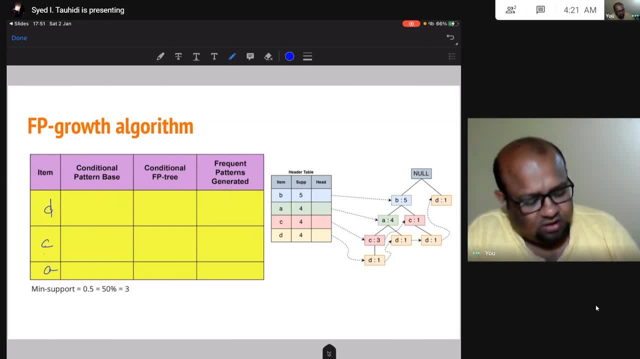 this class. i am going to fill it in the opposite order. all right, so a, how did i reach a? i came from null to b and then b to a right, so i came from null. i don't need to write null because every path will start from null, so writing null. 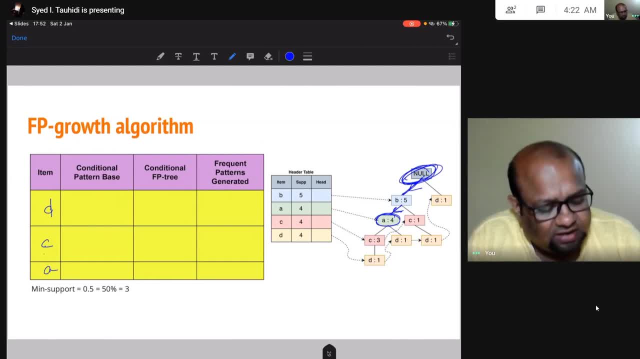 does not give me any information. not going to write that. so I got from B and then I reached a, a also I do not need to write because I am trying to find what is the path that leads me to a. so every path we end with a. okay, so I don't need. 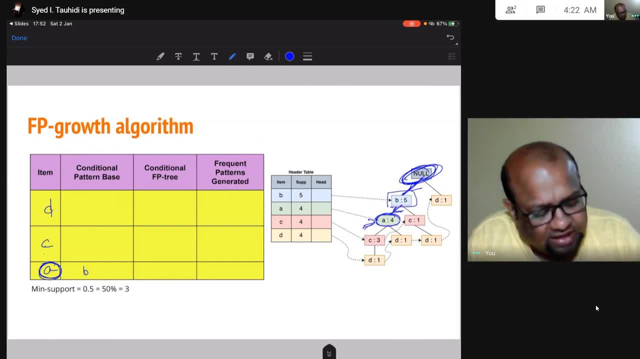 to write a at the end. I simply write this B, and that is enough information. okay, now, how many times did I take this path? how many items are there? when B and A are got together, four transactions are there. okay, so I require that as well. now let's work for C. okay, this was too easy. and because this is too easy, so it might. 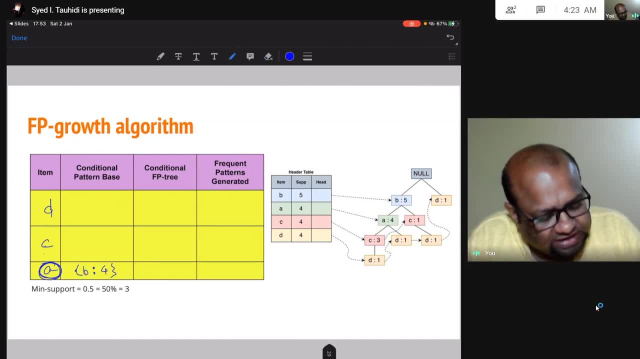 be too confusing, so let's work with C. so there are, 望мiken, two paths that lead me to c. okay, one is this path that goes from b to a to c, and one is this path that goes from b to c. all right, so let us write both of this path. so the first path is b, a and c. 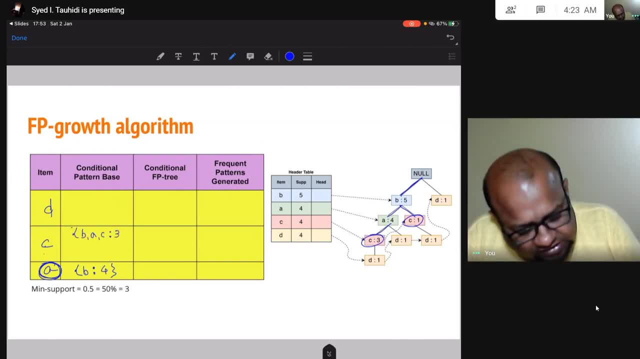 and that has a count of three. second path is b, c, and that has a count of three. okay, i did not write a over here. in the same way i should not write c over here. why? because c is anyway going to be the end node. i am trying to find paths that lead me to c, so end node is anyway going to be c. 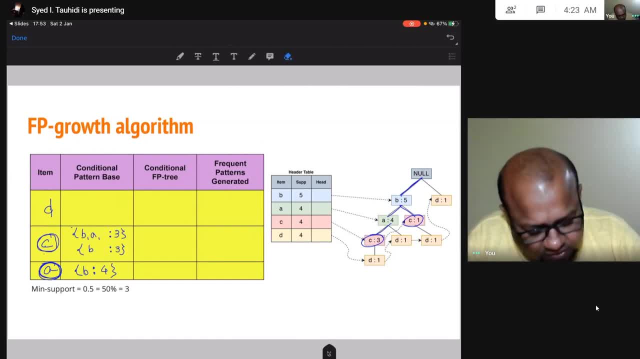 therefore, i am not going to write this c, all right. so this is sufficient information. how am i reaching this c, this b, a from this b? i can write c over here. i go to a and then i reach c. how many times am i taking this path? i am taking this path. 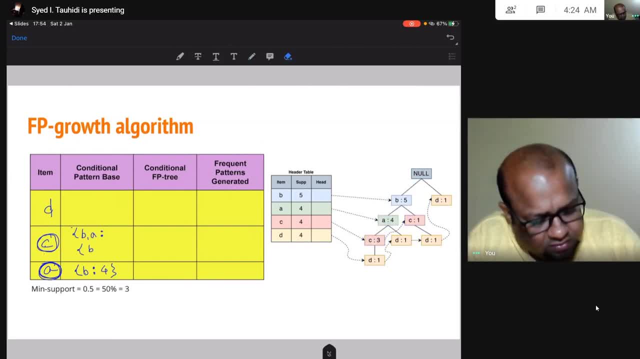 three times, right, so three. then i am taking this path from b to c. how many times am i taking this path? one time, okay, done. next, let me work with d. okay, so there is this d. i take this path b to a to c, so b to a to c. how many times did i take this path? only once. 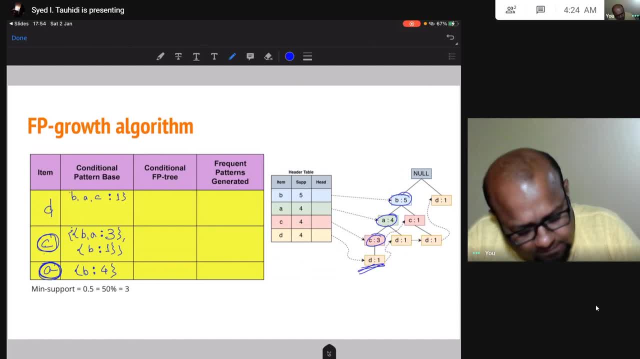 fine, then i have this: how many times did i take this path: b to a to d, this b to a and then d? i have taken this path once as well. then i have this: i have taken b to c and then to d. so b to c and then to d, okay once. and then i have this: 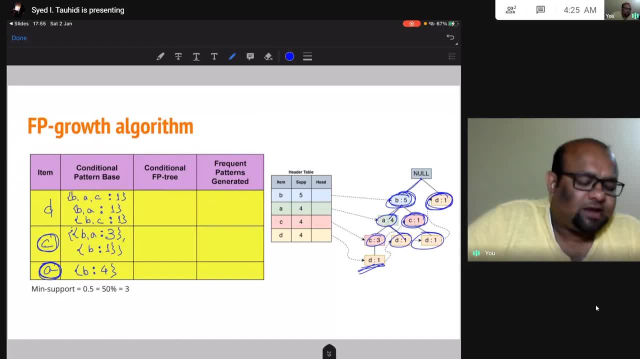 what to do with this. this item was purchased alone, okay, this d does not have any parent, right? so i am not going to write this. all right, so there is no path that takes me to this. this was a single product, okay, so this does not have any dependency on any other product. 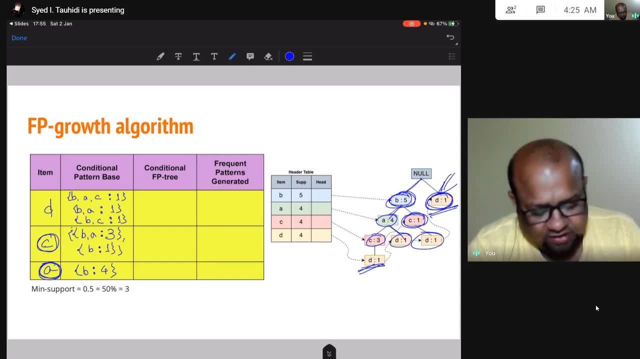 okay, so going to ignore that. and this is how we have drawn, we have written down the conditional base patterns. okay, fine. next we are going to compress this information and write it over here. okay, so the thing that i am going to write is this: okay, how many times is b occurring here? b is occurring here three times. how many times is a is occurring here? not only occurring means. there is something else. 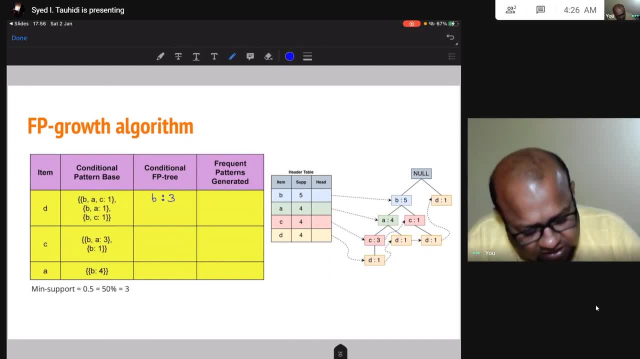 let me do with this as well. how many times is b occurring here? two, okay, but i am not going to write two here. no, this b is occurring three times. right, this b is occurring one time, so this will be four. okay, this b in this path b a c. this b occurred once. in this path b a. this b occurred once. in this path b c. this b occurred once. so in total b occurred three times. all right, but here: 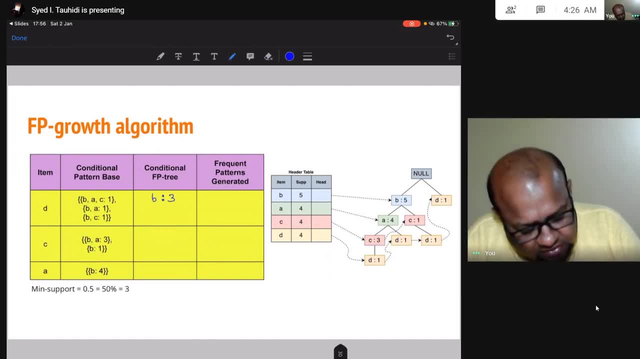 in this path, in this c3 okay in when taking this path b to a to c, how many times did, uh, i take this path? i took this path three times, all right. therefore, i, when taking this path, b, a, c- three times, i saw this b three times, all right, so i saw this b three times. 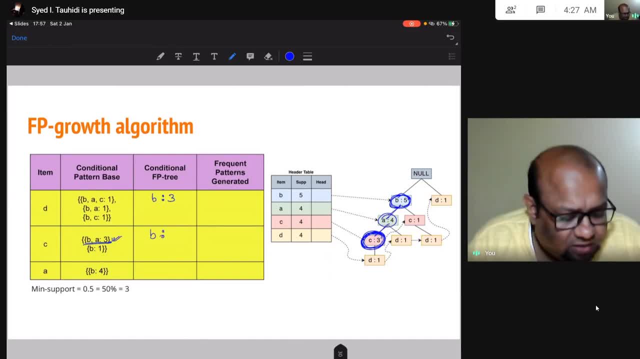 i went through this b five times, three times when going from b a c. one time when going from b a c d, all right. one time when going from b a c d- all right. one time when going from b a c- d. so in total i saw went through these five times. but my question is: 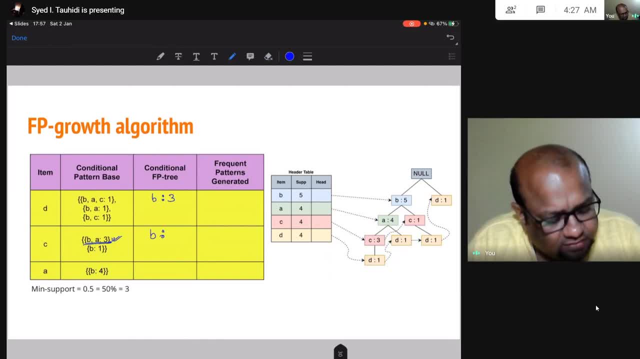 but my question is: when going to this d, two dc. when going to c, i went to c two times. you did the same exact position and you want to be paid, when the problem is that because of this path and this path isから doors are game. when i saw b a c, this path, i took two times. and this path, b a c, d- i took one time. all right, so 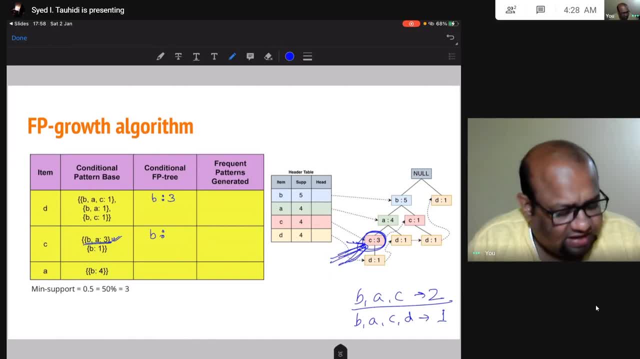 this c when reaching this c, i would reach this c two times when reaching, when, uh, going through this right, and i reached this c one time when going through this. all right, so this is how uh, i have reached this b while reaching this particular c, i saw this b three times. that is what this means. 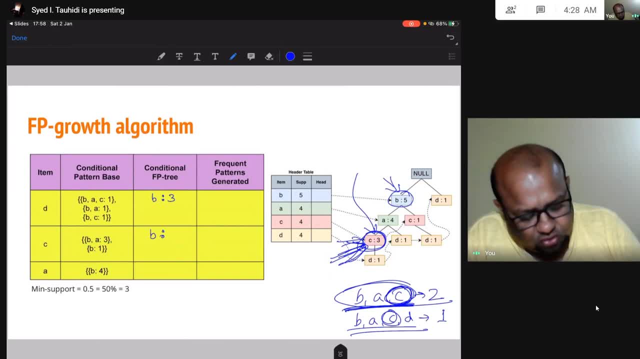 okay, so i, i took this path three times. i took this path one time. okay, what is this one time? there is this. see, i am looking at c, right, i am looking at the other c now talked about this when, uh, looking at this c, i reached this b three times when taking this path. i took this path only once. all right, 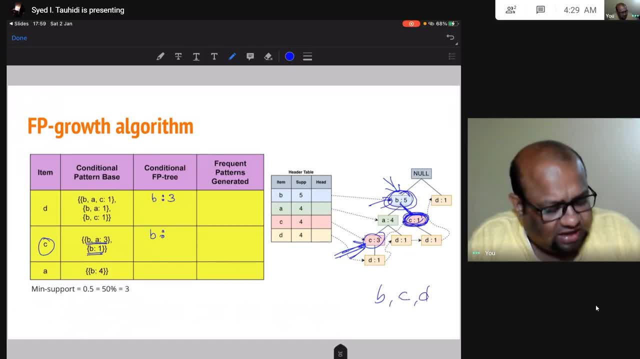 when i was filling b, c, d, i had this transaction i took, i went here, i went here and i went here. okay, when doing this, to reach here, i went through this once. okay, so to reach c, this other c i took went through this b once. when reaching this c, i went through this b three times. 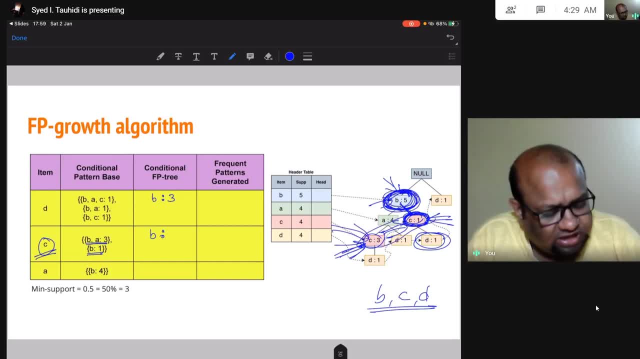 so, in total, i have this two c in total. to go to this two c, how many times did i go through this b? three times when taking this path. one time when taking this path. therefore, in total, four times, and this is what it means. okay, so understand the meaning. now calculation is really. 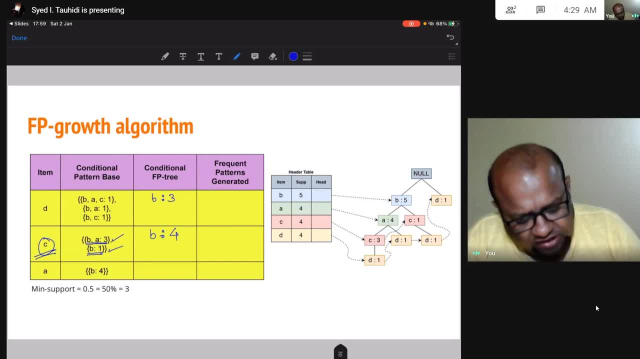 easy, okay, uh. for example, let me calculate for a: a will be one is one plus one, two times occurring here. okay, for c: c is one plus one, two times occurring here. what about a? a is three times over here and none over here, so three here, b is equal to four. you just find out, uh, to fill this for exam, or? 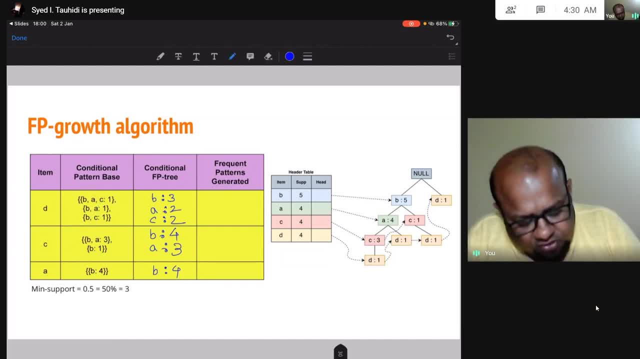 to fill this for your, your program. you just make a count of how many times it is appearing, in how many uh sets it is appearing and what is the count associated with each set. okay, uh. so if i had said x, y, z with four, x y with three and y z equal to two, 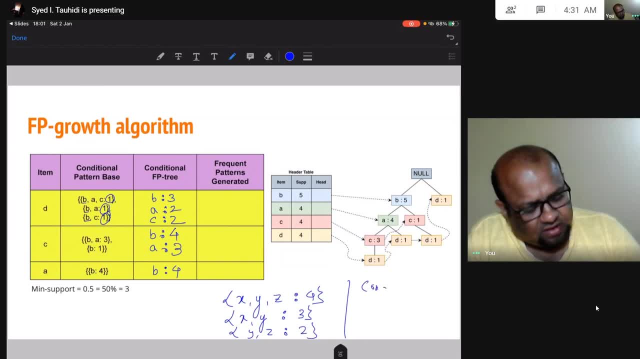 and i find to find conditional fp3 and i want to find for, say, x. okay, what will i do? x is here, x is here, x is not here, right? therefore, i will find for this x, what is this value four? that means i, i would have taken this path four times for this x, what is the value three? so three, therefore x. 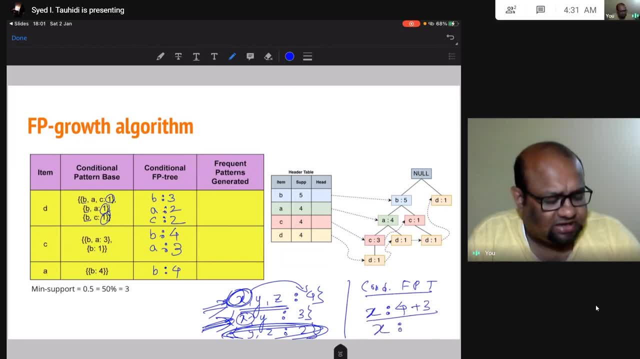 will be x will have the count. how many times do i see this? x will have this count? uh, seven, all right, so this is what we do actually. uh, finding this value. how many times did i see this note? when reaching some note, say: uh, this is to reach some p, okay, so my tree will be from null. 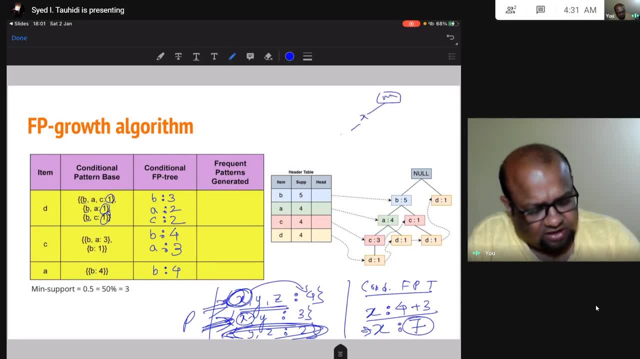 there is x, there is y, there is z and there is p. for this it means there is x, there is sorry, x, y and then p. okay, and then y, z. okay, there will be y, there will be z, there will be p, and this is what the three would look. this is: 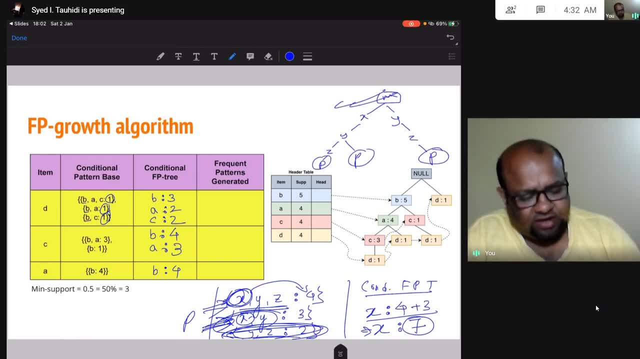 what the p would look like in the tree. there will be other notes. if there is q somewhere over here, it may be there, but at least the p should look like uh in this way. if this is the battery, all right. so point is: how many time am i reaching each of these? 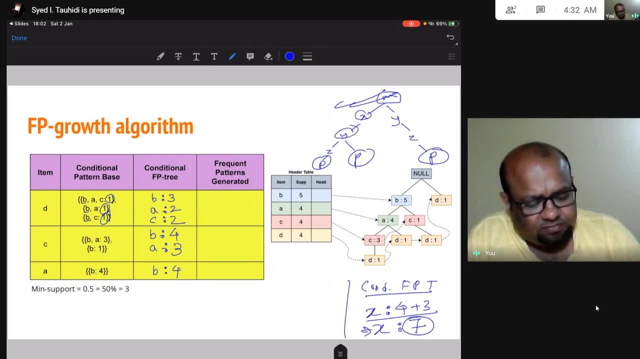 notes when trying to reach p. okay, so this is how we do this calculation: very simple to calculate, but then do understand what this thing is telling us. all right, if you simply calculate and do not understand what this thing is telling us, then, uh, you will not be able to do data analysis properly. you will be able to pass the exam. 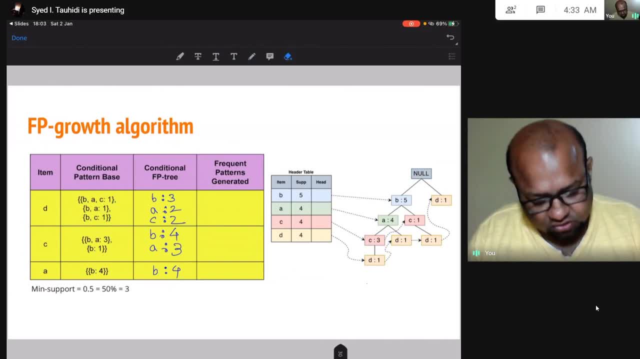 that is not a problem, but my aim here is not to just make you pass exam. aim here is to make you good machine learning expert. all right, so this is what we have now. we have, uh, created this conditional fp tree. okay, now our final thing is to calculate these frequent patterns. 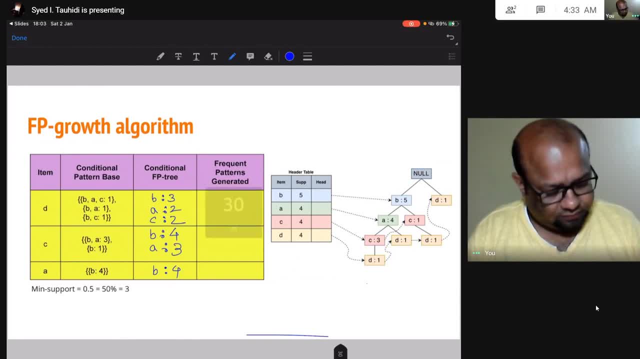 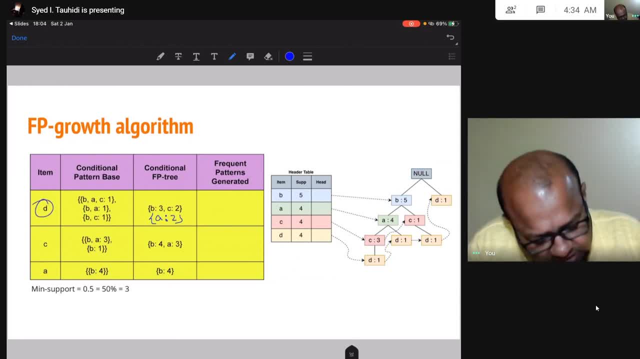 frequent pattern with d, so there will be d, d, b, there will be d, c, there will be d, a. okay, so there will be more. i forgot about a, but then uh, okay, let me once again do from the reverse direction. we will handle this at the very end. 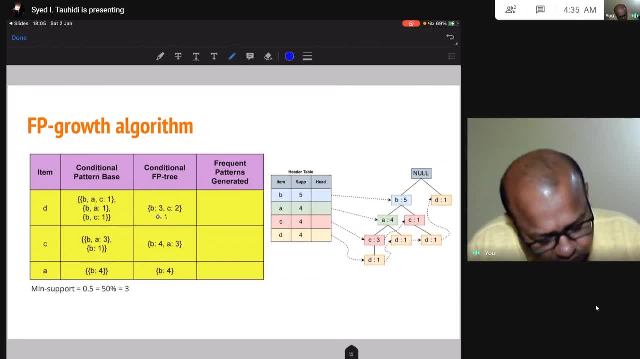 by the mistake, a will be two. okay, the set is not over here because it gets over here. let's start with this. so b, a. okay, i'm making frequent pattern with b and a and this has a support of four. this is what it says. now let me make frequent pattern with b. 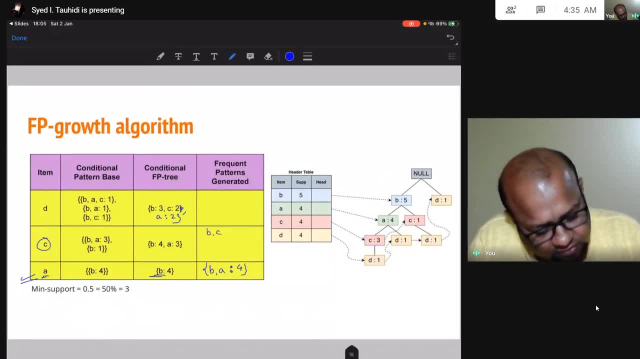 with c. so b- c will be one frequent pattern, b- a will be one frequent pattern and b a- c will be one frequent pattern. let us find support of each of them. okay, how do i find the support? b- c, so b and c will have a support of four. 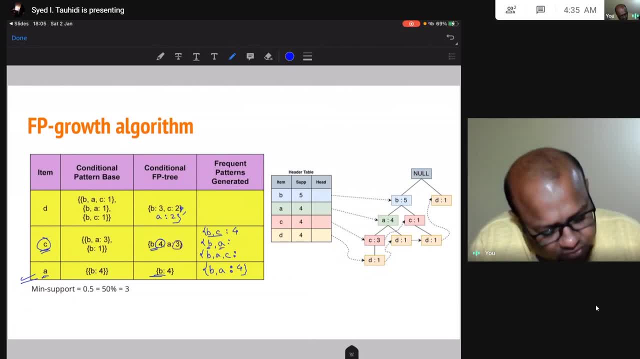 okay, b and a will have a support of three. okay, now, interesting. what is b a c, b a c and b a c, b a c? we have a support of what is the lower among these three, among these two, four and three? uh, the lowest is three. therefore, this will have a support of three. all right, so this is what we have. 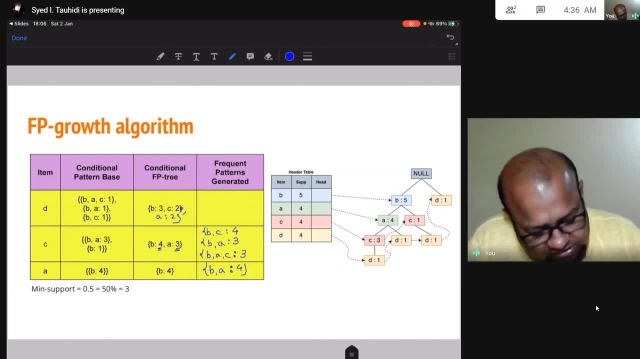 now is: this is not going to be sufficient. i am going to find uh uh pattern with this all. so B D will be one pattern. okay. B C D will be one pattern. A D will be one pattern. what is the support of B D? B D will have a support of 3. what will be the support of C D? 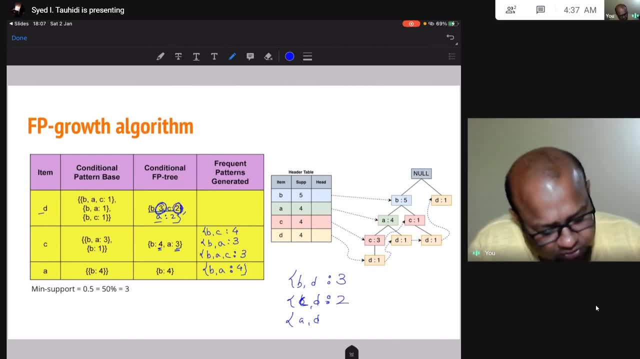 C D will have a support of 2. what will be the support of D A or A? D A, D will have a support of 2. okay, fine, now let's make a pattern with three objects. so that will be D C, D, there will be B A, D and there will be B. 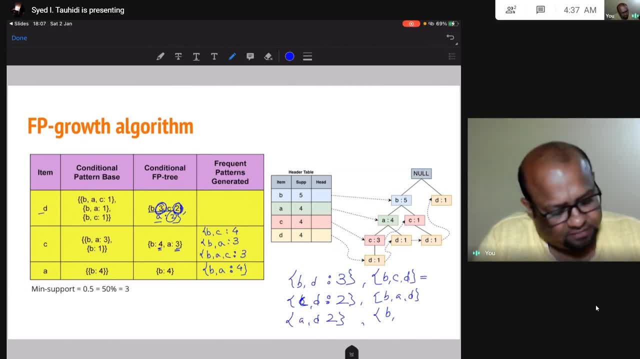 let me show for B C D and B A D. okay, there will be lots of possibilities. let us not do all of them. so B C D, let's go ahead and find that. so B has a support of 2. C has a support of. B has a support of 3. C has a support of 2. 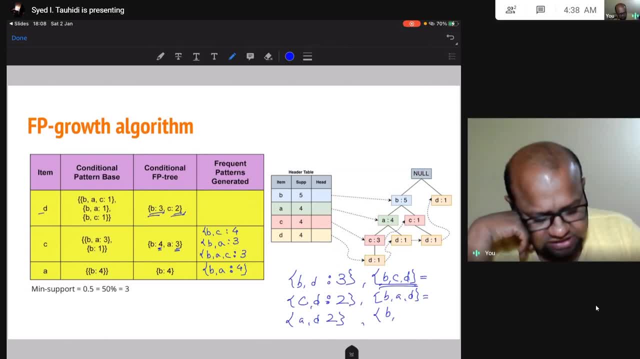 therefore, B C, D will have a support of what is the minimum amount here, 2. alright, so B, B, then C, then D, we will find a support of 2, okay, once through here and once through B C D. taking this path once. taking this path once. alright, so this is how we do this compression. we were looking at how to do this compression, okay. 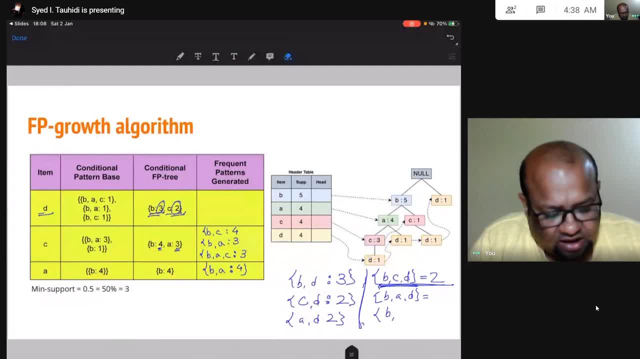 so this fact that I have this B C D once over here and B C D once over here, I want to compress them and make sure that I count this pattern occurring together 2 times. this is how I am counting it: 2 times. alright, so this is what we do. there will be lots of possibilities here, okay. 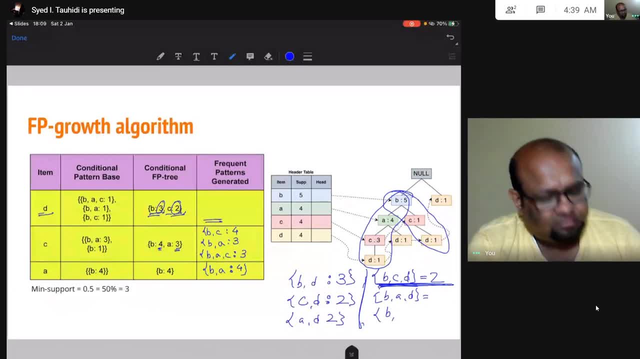 so you have to do this count lots of times. it's at least less than this: the number of possibilities in a priori, far less than the number of possibilities in a priori. this is polynomial, not exponential. alright, but then this is how we do this count. now, yeah, let's go ahead and fill this table, okay, so this is what we do. this is how we have filled the table, right. 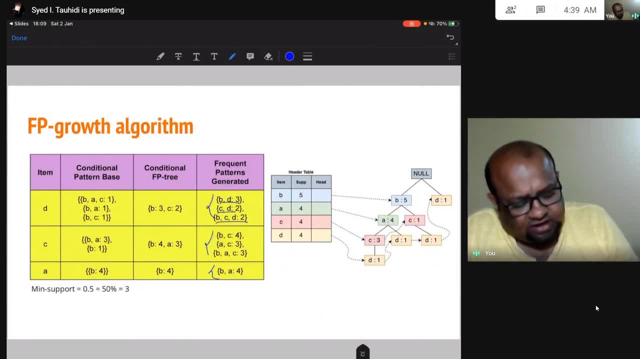 and these are the frequent patterns that we have generated. okay now, B A is often bought together. this has a support of 4,. okay, that means there are 4 transactions in which B A were bought together when buying A. okay now, when buying C, B A was bought together 3 times. B C was bought together 4 times. 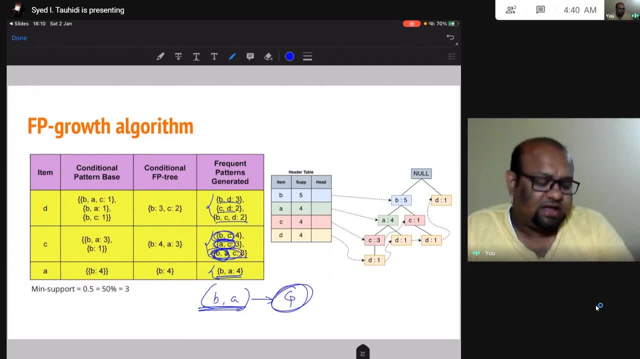 A C was bought together and B A C was bought together. 3 times right B A C. there are 4,, 3, how many 3 transactions in which B A C were purchased together? there were 4 transactions where B A, B C were purchased together, right? so in this way we get all these frequencies right. so lots of calculations we have to do. once you write the program you don't have to do all these calculations manually. 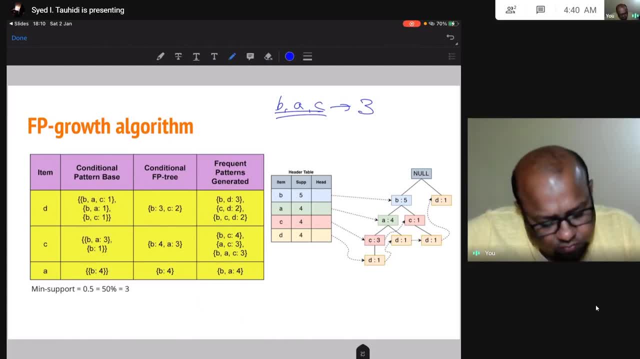 okay, now here there will be lot more. I forgot to generate with A. I made this mistake of not generating with A. I ended up ignoring A, should not have done that. okay, so that would generate lot more pairs over here, over here, okay. but no matter what, you have to follow the same rule. like we did in the other sets. you can generate for this set as well. okay. 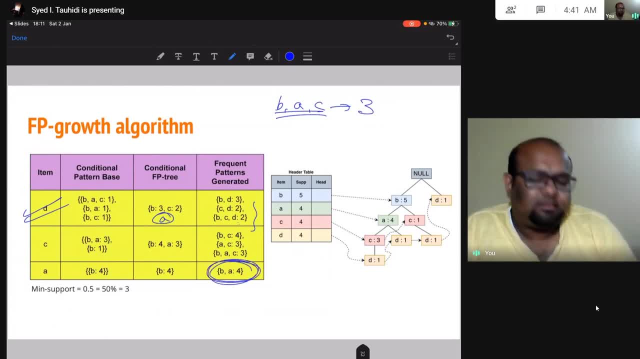 what does this mean? what does this mean? let us speak one of them and talk about this. this means that B and A are frequently bought together, these 2 items. therefore, I can generate a rule B implies A, or I can generate a rule A implies B. that means a person who comes to buy B go ahead and suggest A to that person. a person who buys A, go ahead and suggest B to that person. there are 2 rules that I can generate. now which of this rule am I going to choose? 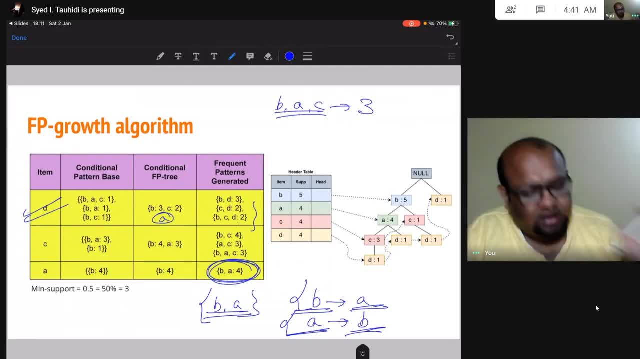 that is something that we are going to discuss at the end, in the same way we can. we generated frequent item set in April. we did not discuss how to create rules. in the same way, we are discussing how to generate frequent item set. we have generated all these frequent item sets, right, we are not discussing how to create rules yet. okay. 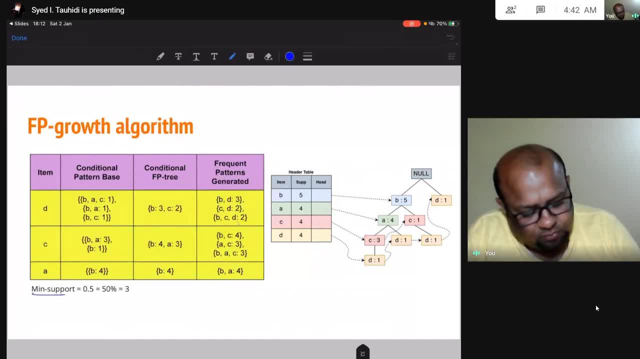 one thing: my mean support is equal to 3, so this, this will go away. okay, so what are the ultimate frequent sets that I have? I have BD, I have BC, I have AC and I have BA. okay, I have this, this, this and this. these are the 2 item frequent set. 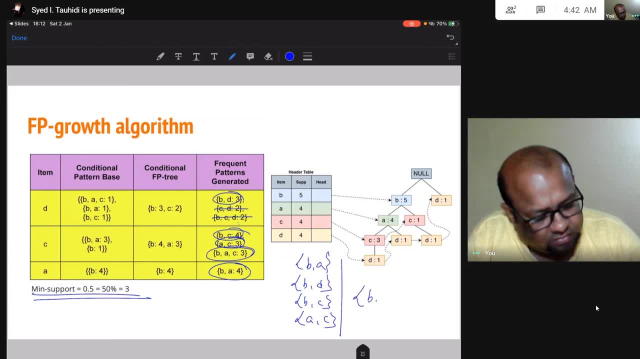 what are 3 item frequent set? I have generated BAC. okay, this is a 3 item frequent set. so I have generated frequent item set like this: from this, I have to generate rules. all right, we will talk about rules at the end. this is a priori. this is FP growth algorithm. all right, now think about this: how many times did we scan the data set? okay, we scanned the data set one time. 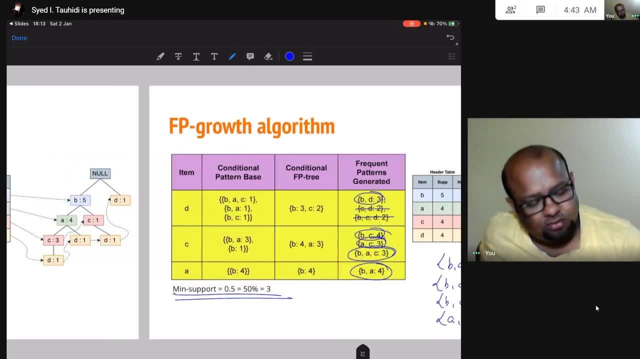 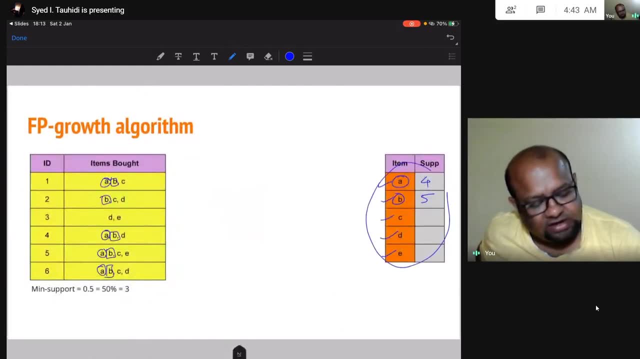 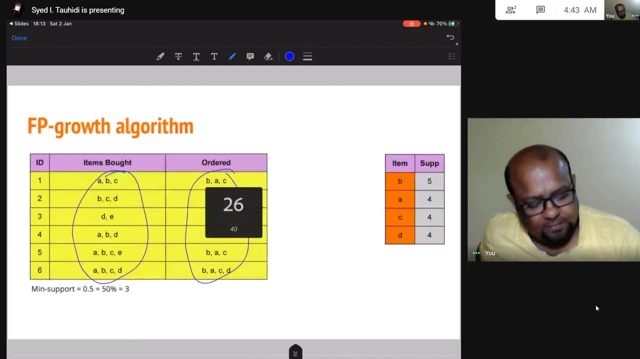 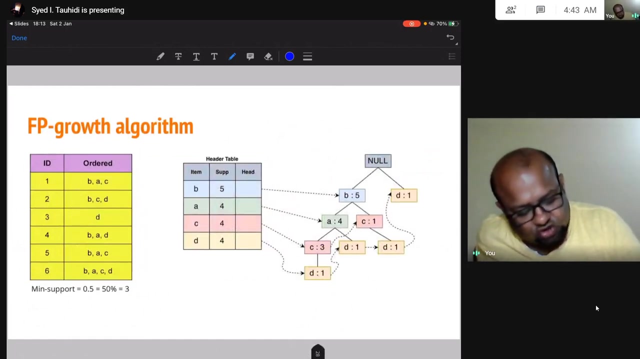 when we were creating this table of support. when creating this table, filling this table, we did a scan of this data set and then we scanned the data set once when sorting and creating the string. okay, this sorting that we did from ABC to BA. 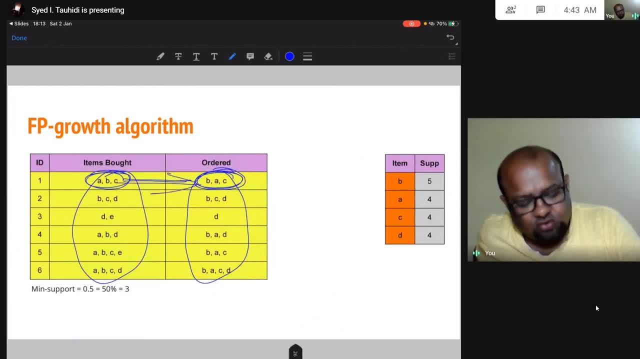 BSE. This is one sort. As soon as we did the sorting, we can insert it into a tree. Okay, It is not necessary that we do this sorting once and then we scan it again and then create the tree. As soon as we do the sort, we can insert the transaction into the tree. We sort this from this to this, and then we insert this into the tree. 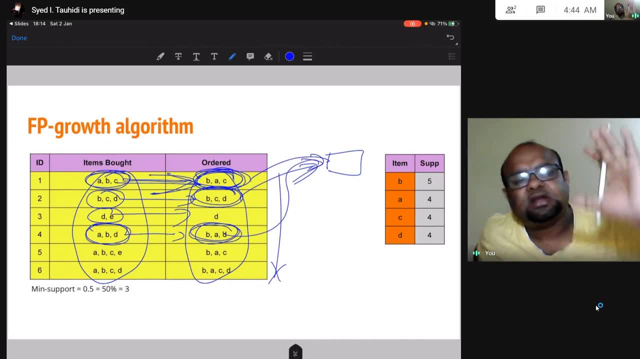 Okay, So in total, how many times we are scanning? Once at the beginning and once at the end? Two times With two scans. Compare this to April. In April we could generate an exponential number of items. For each of them we have to do a scan of the data set, Right, So an exponential number of times. This is far better. 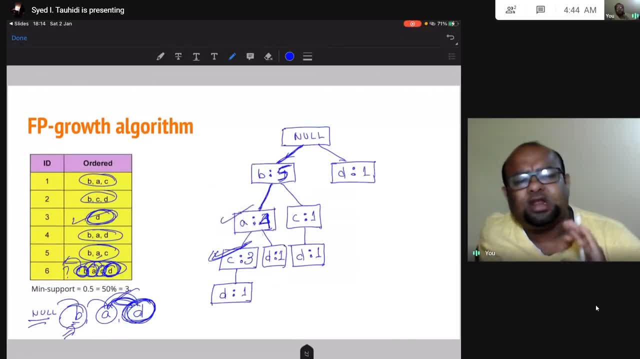 Okay, In April, don't worry too much. Okay, Theoretically we can scan for an exponential number of time, but April is actually good. It's not bad. We stopped much early and we do lots of pruning, Okay, So we. 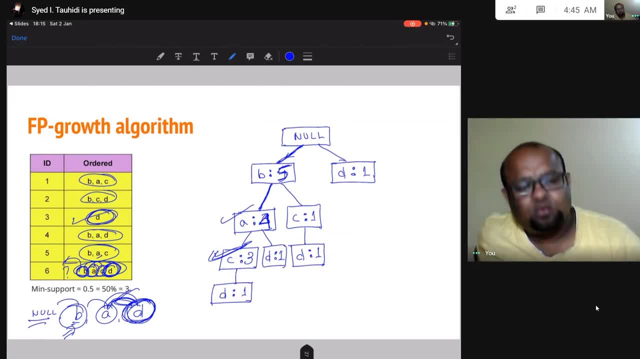 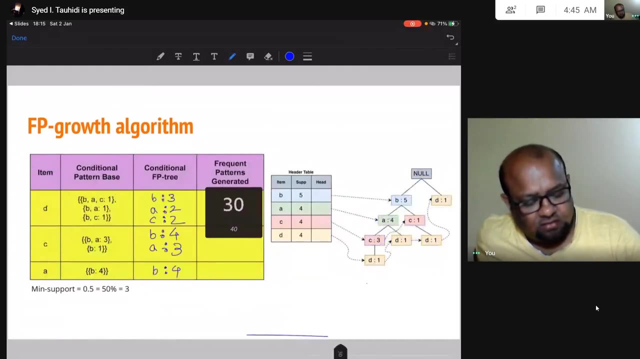 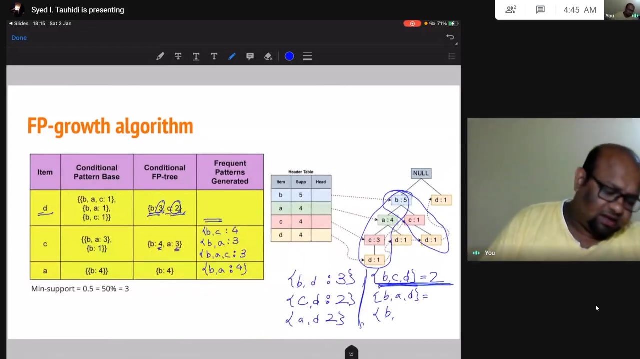 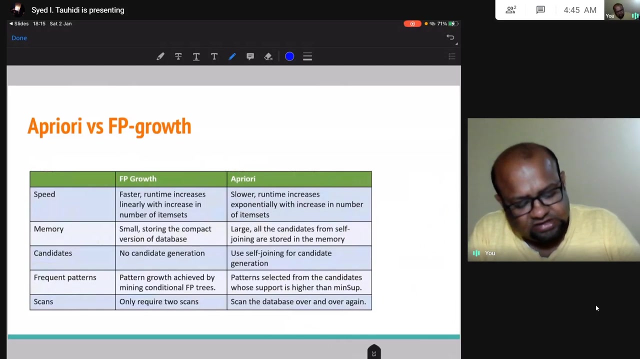 do not actually scan it for an actual number of times. We could potentially do that, but we do not usually do that. April is good. Don't hate April. Okay, See also the 这么 degree. there was nothing good or not OK, and. 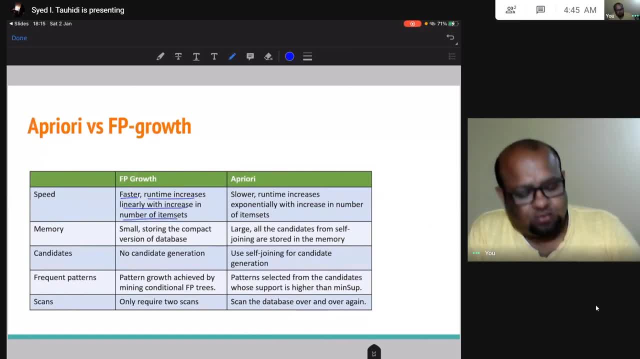 when we talk about at 1 pm, let's talk about 1 pm drop exponentially with number of items. okay, so if number of items increase, there is an exponential increase in time. okay, memory is, requirement is small because we just stored a tree here, all the candidates, the exponential number of candidates that could 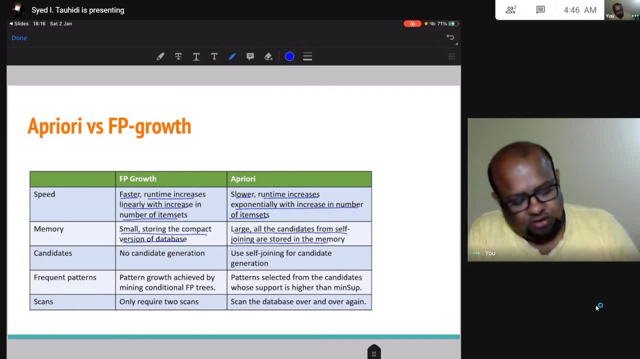 potentially be generated have to be stored. okay, candidate generation in epic road. there is no candidate generation here. we have candidate generation frequent pattern. we get this pattern by analyzing the tree, by mining the tree. here we generate candidate and then we see if the support is being achieved. all right, then scan. we only require two scan. i said at the beginning when 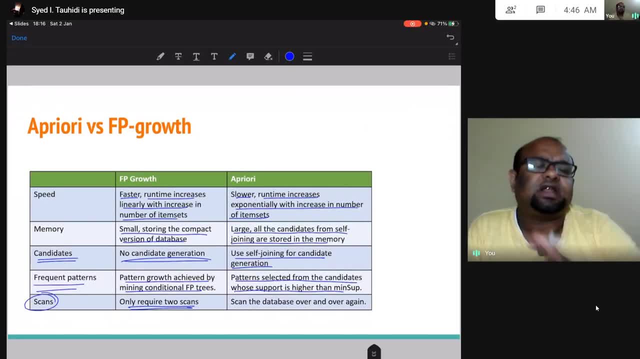 finding the support and at the end, when ordering and inserting into the tree. you now here we scan over and over again in april. all right, so these are some differences between april and epic road. epic road, in case our data is very big. epic road is the way to go, but in case, 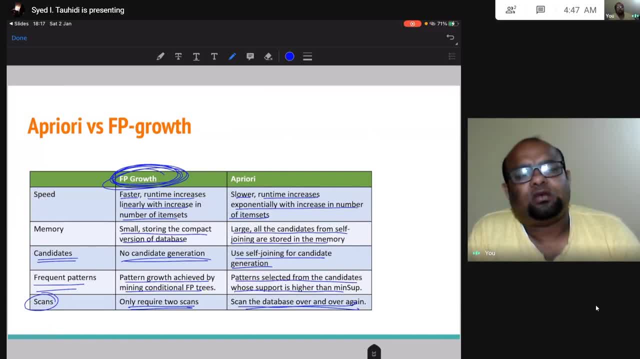 our data is small and handleable and we know the item set is not going to be large. all right. so three, four, item four is the maximum. say size of item set, all right. and number of items: item number of items is small. in that case, f you can go ahead and use a brydie. it is also good, not bad. 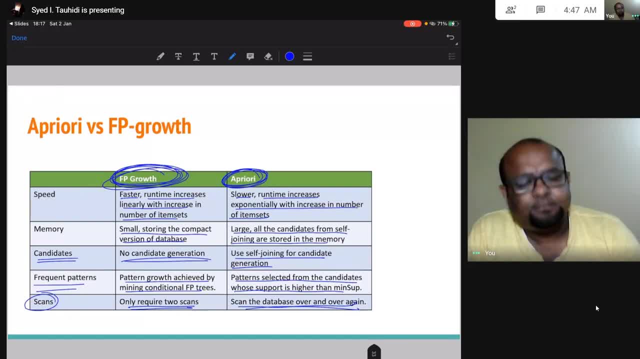 but epigroth works better, scales better, requires less memory, faster- lots of advantages. okay, now we are going to look at one more algorithm. all right, but don't worry too much about this algorithm. i just want to show you one more algorithm, why you do not go with this one. 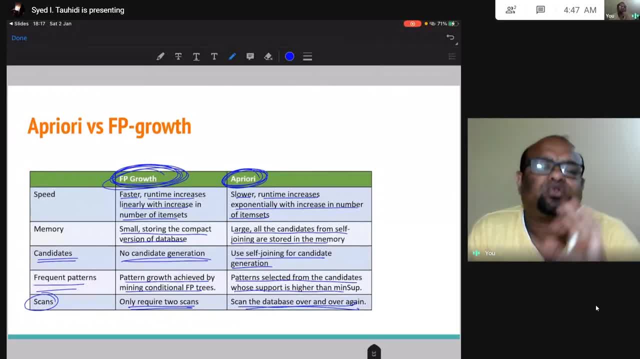 don't worry too much about this algorithm. i just want to show you one more algorithm why you do not go with this one, you this algorithm, because up to this point we were working in this way. i had a transaction here, transaction one, transaction two, and items here say item one. 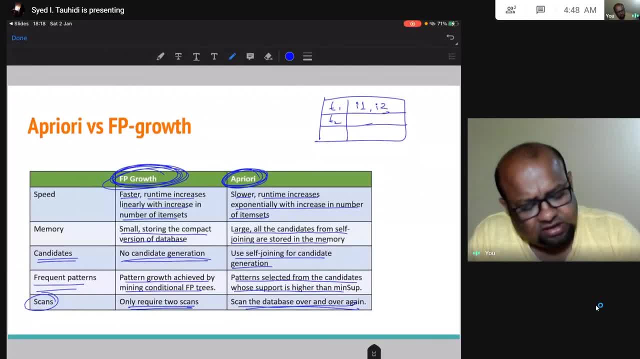 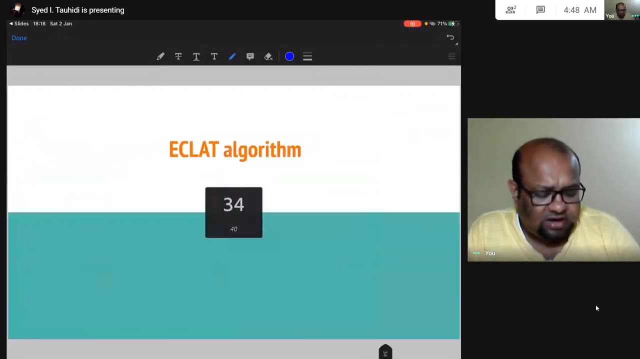 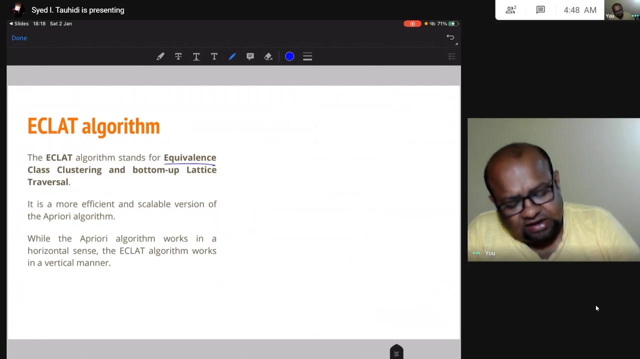 item two in this way. okay, so this is item three. item four: in the next algorithm we use a transpose kind of thing of this, not exactly a transpose, but you will understand. the algorithm is called a clutch algorithm: e, c, l, a, t, right, the performance equivalent plus clustering and bottom of lattice traversal. okay, it is a bit uh, efficient and 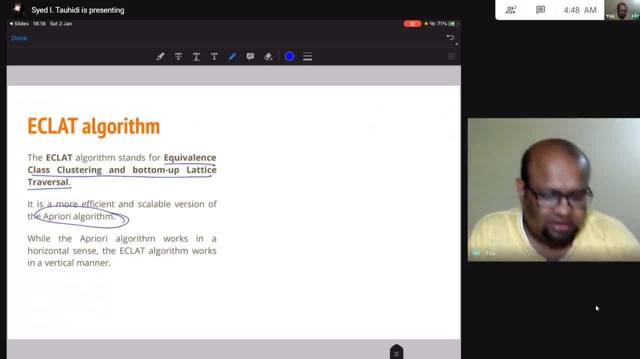 a priori not as efficient as fp3. this is also a uh generate and scan kind of algorithm. right, a priory is horizontal, horizontal, i mean: uh, there is transaction one, transaction two in this way, and then item one, item two in this say item three, item four, and item two say let me repeat item two two times. what is going to happen? 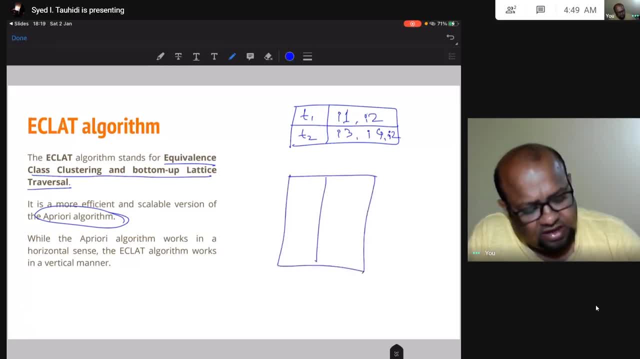 in: uh, eclat is. i will have items over here: items one, item two, item three and transaction will be over here. okay, so item one is there in transaction, uh one. item two is there in both transaction one and transaction two. okay, item three is there in only transaction one. item four is there in. 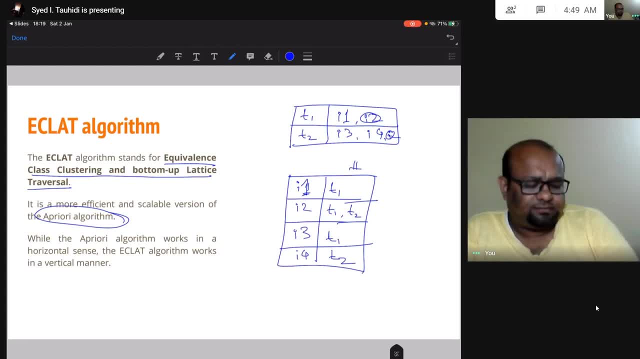 transaction two: all right, item three is there in transaction two, sorry, so this is uh vertical, this is horizontal. if this is horizontal, then you will call this vertical, because it's uh transpose kind of thing, not exactly a transpose in the linear algebra sense, but uh looks like a transpose. okay, this is our. 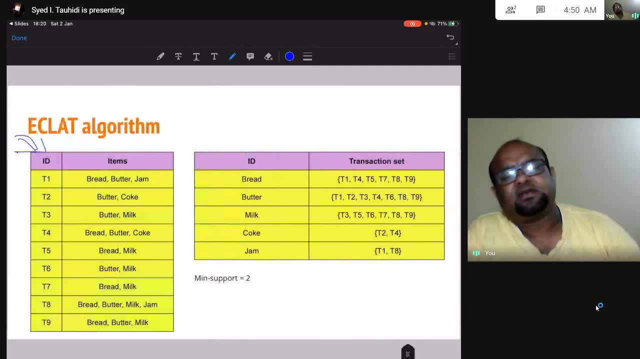 original data set as given to us. uh in uh. this a priory and fp tree. the transactions are over here. the items are over here. this is like before. okay, from this we transpose. this is not exactly a transpose. okay to this. let me call this pseudo transpose. 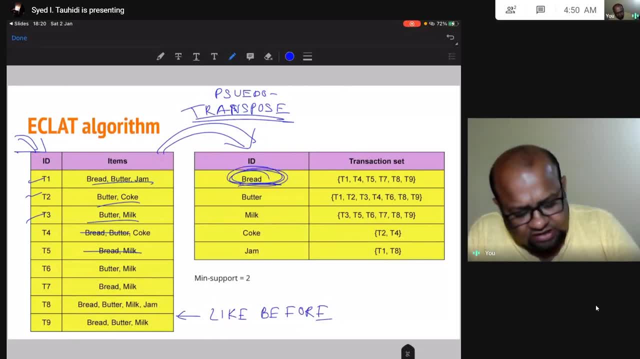 let me call this pseudo transpose to this. now, yeah, in how many transactions are there? well ready, suffering bad is in t1, okay, t4, t5, t8, t9, so we write that over here, okay, so cokey's occurring in transaction two and transaction through. 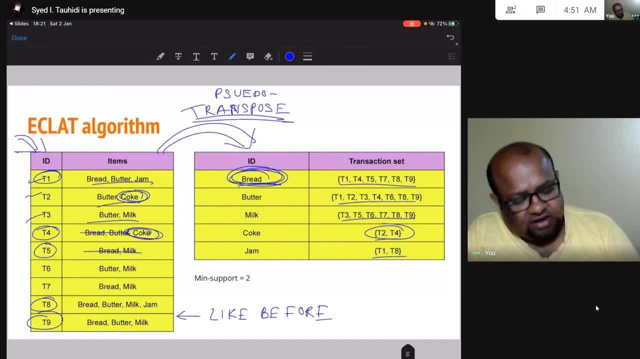 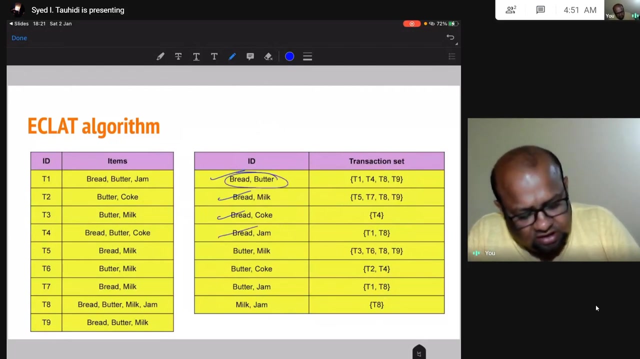 four: transpose our data set. then what we do, we have. we have done this for item set of size one. let us now work with item set of size two. okay, this is item sets of size two. now i find bread and butter. they are occurring in t1. 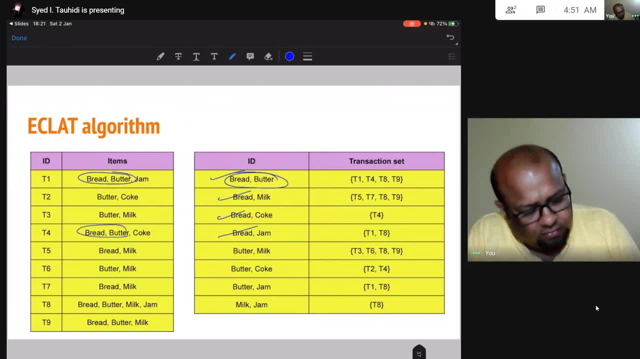 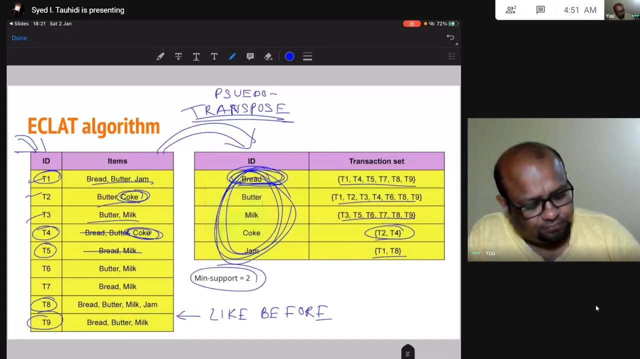 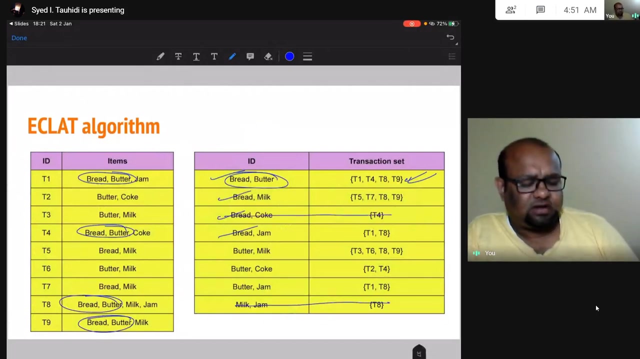 okay, t4, t8 and t9. okay, so that is what i have written here. so in this way i figure out item set of size two here my mean support i have taken as two. okay, so, uh, this will go away. this is less than mean support. this will go away. this is means less than mean support. and then i will. 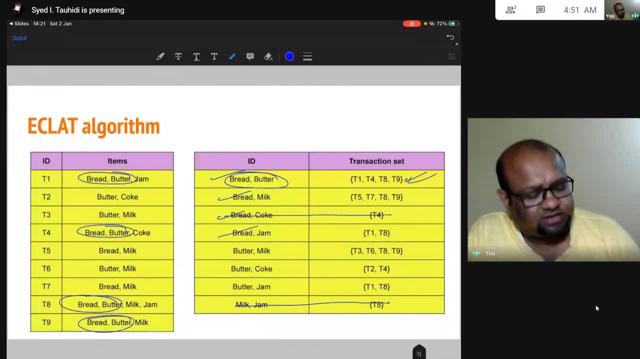 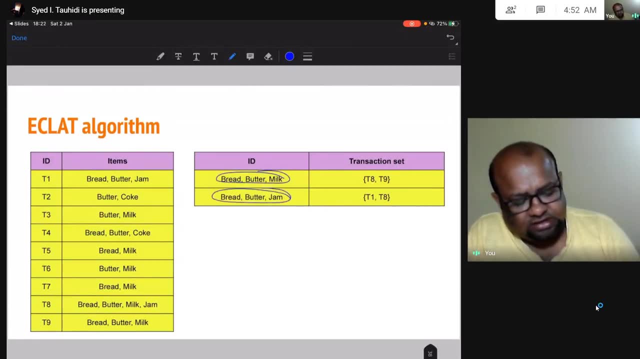 go ahead and make, uh, this item set of size three. three, so we make item set of size three and we have two potential item set of size three. okay, so this bread butter milk is occurring here, bread mutter milk is occurring here, then bread butter jam is occurring here, and bread butter jam. 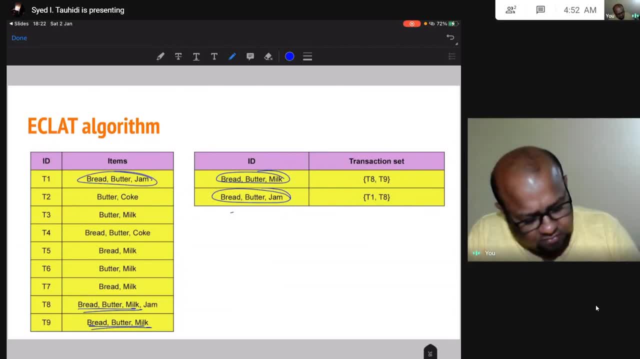 is occurring here: bread, butter, jam. okay, so in this way, i have uh reached here and then there will be jam- is one four item item set, but this has a support of only one. therefore, i am going to remove this and then i cannot make any five item item set. okay, this is not considered. 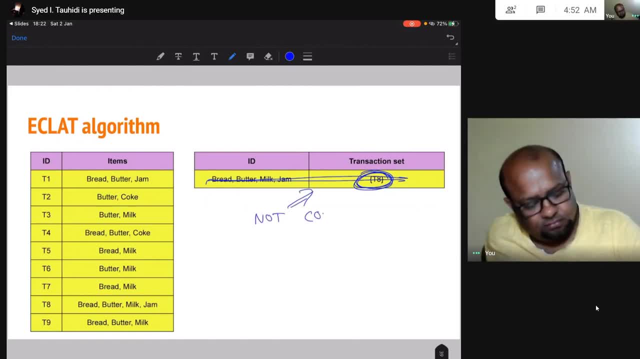 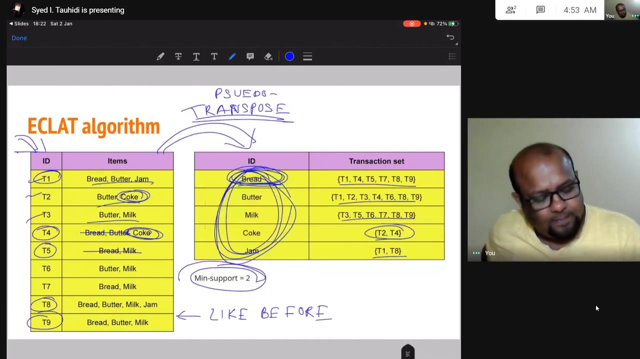 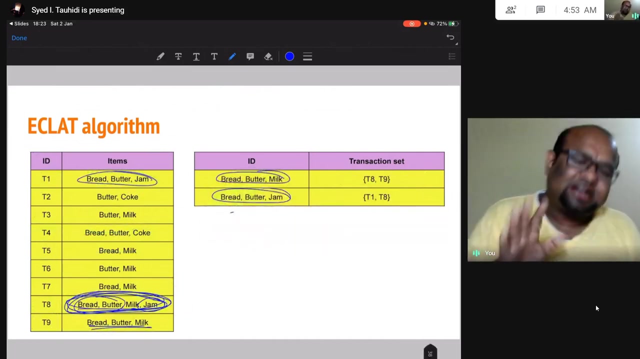 why is it not considered? because, uh, the threshold is not made right, the threshold we had fixed as two. okay, so this is what we do. this, uh, is one more algorithm. don't worry too much about this algorithm. that is the reason i am showing you this algorithm is because, uh, because of the 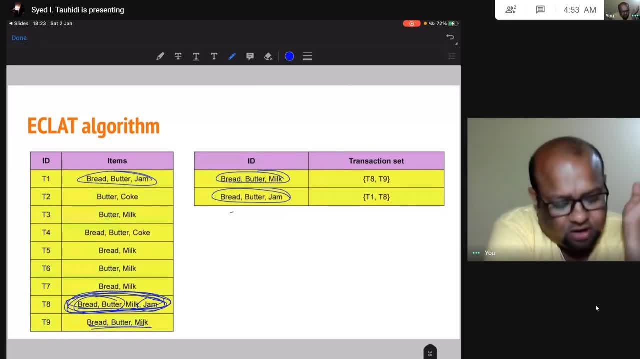 transpose of the threshold we have fixed as two. okay, so this is what we do. this is one more way in which this algorithm works, and i just wanted to show that there is also this technique. don't worry about this algorithm. study a priori properly and study fp growth. okay, you can do. 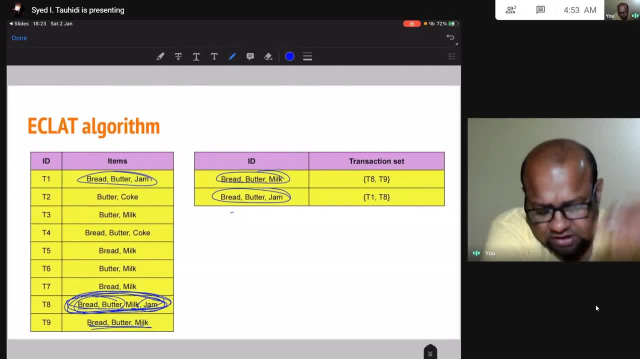 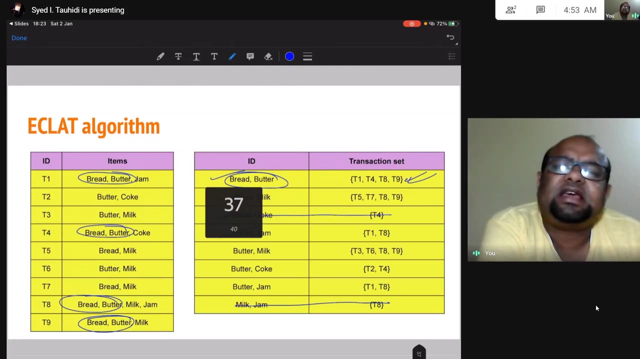 this as well. okay, once, if i give you a problem in a class, you can go ahead and solve that. of course, the reason i'm showing you this algorithm is because, uh, till now we have worked in horizontal manner right in both, in both- in both a priori and, uh, fp growth- we have worked in horizontal manner. here we are working in a 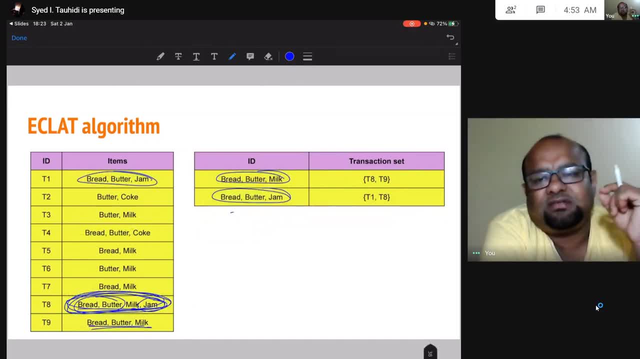 vertical manner. right, instead of counting means these items, we are counting transaction. so this is what we have. okay, okay, uh, we are going to conclude this video by talking about this topic that we are going to talk about now. the third thing is only if frequency set while we are doing gradation. 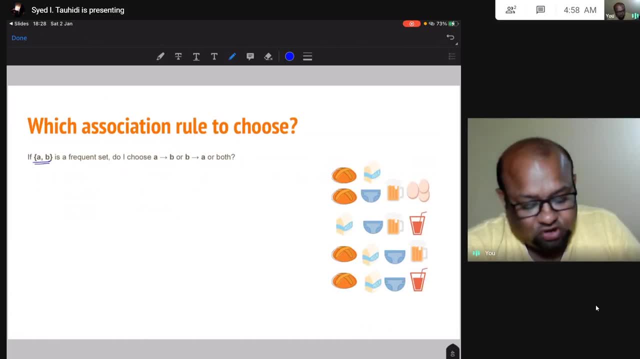 okay, this is what i just want to talk about. if you personally something already, you know, all I must well take a moment. or you might submit something. so in the previous we have, after two years, if there is a spring set of a certain frequency set. okay, that we did not talk about yet. 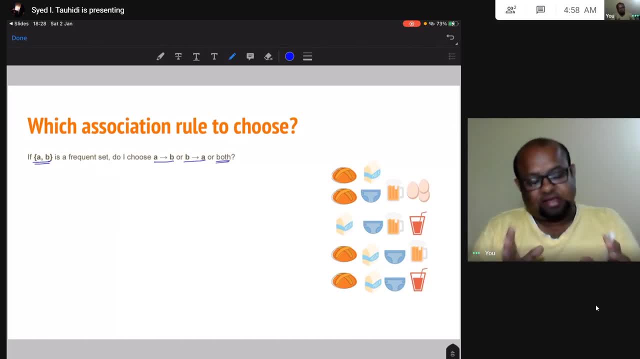 voi, choose: a implies b or b implies a or both. okay, given some frequency set, what is the association rule that is generated? so that was one question that we did not answer. till now, we have been talking about how to generate frequencies. all right, we had generated frequency set like this: plan the last group, for example, selection earlier morning. so the sequence set set time allows us to start with someosse cellular and all together then consider the correlation between the first other set of the composition we said, set a and b, each set of the association rules of the request set. so when we 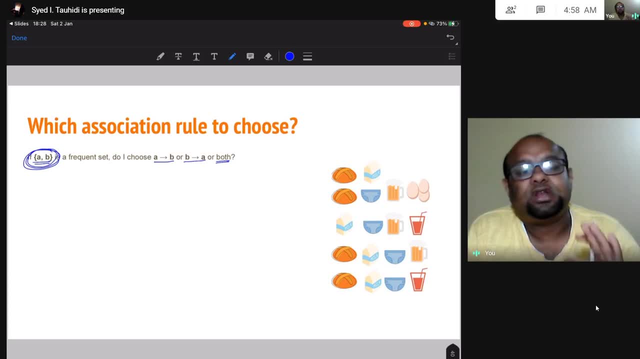 had generated frequency like this. but we did not yet talk about how to mine this rule. all right, so association rule mining is our ultimate aim, not generating frequency. let us talk about this. we need a criteria called minimum confidence. okay, so say we have set a minimum confidence of 70 percent. 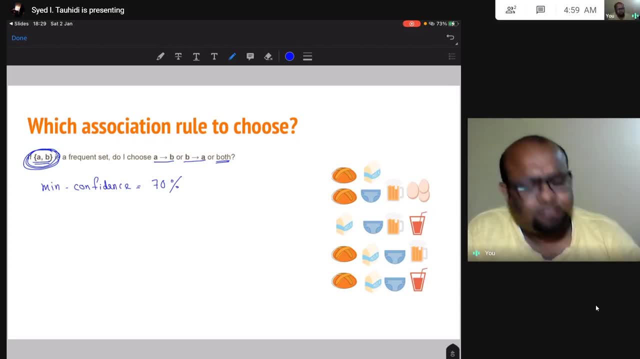 all right and say using some algorithm, uh, our support, say mean support plus two. okay, say using a pride, simple algorithm, we have found milk and juice. okay, so say we have set a minimum confidence of 70 percent to be a frequent pattern. alright, Now question is: do I choose milk juice as a association? 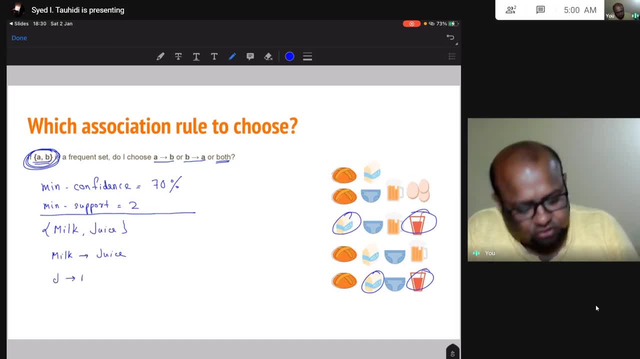 rule. Do I choose juice to milk as an association rule, Or do I choose both of them? I am going to find the confidence of both. Now, if you remember the formula for confidence, I have to find how many times is milk occurring. Milk is over here, here, here and here. So 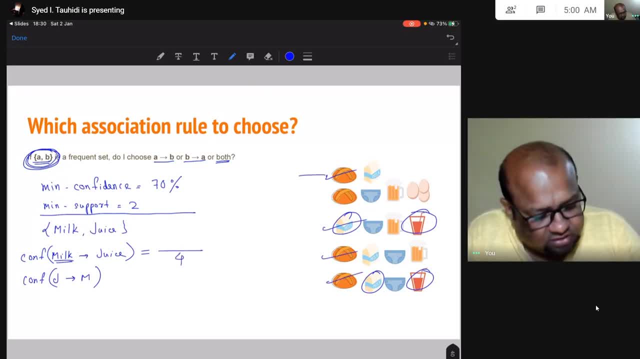 four times In these four times- alright, all the times that milk is occurring, in how many of them is juice occurring? Juice is occurring in two of them. So juice is occurring in two of them. So this is equal to 0.5,. okay, Confidence is 50%. What about this? If someone 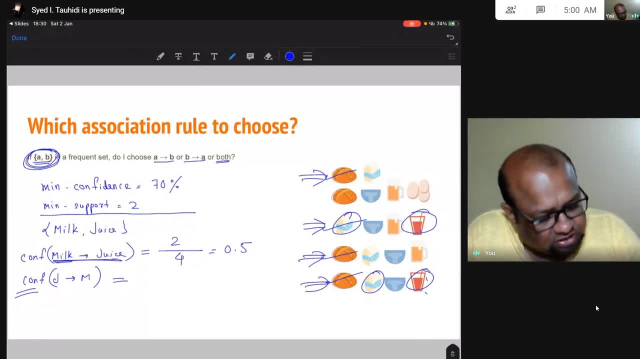 is buying juice. do I recommend milk? So this person is buying juice. okay, There are two transactions in which juice were bought, This and this. In all these transactions where juice was bought, in how many was milk also bought? In both of them, milk was also bought. Alright, Therefore, my confidence is 100%, Alright. 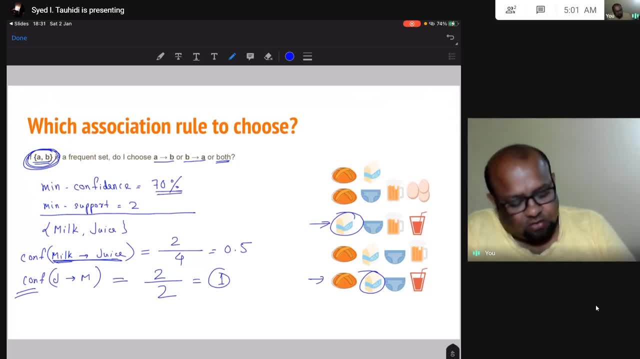 My minimum confidence is 70%. I am not going to choose this association rule. Milk implies juice, I am not going to choose. but juice implies milk, I am going to choose. Alright, That means, if a person is coming to buy juice, I am going to tell that person: do you want? 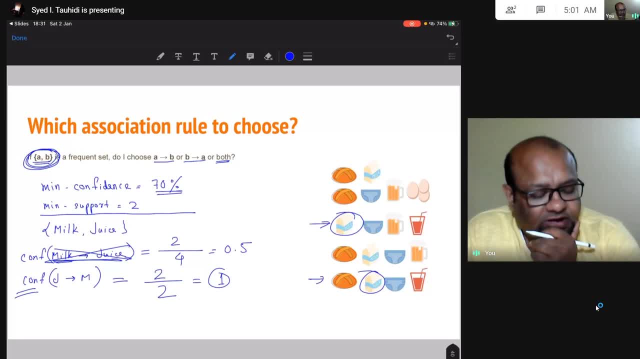 to buy milk. But if a person is coming to buy milk, I will not tell that person. do you want to buy milk? Do you want to buy milk? I will not tell that person. do you want to that person? do you want to buy juice? all right. so instead, what am i going to suggest to that person? 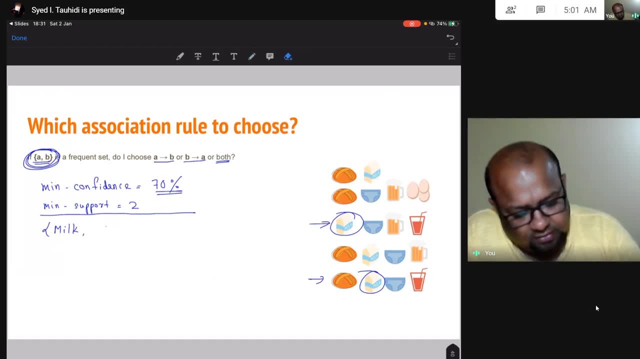 let us look at this: milk and bread, all right. so going to find confidence of milk implies bread, and going to find confidence of bread implies milk. all right, so this, this, this and this and this, all right, hold on, let me work on the first one first. all right, first one here. how many transactions are there when milk is bought here? 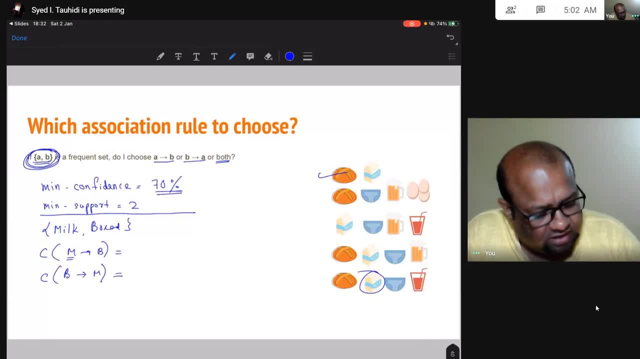 here, here and here. there are four transactions where milk is bought. out of those four, there will be three more in the first one. these four transactions- how many are there- where bread is also bought? so this, this and this. there are three transactions where bread is also bought, so three out of four. this is 0.75, so i'm 75 percent. 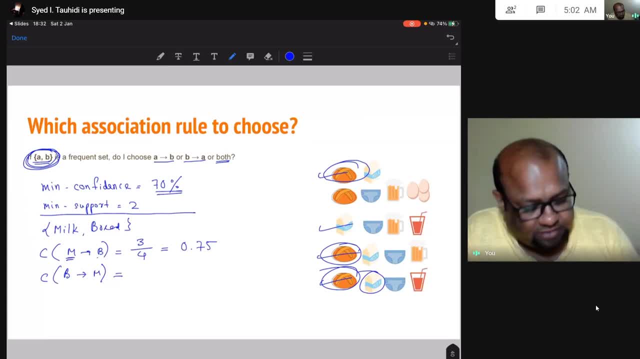 confident that milk implies bread. okay, so this passes my uh minimum confidence, so i'm going to choose this uh rule. okay, let us look at the other rule. bread implies milk. so this, this, this and this: there are four transactions where bread is bought. out of this four, there are three. 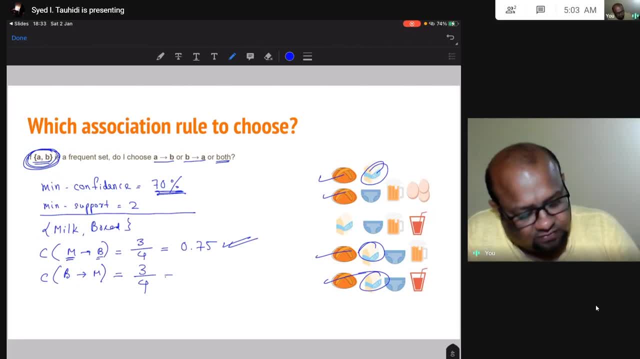 where milk is also bought. all right, once again, 0.75. so this is also something that i'm going to choose. all right, so think about what we were doing last time. last time i had this frequented milk and juice. all right from this if someone is coming to buy juice. 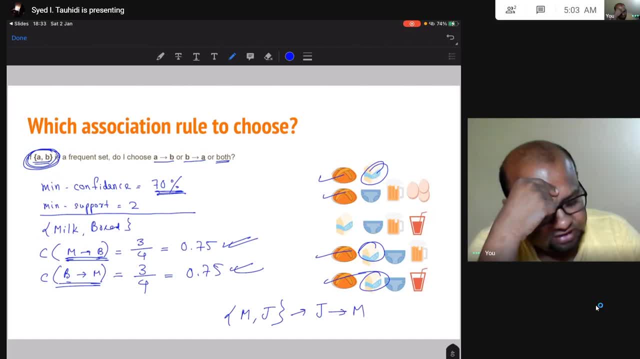 i am going to suggest milk to that person, all right, but if someone is coming to buy milk, i'm not going to suggest juice to that person. why? because my confidence in milk implies juice. this rule is not above the minimum confidence threshold that i had set. all right, but uh. 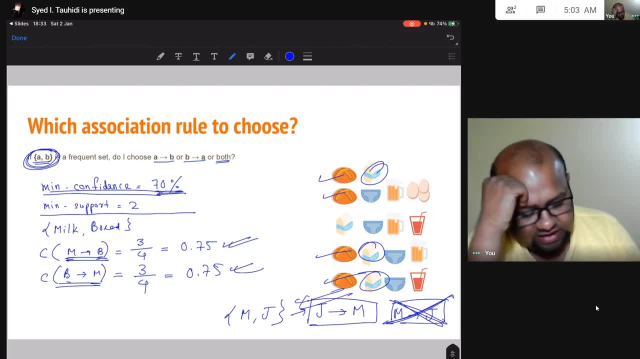 this passed the confidence threshold here, and if someone is coming to buy milk, i am going to suggest bread to that person. if someone is going to come to buy bread, i am going to suggest milk to this person. both of these are passing my minimum confidence threshold. okay, now, uh, if you have this, 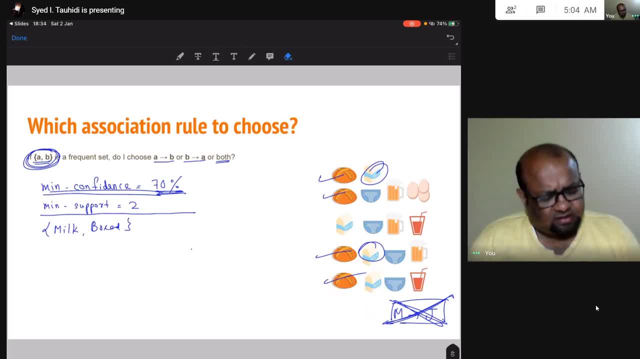 confusion. okay, let me not uh explain to you using examples. i'll just talk with you. okay, if you have this confusion? say someone is coming to buy milk and then there are two rules. okay, uh. rule number one says: uh, milk implies bread. rule number two says: milk implies diaper. okay, now, milk implies bread has a higher support and good confidence. 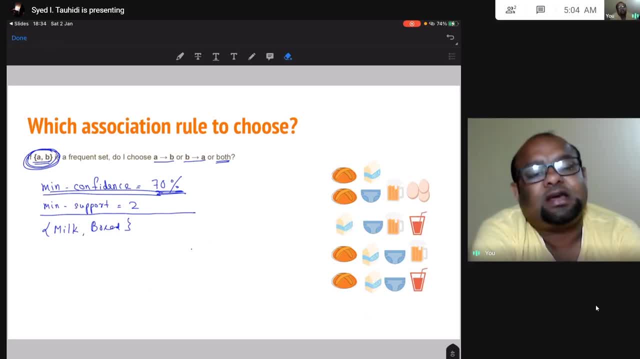 then i'm going to suggest that first. then i'm going to support uh such as diaper, so the one that has higher confidence, i'm going to use such as that first. but it should not be a single uh criteria. okay, i should also look at support, the. if my support is high uh, then i should focus on that as well. 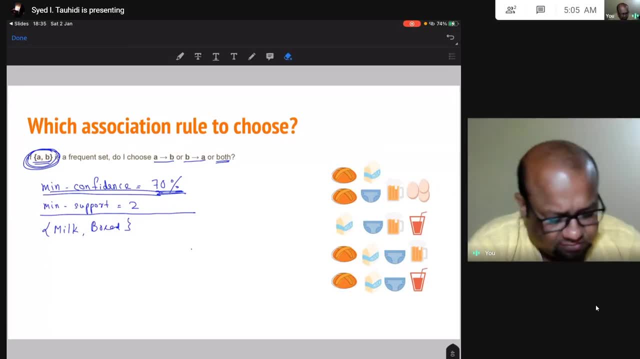 so how you do this is up to you. okay, right now i'm just giving you ideas on: uh, what are the things? okay, how to generate rules and how to do suggestion. okay. so, the more confidence there is, i'm going to choose that. but if something is bought only five times, okay, uh say, uh a person, uh bought milk and 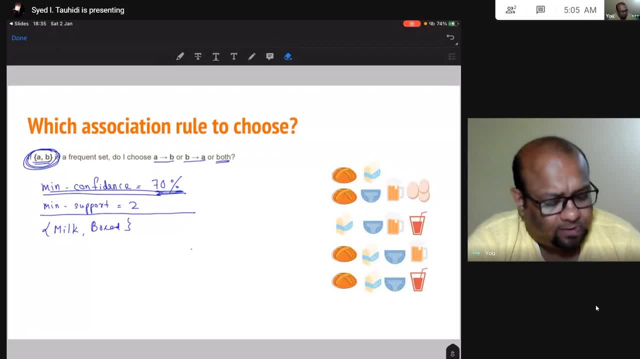 juice, okay together. so from juices perspective, i i am going to suggest milk okay, but uh, give you an example. uh, yeah, this is what. it is okay if something is bought a very large number of times together. i am still going to suggest that, even if something is bought very rarely together, 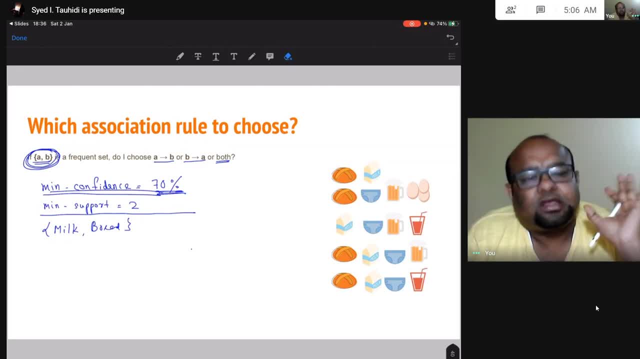 that has a higher confidence. okay. so yeah, that is what i meant, that, uh, not only confidence, i'm going to also look at support. if sometimes i'm not confident, i'm going to also look at support. if something is bought a large number of time together, then uh, going to suggest that okay. 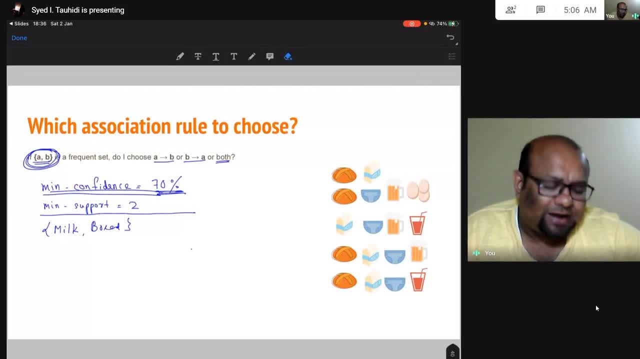 but, uh, here in our application, in our kind of transaction, that is not going to. this problem is not going to arise because we are looking at this from only one side. okay, so don't worry about all these things. this will be, uh, advanced topics that you can study on your own. we are not going to. 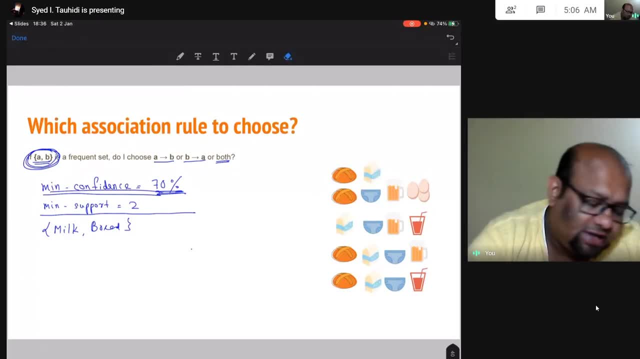 go into this now. so i'm going to say that if something is bought a large number of times together. now there is one more thing in recommendation engine system that we are not going to touch in this course, but i want to give you a general idea of how that works. okay, say in netflix. okay, 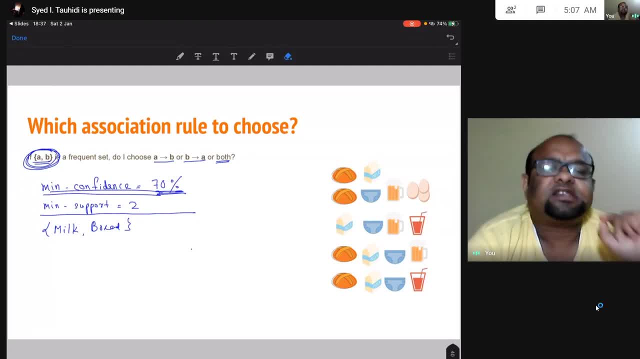 how to recommend a movie. i can find, say, harry potter and the chamber of secrets. i can find similar movies. right, i can find similarity using lots of similarity. measures are there. we saw how to use having distance to find difference between title. so harry potter and the chamber. 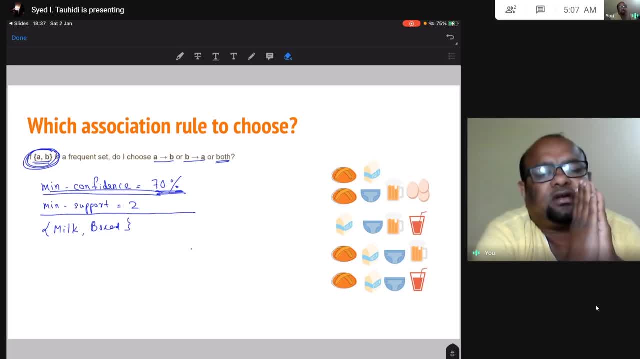 of secrets would be nearer to harry potter and the prisoner of askaban. then it would be to harry potter say then pirates of caribbean, okay, so i am going to suggest harry potter and the prisoner of askaban, okay. so this is uh direct content, uh similarity. how similar is my content to one another? 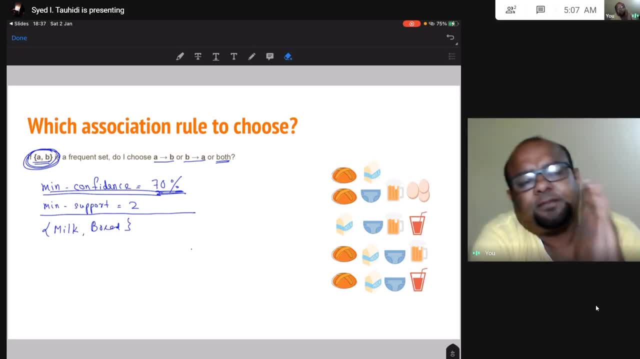 based on that, i can do recommendation. okay, but there is another technique of doing recommendation, a bit like what we have studied here. but, uh, not exactly what we are going to do is first: uh, i am going to see same. i want to suggest to, uh, mr x and mr y. there are two people i want to suggest to mr x. okay, i am going to find. 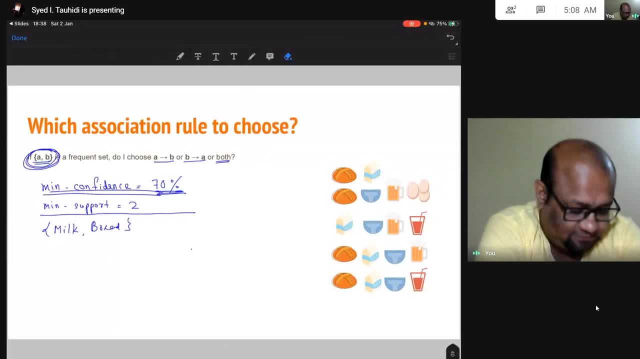 all the users that are similar to mr x. so, say, y is a user that is very similar to mr x, then what i am going to do is, uh, so similarity in things that mr x and uh mr x watches. so, out of all these things that mr x watches, i am going to find the similarity between mr x and mr y. 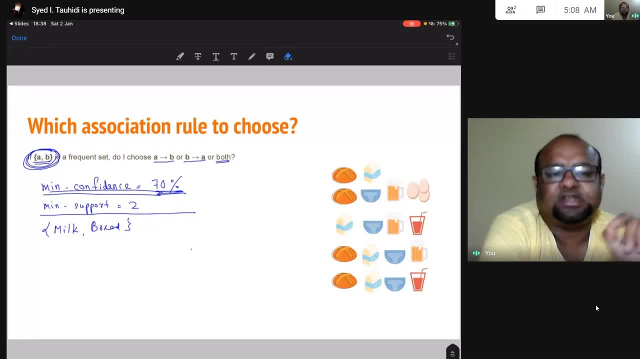 a similar user say: why is a user who watches things whose choices of things are similar to the choices of mr x, so why would be a similar kind of user? so i am going to see what. why is watching? okay, and based on that i am going to make recommendation to mr x. this is called. 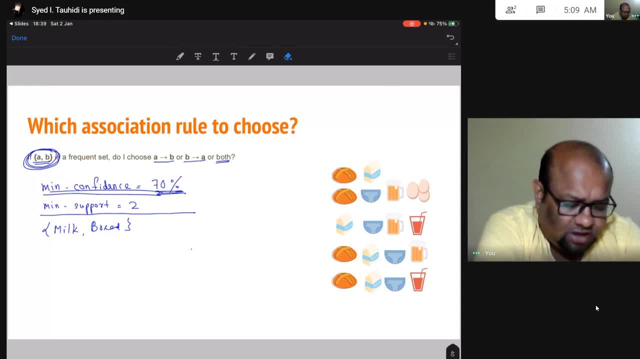 collaborative filter. okay, and nowadays this is the popular technique to do recommendation: first find users who are similar to you and then do recommendation. but, uh, this does not make sense in our uh application that we have seen in this video, because in this video, uh, i cannot rearrange. 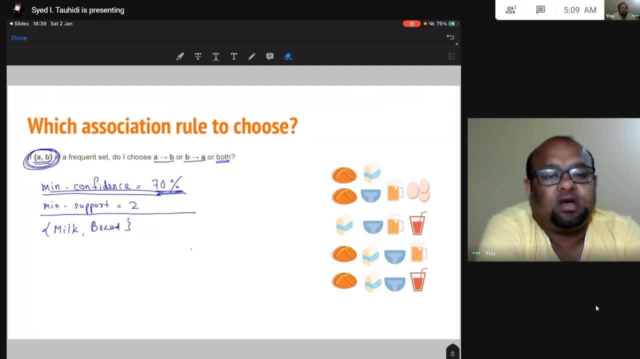 big bazaar for every user, right? so, uh, just because this user comes in and he likes electronic, so i completely keep electronic stuff near him. and then some other user who likes cosmetics, so i suddenly bring cosmetics to the front of the video. so i can arrange big bazaar for every user. so i can arrange. 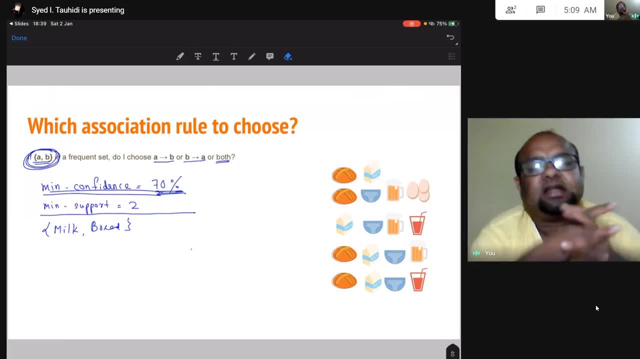 different road. that is not possible, so i have to do in general these are good techniques to do this stuff in general, all right. but yeah, understand that recommendation uh is more complicated. you can do user specific recommendation, all right, not only item specific. we have been doing item. 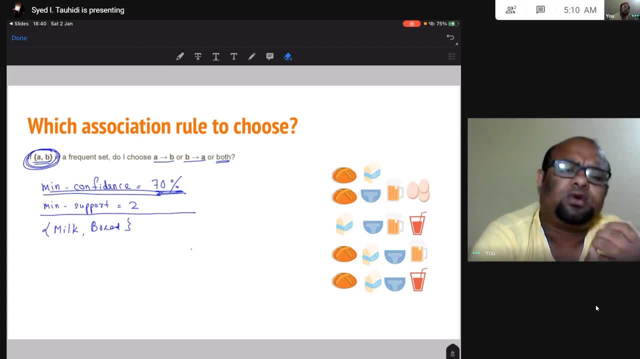 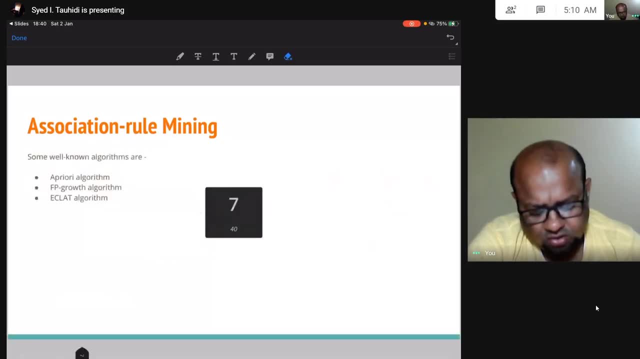 specific recommendation in this video. so to conclude, uh, we saw what is association rule. mining, we saw, is support. what is confidence? then we saw three algorithms to do association role mining, or two of them we saw in that and one we saw at a very high level, this eklat algorithm, at a very high. 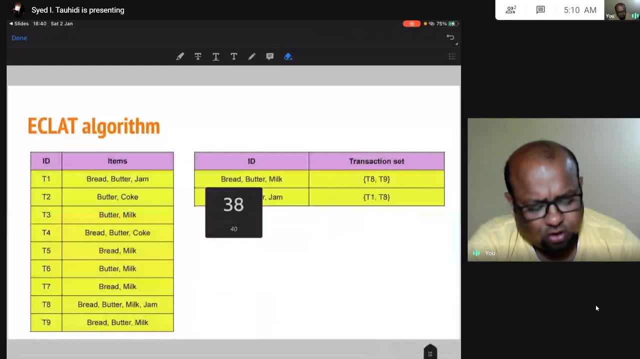 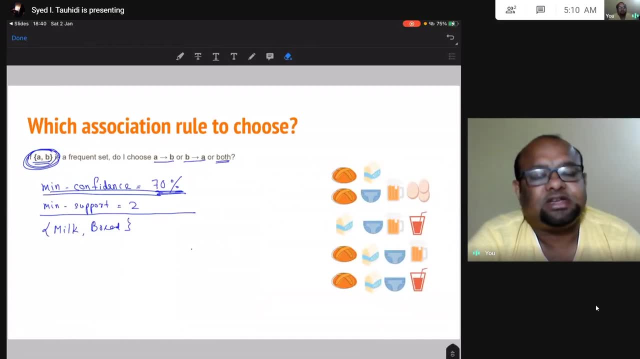 level. then this algorithm taught us how to create frequent patterns, frequently bought item set, items that are frequently bought together, how to find those kind of set of items. all right, and then we finally concluded by talking about: from this frequent set, how do i actually mine this rules? all right, so we have this association rule. how to get this association rule? one set can give. 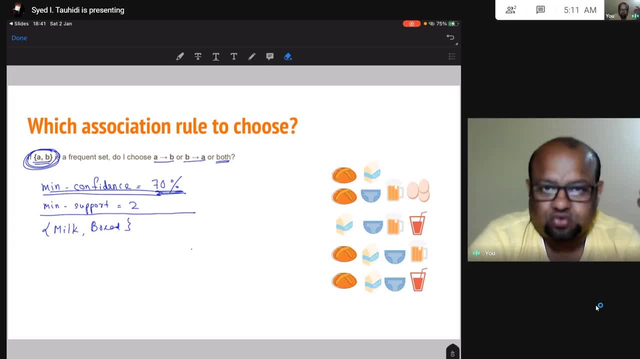 us multiple association rule. which one do i choose into my data set? right? so that's it. that was all the content for today's video. thank you for watching this video and if you have any doubt, feel free to reach out to me through whatsapp, through mail or by writing your. doubts in the comment section below. see you in the next video.